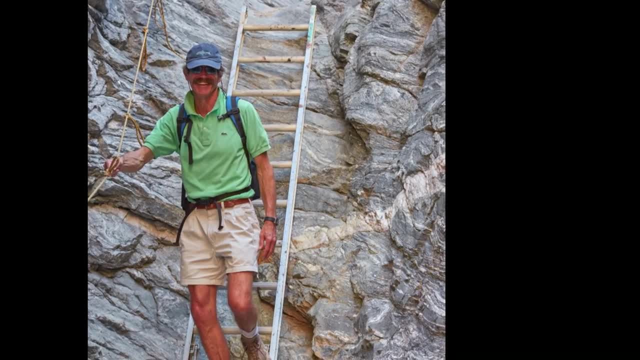 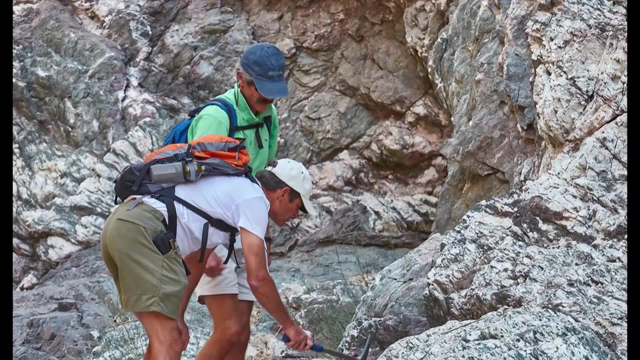 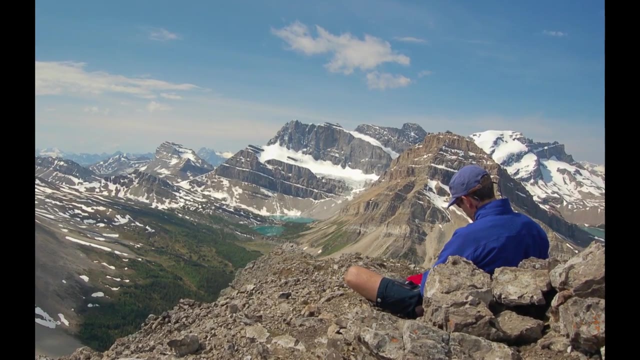 where his legacy includes the Gallagher Library and Gallagher Colloquium series. Tom has been involved in the research and development of the Gallagher Library, in resource exploration and development around the world. He is a member of several boards and foundations. Most recently, he has applied his knowledge of earth and ocean science to understand. 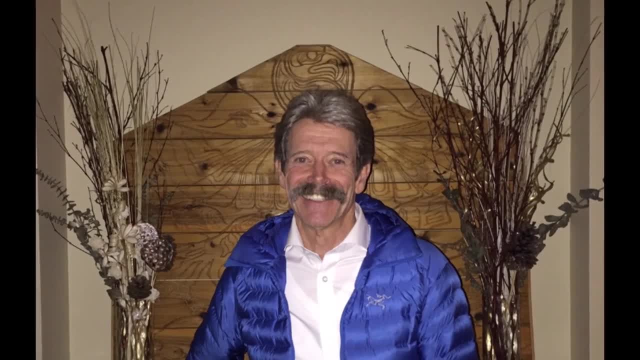 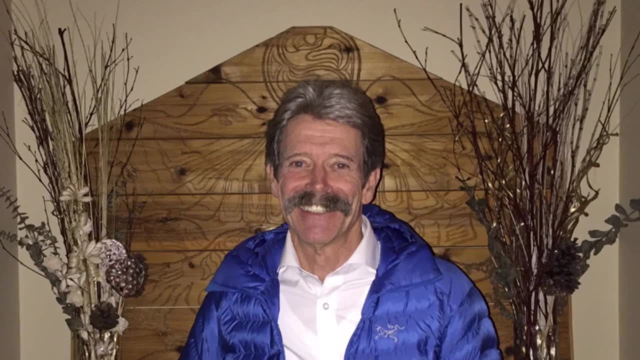 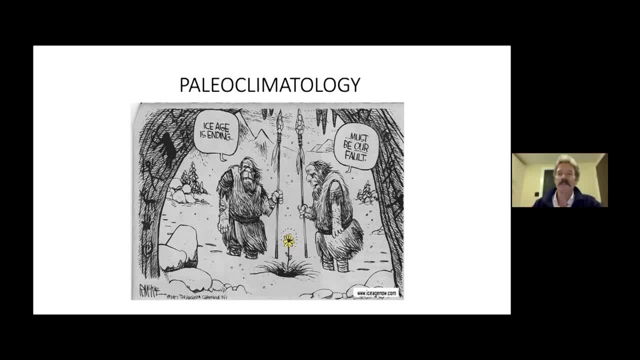 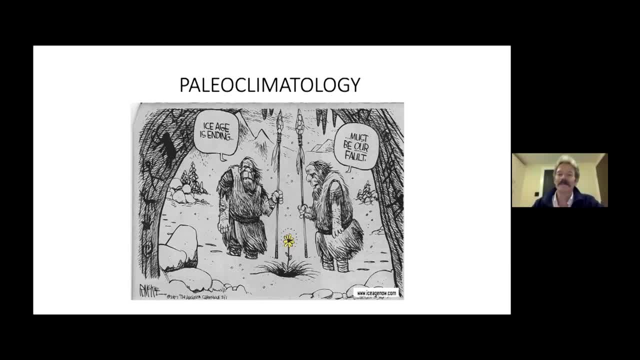 I'm not alone. I'm not alone- Huge word. We've been looking at ourselves in a little bit different way in the last little period of time than these fellows would have been. They would have been caught in the middle of the Cro-Magnon period. 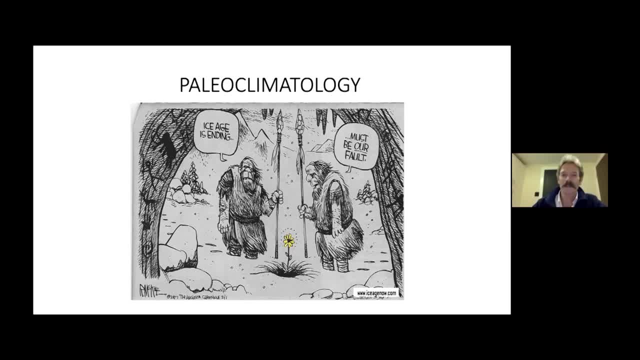 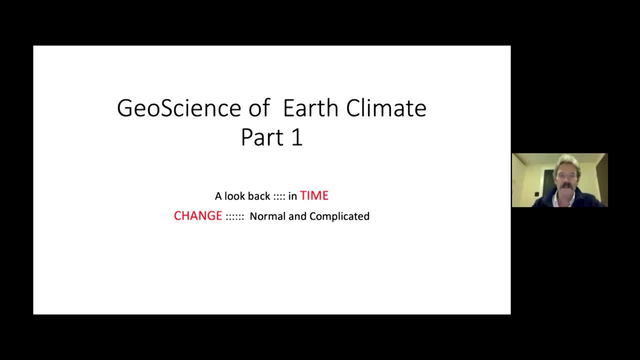 the ice age. When we survived, we got through, but barely by the skin of our teeth. So, as a geoscientist, as Roger has indicated, we'll be using my eyes- and hopefully I can train yours- to go through time and have a look at the earth's. 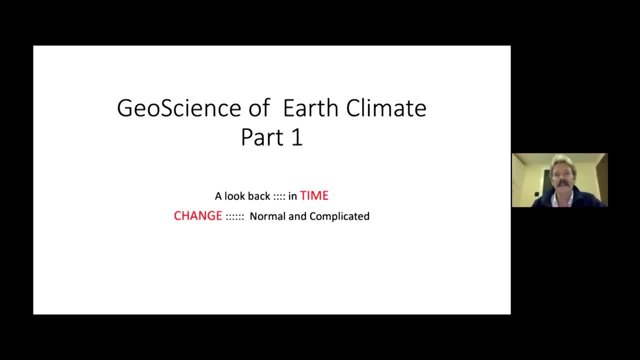 climate. We'll call this part one, because there's a second portion of it which will relate to our more current period of time. We are going to look back quite a way, and the thing that will be dominant- and you'll hopefully notice it very right away- is that change is everywhere and it's normal. 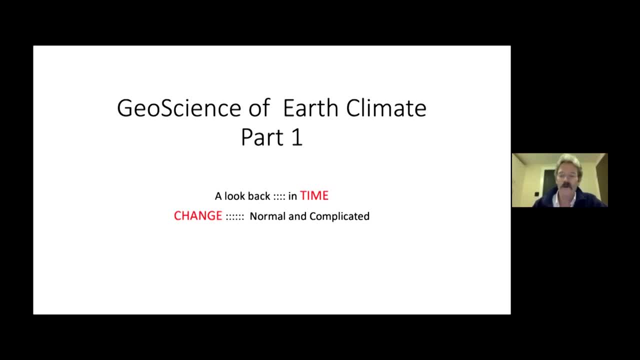 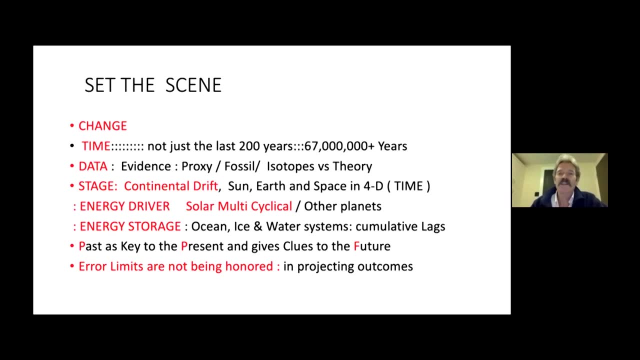 although it is complicated and so therefore has to be looked at fairly carefully, and we need to do that. We're going to be flashing back 67 million years, not just the 200 years that you often see many speakers talk about. now We have to look at the driving mechanisms, and we're going to do that. 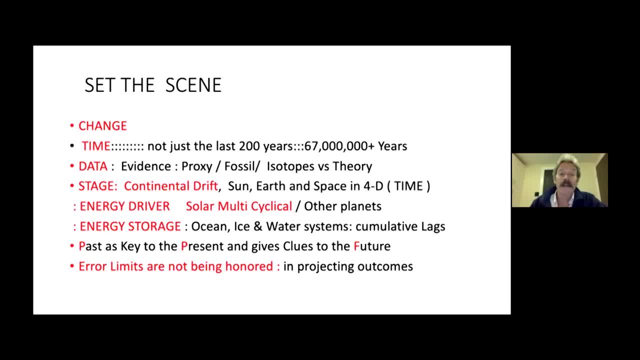 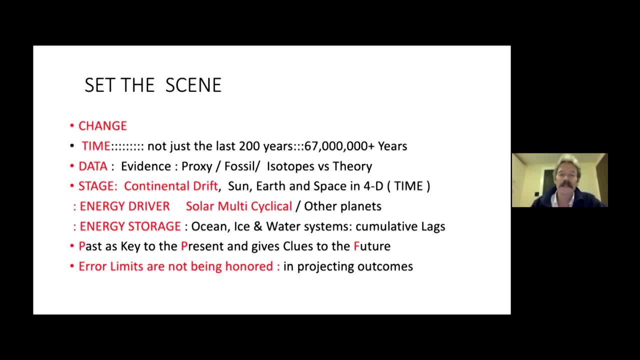 proxy, because we have to look at things that are fossil evidence in the rocks- and this is where our geologic evidence will be coming from, and we'll be looking at isotopes. These would be the components of oxygen and, in this particular case, carbon as well. We will be contrasting that. 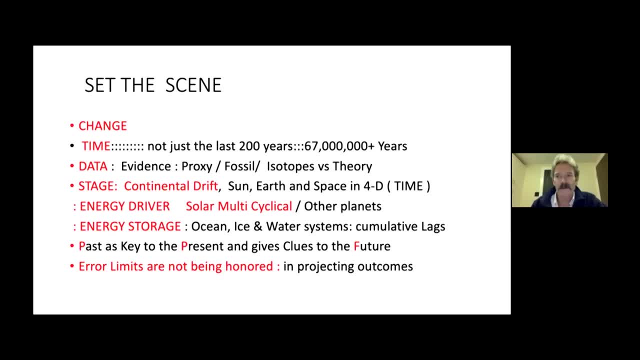 with theory, So I would rather be on the side of data and interpreting some data, not espousing theories, and so I won't do that. today, The stage, a place that we'll be working from, will be changing. It's going to be shifting around continentally, drifting around The sun. 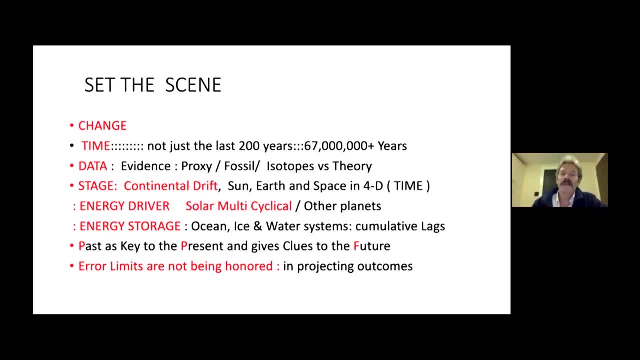 the earth space. we'll put that all into a 4D time framework and we'll slide the earth's components around to show you why we're getting such big change. Change is something that the earth is going through even as we're speaking. The energy driver. 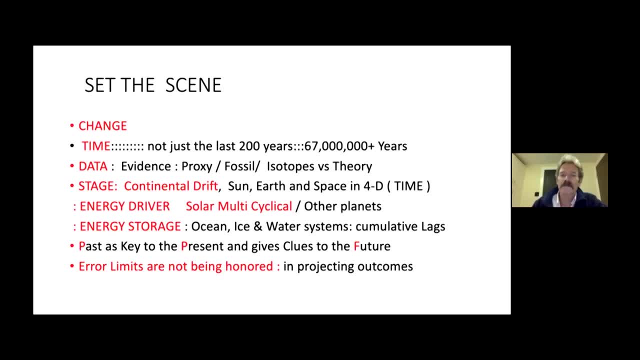 in this will be the solar cycle, the multi-solar cycle which we will explain a little bit later on, which has been with us like a heartbeat from the beginning and will show through the entire data set. We have other planets playing into that. sometimes We won't be able to get into a lot of. 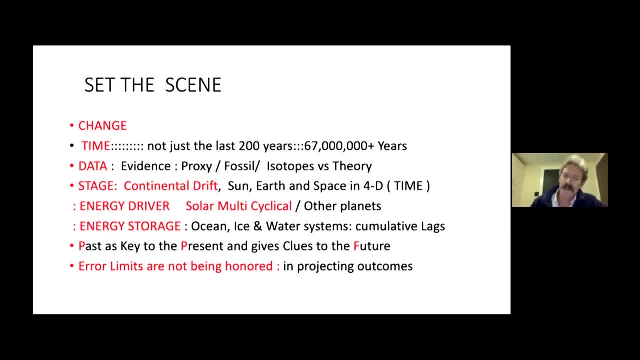 detail there, The energy storage in our system. as the only energy is really coming from the sun, we have to store that energy. We're going to keep it in the ocean, in ice, in water. The water systems, essentially, will show us why we get. 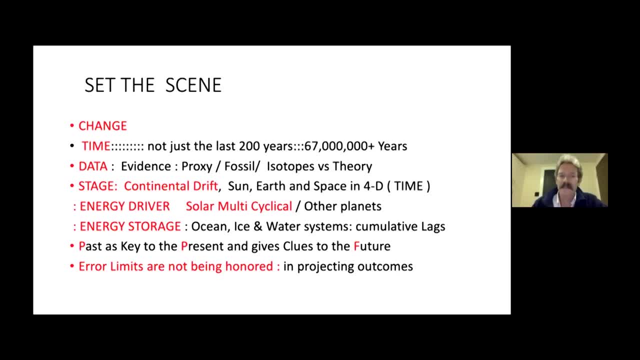 cumulative lags in the system, the energy system which drives climate. We are looking at the past as the key to the present, which shall give us clues about the future. Let's hope The error limits that we will try to honor all the way through this are not being honored. in much of the research that you will see, and many of the talks or the- I guess probably more- articles on climate do not honor any sorts of error limits that really exist. 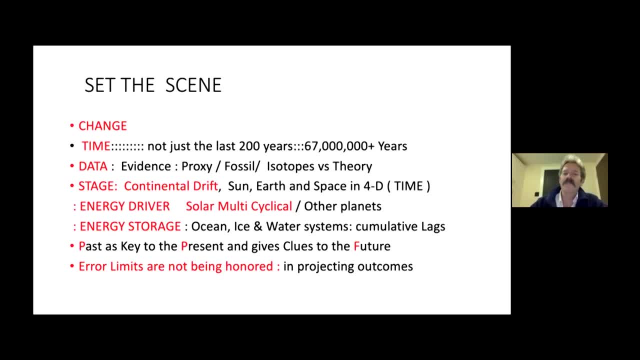 Notably, a lot of things based on the climate are not being honored. We're not going to be able to do that. We're not going to be able to do that. We're going to be able to do that. There's a lot of things that are based on what we would call modeling do not always honor their limits, and we will have to look at that eventually in part two. 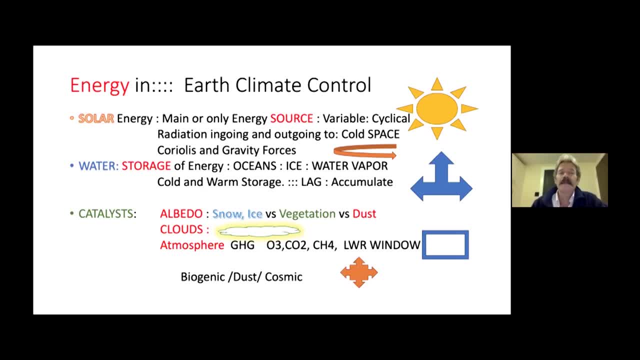 The energy itself for climate control is solar. as I had mentioned, It is the main or only energy source that we can look to of any significance in this particular request And of course, we're looking at it coming to us through radiation. We have to look at the incoming radiation from the sun And then we will look at the outgoing radiation. All of this radiation is coming to us through the cold vacuum of space. It'll be the place that our energy goes to as well. 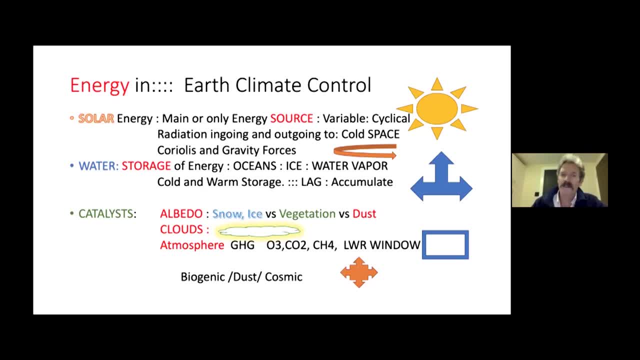 We have some minor forces, Coriolis forces, which drive the circular forces on the Earth of currents, wind, of course- Notably we noticed that- but also under the ocean. Gravitational forces will be a minor component of that. We'll just try to touch on that briefly. Water, as I mentioned, is our storage mechanism. 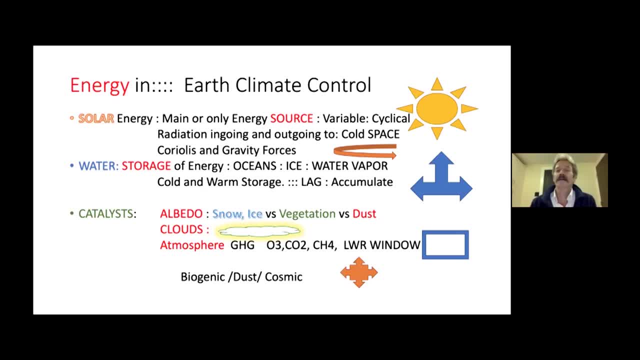 The only one that works really here on Earth. We have a unique system, We have a unique temperature regime And we are in an area of abundance. Ocean water is very abundant, of course, And we can tap into that with many means. 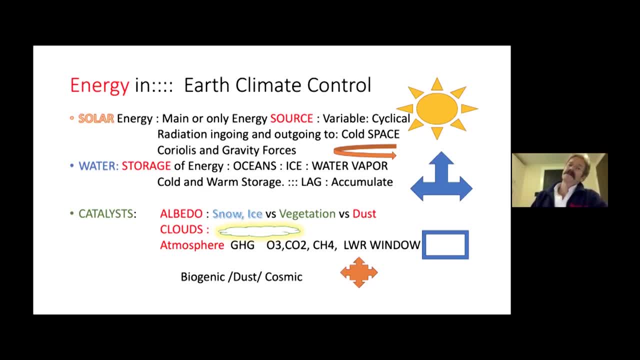 So we're looking at the oceans, the ice and the water vapor as our storage mechanisms. We're dealing with hot and cold, or warm and cold and lags, and accumulation of energy that will drive the system. We're dealing with hot and cold, or warm and cold and lags, and accumulation of energy that will drive the system. 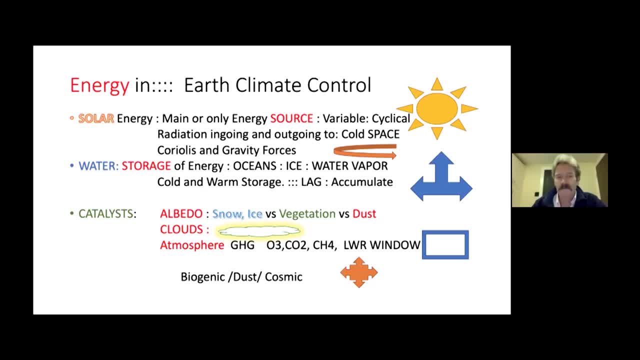 We're dealing with hot and cold or warm and cold and lags and accumulation of energy. that will drive the system. The sun will always be there, but will vary to a degree. We'll look at that as well. Catalysts for this are albedo- Now, that's the reflectivity off of snow ice. 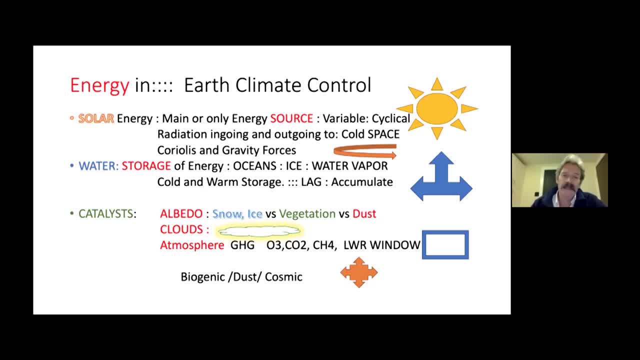 What we have is also clouds. Vegetation, as I would say, under albedo, would be something that takes energy in and retains it and preserves it. The snow and the ice reflect it. The clouds reflect it. for the most part, The atmosphere will be the last component of what we'll look at and it will be more dealt with in part two. 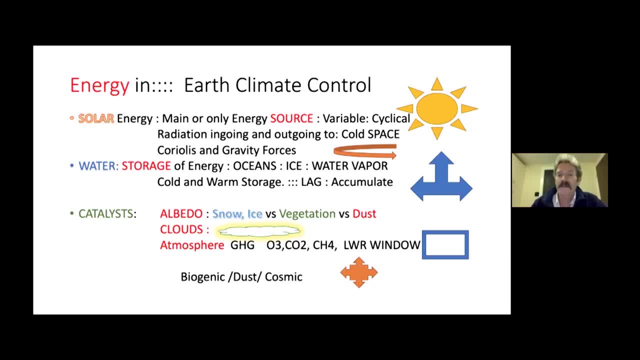 But that is a situation which always is present in our minds, but isn't the major driving mechanism that we need to go back in time with. So we'll have biogenic dust and cosmic Rays or particles as a component of what we talk about in future. part two: 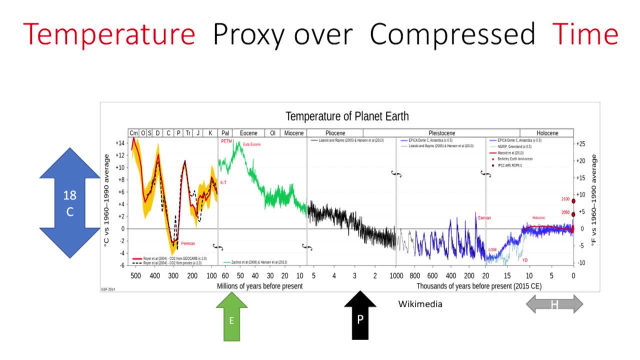 Temperature as shown on this graph, or a proxy of temperature. we'll deal with later what that means is shown here over very compressed time. So what we're dealing with here is 500 million years on this side and present day over on this side. 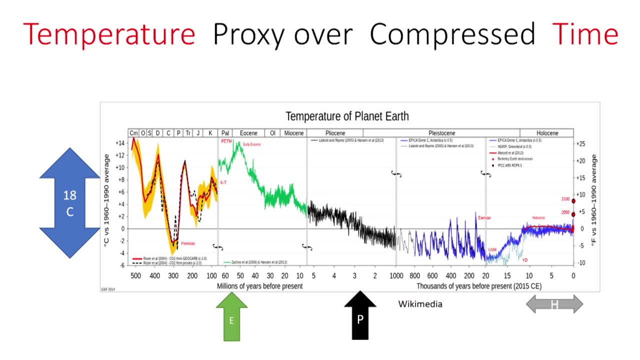 Here. these arrows will be more meaningful later on, but we'll be picking up our historical look at Earth's temperature and the Earth climate from the Eocene- this E green in this particular case. We'll be following it through to this portion here. 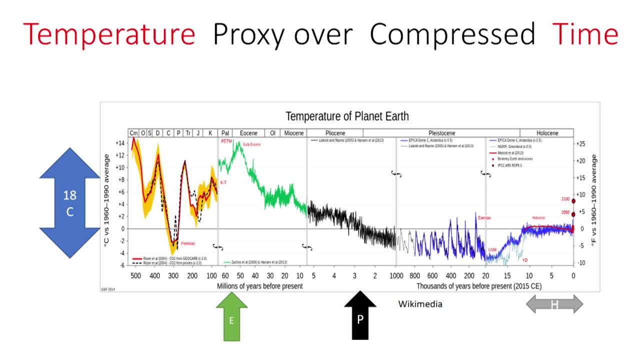 As you can see in this graph, there are big breaks in time here and we will fill all of that in and we'll deal with the entire period We are living in this little island of time here, The Holocene, So we'll come back to that as well. 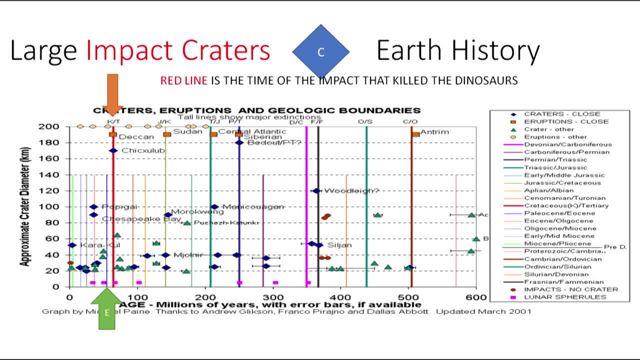 This is where the impact craters that created the death of the dinosaurs are shown. This particular one, Chicxulub, is the one at the red line here which killed the dinosaurs. We'll be moving from this point to the left. 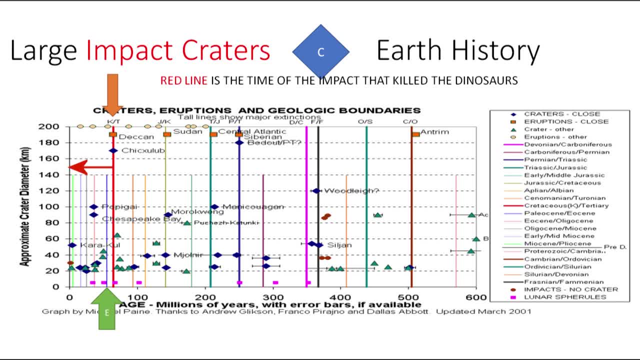 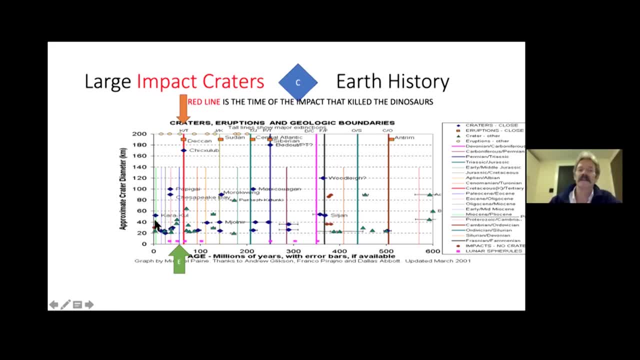 We'll be going into the zero point here And we will not be concerning ourselves. We will be dealing with former time periods which all, of course, can be studied, but in much less detail than what we can do in the current period, and with a very different arrangement of all of our continental sheets and the Earth itself. 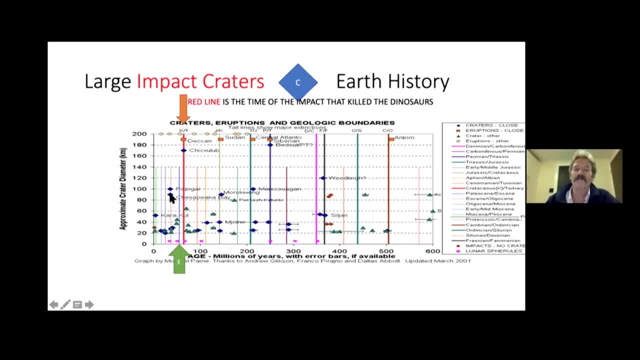 So we'll be dealing with a fairly consistent series of things in this other period. We do have some other impact craters which we will be trying to allude to or look for the evidence of in what we see a little later on. So 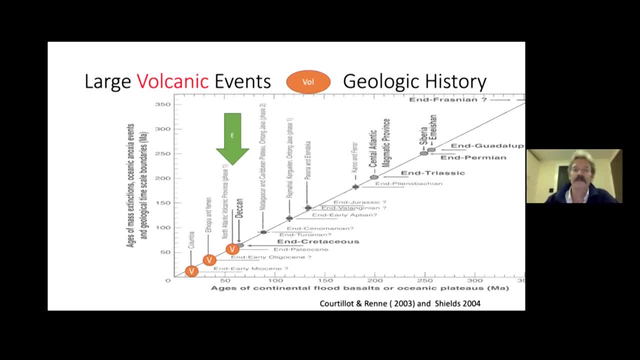 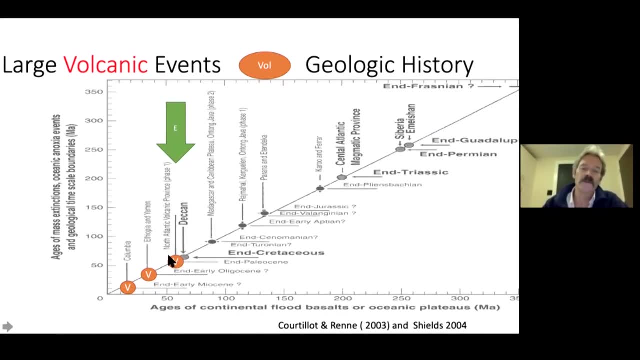 Those are the craters. Now we're dealing with a lot of volcanism in the Earth as well. These are the past volcanic events and these are the ones that these V zones here which we will bear in on because they're within our time frame. 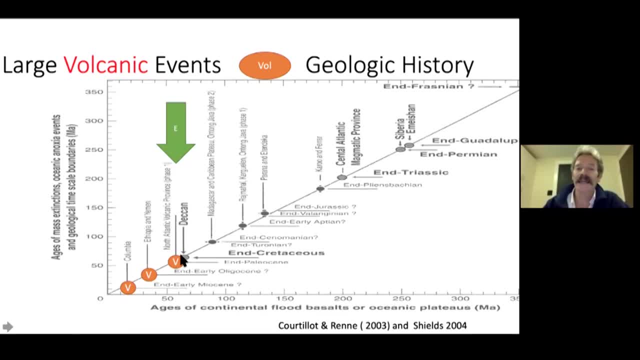 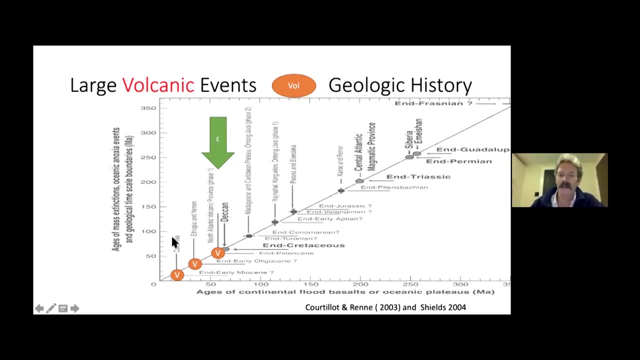 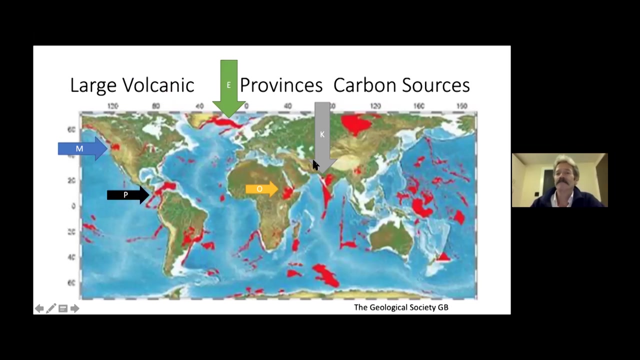 The death of the dinosaurs, and this very large one here, the Deccan Traps of India, are the beginning of the volcanic volcanic situation. These areas here end with the Columbia River basalts And we move through something And This is the location of those on a world map: the Deccan Traps, the Cretaceous K- that's how we'll symbolize the death of the dinosaurs time E. we come over to the Eocene here, which is the opening of the North Atlantic, we'll see a lot of volcanic activity even there today, because of Icelandic volcanism, etc. 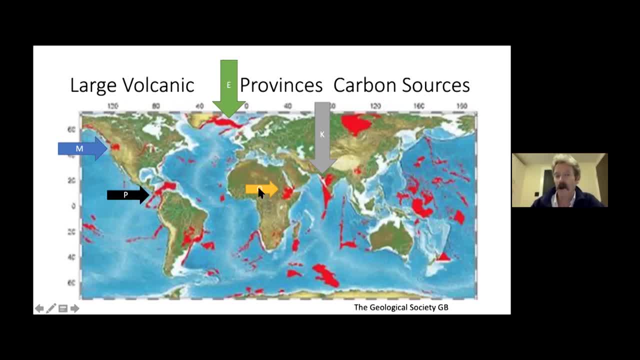 We'll move on to the Olympe, Oligocene O and in the yellow, and this is the area where the large volcanic eruptions took place in the Ethiopian area. We move then further over to something that we're very much more familiar with near home: the huge volcanic area that covers an enormous part of Oregon, Washington and Idaho. 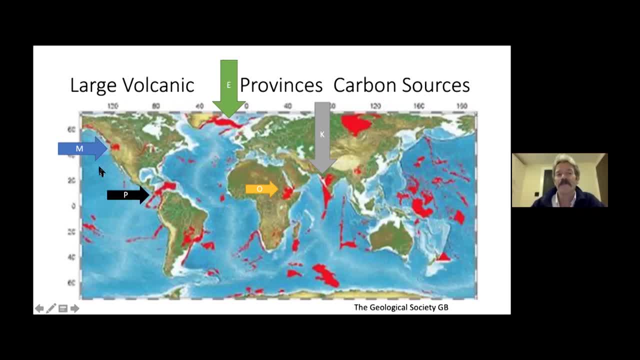 That's the Miocene M, the period of time we'll be looking at related to those. Finally, the Pleistocene, where volcanic- sorry volcanics- eventually closed the Panama Isthmus here. That'll be quite important in the next few slides as we get to them. 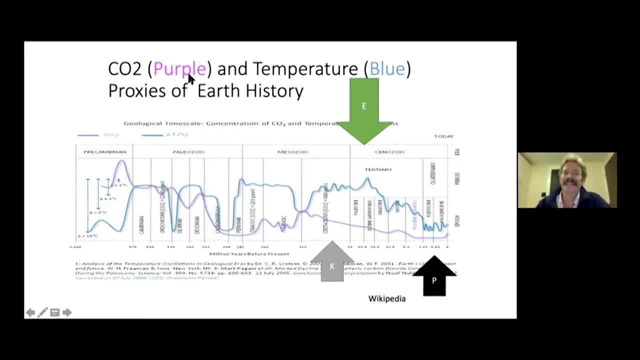 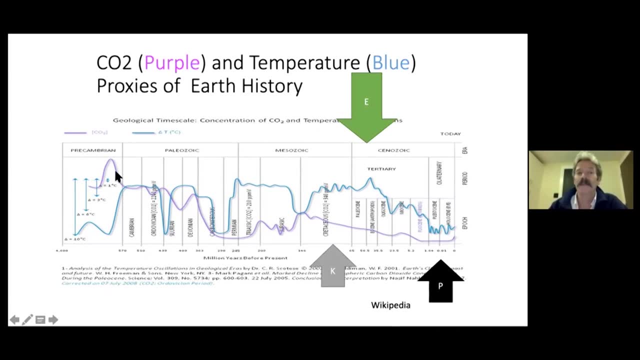 Is carbon dioxide and temperature linked in time. These are proxies. once again, for either one of them, Purple line is CO2.. The blue line Is where the temperature from proxy evidence is shown back in time, the more ancient times. there is no synchrony, no congruence, no way of saying that one is associated with the other. a matter of fact, they're working in opposite directions in many cases. as we move into the current time- the Cretaceous here- and forward K, moving forward in time to where we are today and through the Pleistocene. 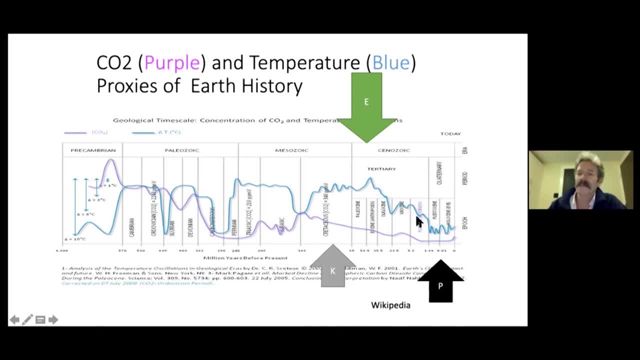 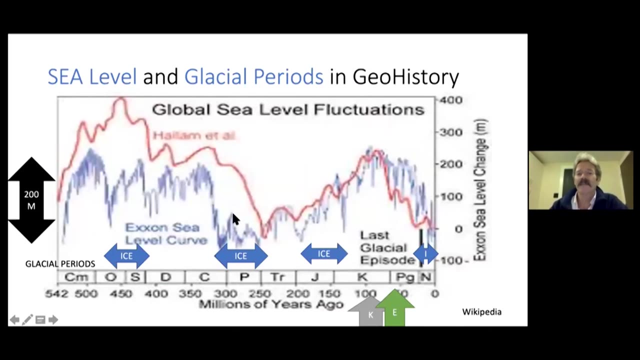 We see a very strong fall in temperature. we see a fall in CO2. This is something we're going to parse out, because could it be that there's some kind of a relationship we're missing here? Sea level, sea levels and ice. 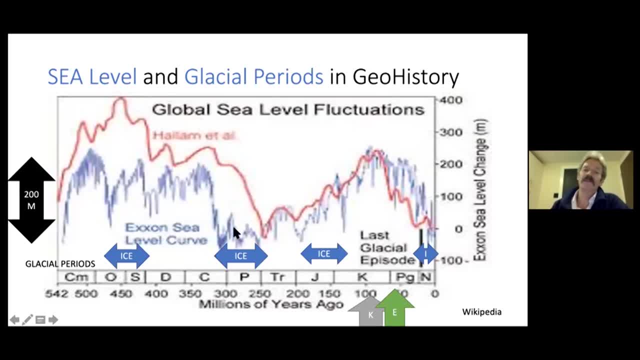 These are the ice ages shown here. this blue sea level line is from a lot of work done, from seismic evidence, old rock records, and look at the entire sea level as it's falling over. here We're falling from something that was in the area of 250 meters of sea level above where we are now down to where. 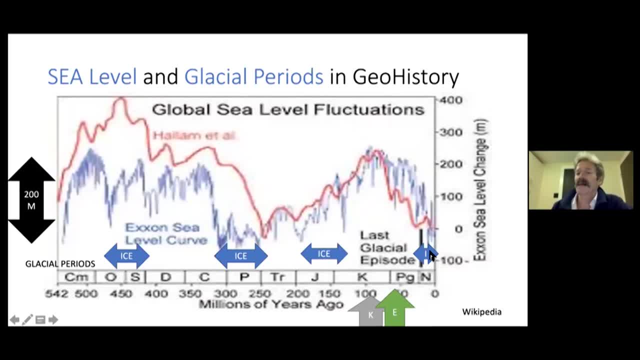 we are now. The ice age is here, the last one, starting with the P area, which should be shown here, but we'll be dealing with only this component of the ice history of the earth and the sea level, history of the earth, declining sea levels into an ice age, Solar ocean currents and continental 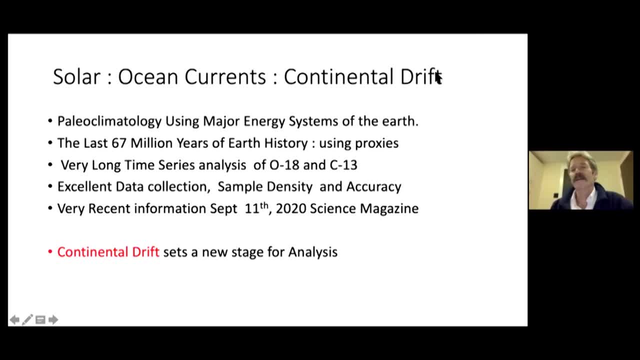 drift will be dealt with this time. What we're dealing with here is another synchrony which we need to understand to work from Eocene forward in time to where we are now. This is paleoclimatology, as I mentioned, It will use the major energy systems of the earth. 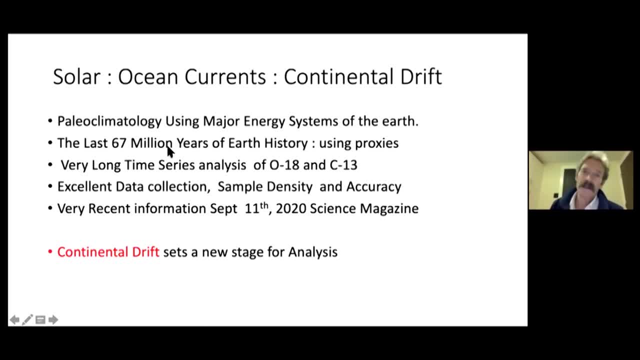 and they'll be looking at them over 67 million years through a recent study. This is the proxy evidence that we'll be using and it's a long time series, as you would recognize, A long time series with great detail within. it is very important to the analysis of any 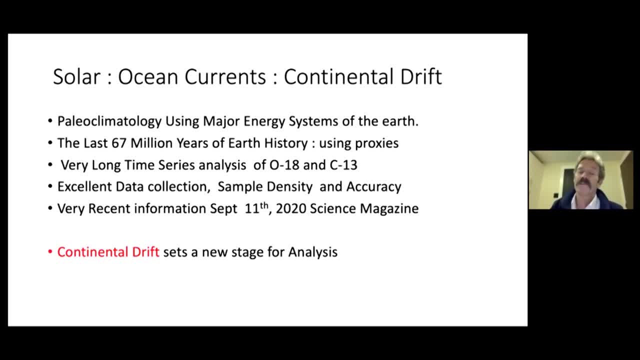 data from any field of science. This is one of the first times this has really been brought together and worked with properly over this kind of a time period, And that's what we're going to be trying to work with today. The analysis will mainly be of oxygen. 18. 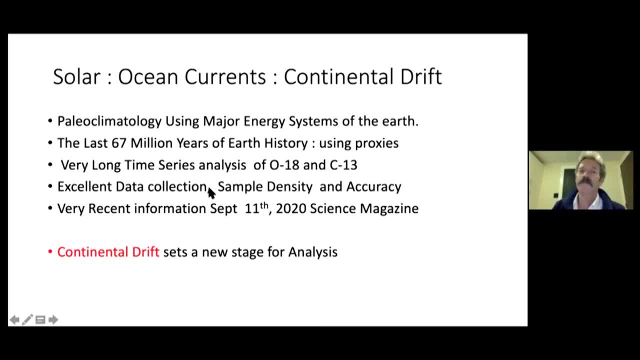 and carbon 13 that we'll be looking at in the early part 1 component of this lecture. The excellent data quality is owed to this science magazine article and all of the good work done by many people over several years. A group of 20 published this from around the world and we are adding to it the additional 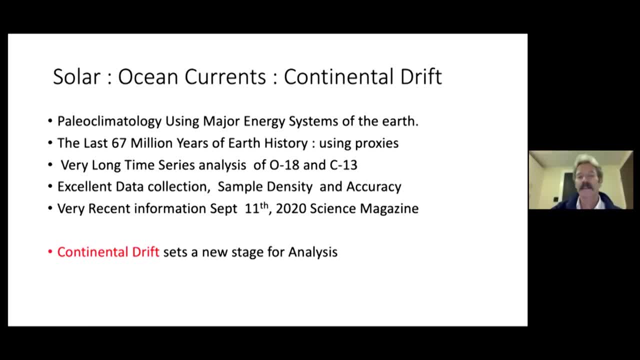 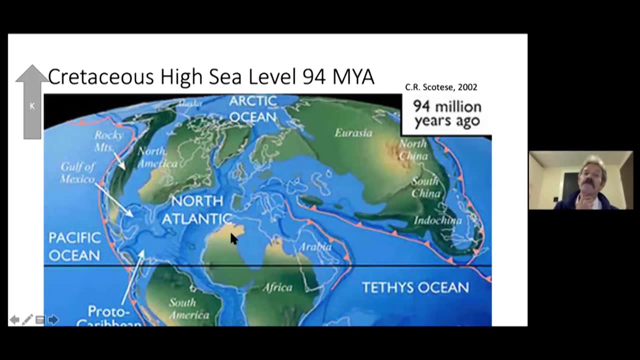 component. That component is of continental drift. Continental drift we'll get into and how the staging of that affects the entire analysis. This is where we're going to start with that: continental drifting 94 million years ago at the high level of Cretaceous seas. the K on those. 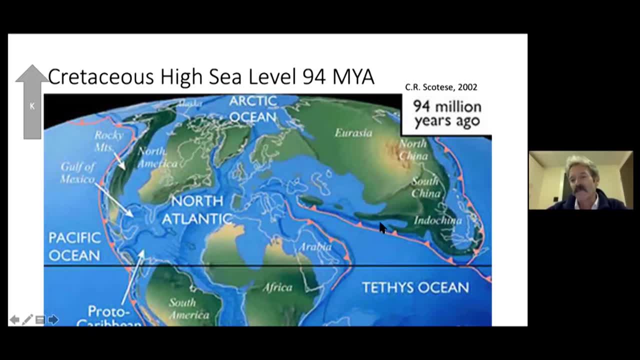 diagrams. What was happening here was we had very large subduction systems. This is like we have off our west coast here, This being North America, Eurasia, Africa and South America. They hadn't quite split apart quite as much as they have now. The Atlantic was a small feature, but what was a? 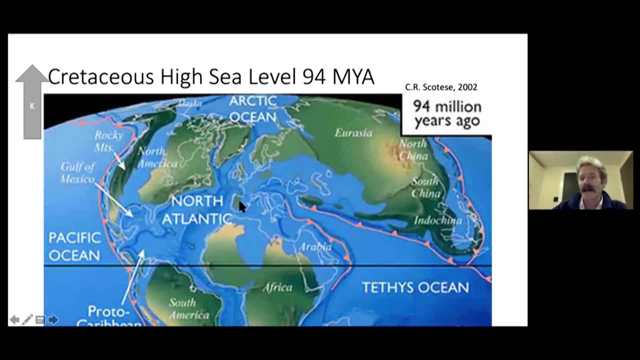 major feature was a entirely open Tethys ocean, which went clearly over to the Pacific and through what we call the Atlantic today. That's going to be quite important in the analysis of what we look at here. So the world was changed. It was changed, it is changing and it's drifting at millimeters a year. 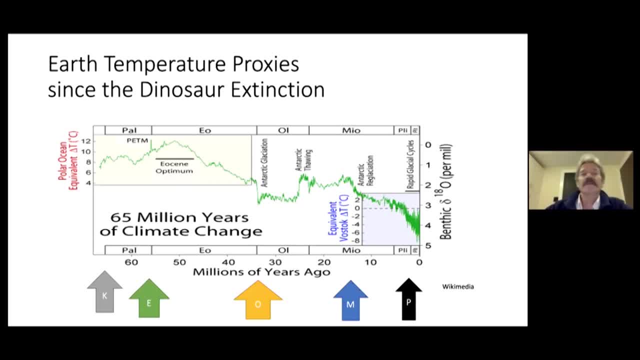 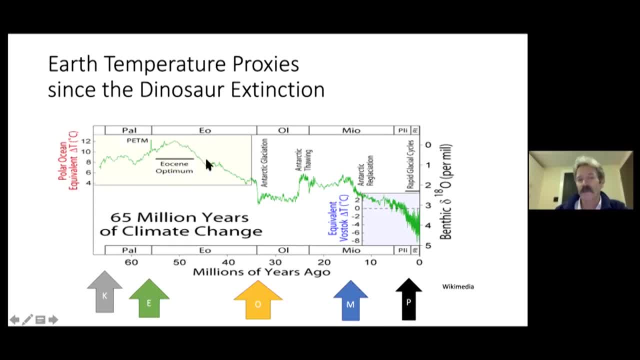 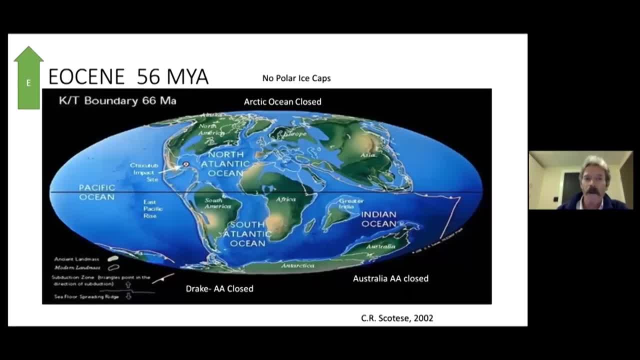 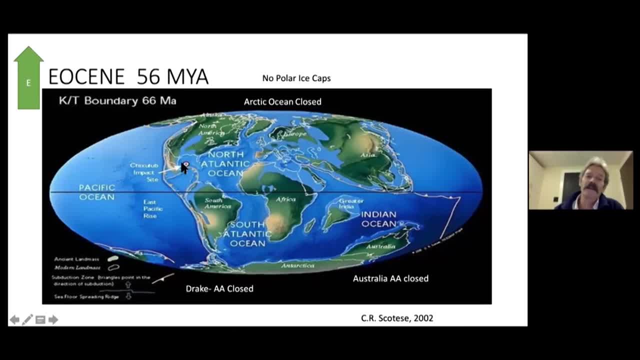 Chicxulub hit in the offshore area, creating a very large crater, and locally it changed the climate for a while, created great extinctions of life, but we'll have to look at that on a broader look and broader scale. What was happening here also, though, was there was a big change in what was happening here along the equator. The equator, the equatorial current, which existed here, was running strong. 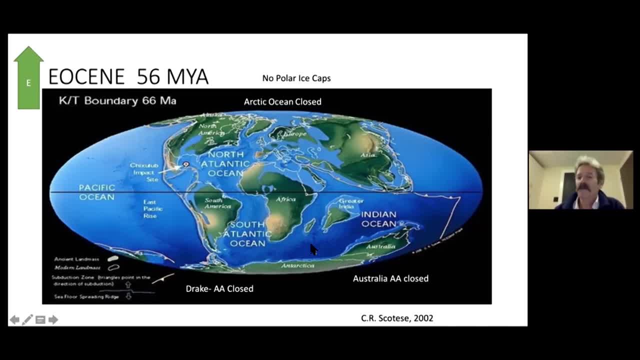 What was not happening was we weren't getting any real currents down here, Why Australia was joined to Antarctica. South America was joined to Antarctica. What we had was: What we had was a closed southern ocean. We had a barely opening Atlantic Ocean. We had a closed Arctic. No polar ice caps existed here at all. This was a total meltdown time. 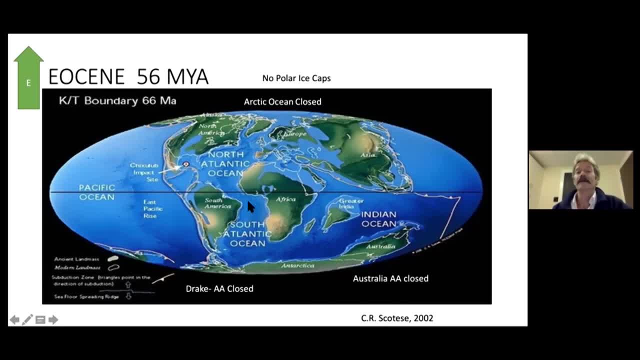 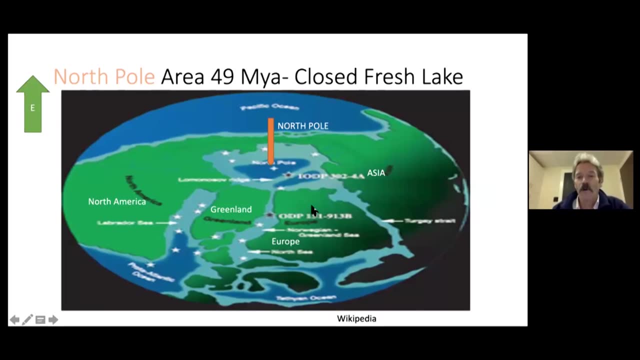 So this was a high period in temperature of the Earth: 66,- 56.. We've got a couple of different numbers here, but 56 million years ago is where I want to deal with At the top of the Earth, the North Pole area here shown with the red was a large closed freshwater lake at 49 million years ago. This has been shown by drilling through this area and, as you see, Greenland, North America, Europe and Asia were joined around that area, not allowing any of the water accumulation to mix with the main ocean systems. 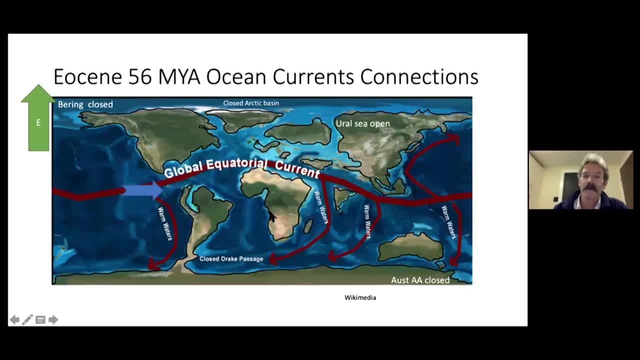 It was a closed Arctic Ocean. The equatorial current at the Eocene was dealing with a closed north and a closed southern ocean. The equatorial ocean was strong In that regard. the equatorial ocean could collect and save and transport energy throughout the then global climate. 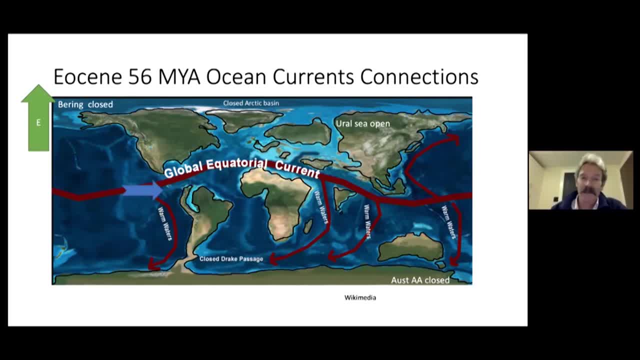 сем machstur that power. So this was the driver, even though the Sun, of course, was the major driver. this was the driver of all of the moderating things that happened at that time. as you would recognize, today that happens to us because of other near equatorial currents, like the issue of the South American currents that we'll talk about a little bit later on. So this is the driver, especially if the sun's already out. as you see, here in that area, here in the US, This maybe happened 20 years ago, at pretty high altitude I think, But it did here as well, But it was never the sun. 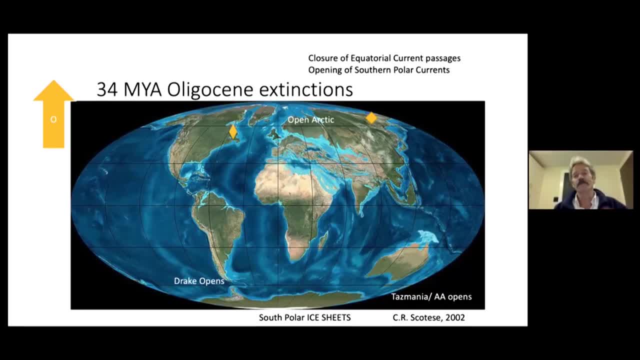 And in the 22 year period it winds back down as well, Or the sun is picking up. attention to many, many more hues to come out here. scene. now we're moving to the o, the o arrow. we're at 34 million years and there were some. 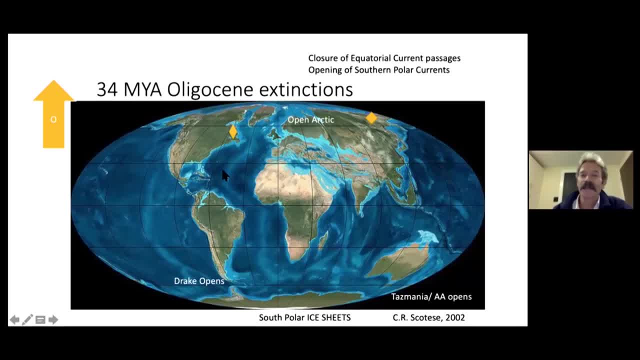 extinctions at this particular time. what's happening here? what happened to our passageways of transportation of energy and keeping energy going in the system? and and heat, of course too? as i forgot to mention in the last slide, india was sitting down here. it is now slid up to. 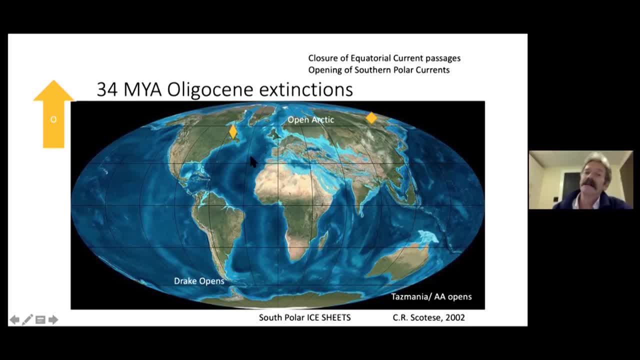 close or semi-close the passageway for that heat. the arctic is opening at this particular stage. the drake passageway is open and the tasmanian australian area over to antarctica is opened. we are getting the beginning of southern polar ice sheets only on the south pole, so this is a 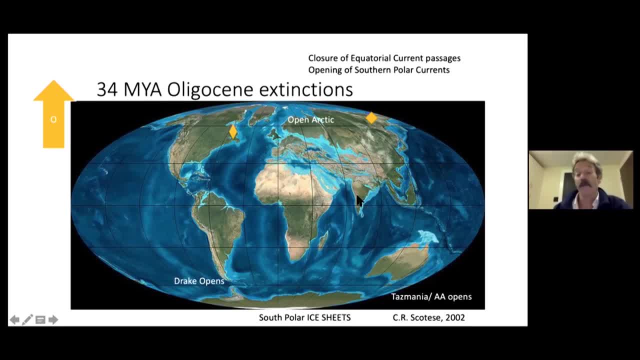 the ability to get tremendous heat movement, although it's still happening to a degree through some of this uh seaway, the shallowing seaway here and through. here, we're not getting it as um, it's not moving the amount of water that it needs to be able to moderate the the climate as 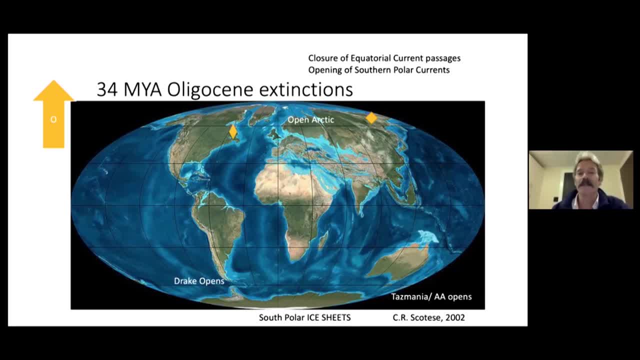 much as it can back in time or it could back in time, the two diamonds there. the other two zones are in the chesapeake bay area right here and the other one um in the siberian area back here. they're very large and we'll see whether they impact our climatic um proxies or not. that's going. 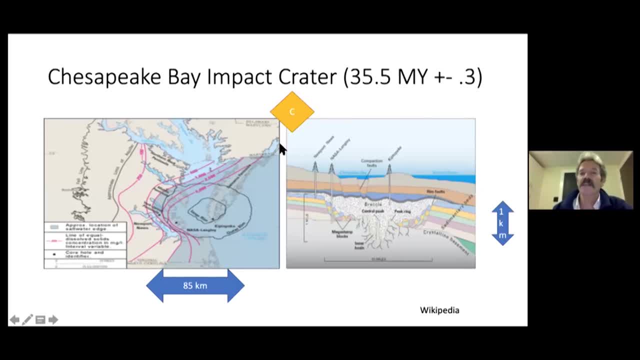 to be important to us to understand as well. this was the chesapeake bay crater. it was a kilometer deep. it hit right here in the chesapeake bay area in the old legacy. 85 kilometers across is its and uh, we are fortunate um to be able to look at a lot of that because of drilling that's been. 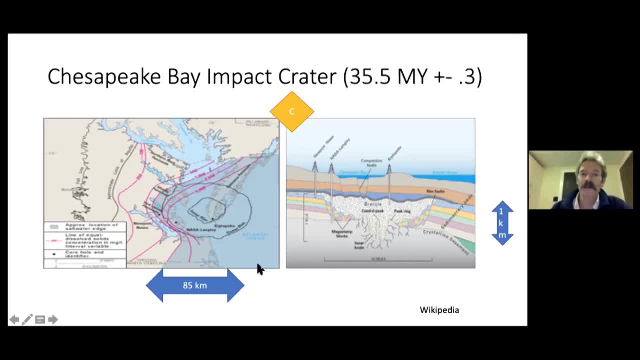 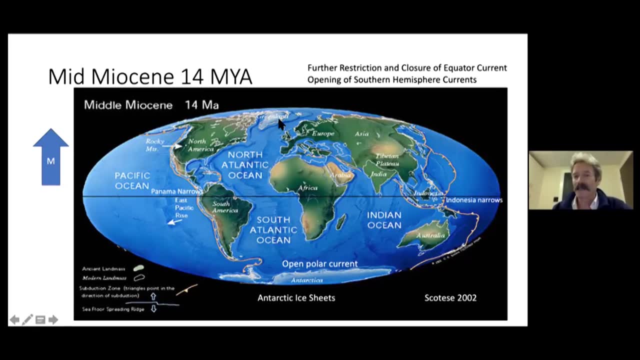 done. uh, all around and through and into that portion of the middle miocene is another drift. now we've got a much more open atlantic, we've got a bigger area here. india, of course, is out of the way, but what's happened here is we're closing the alps. we're actually closing through turkey. 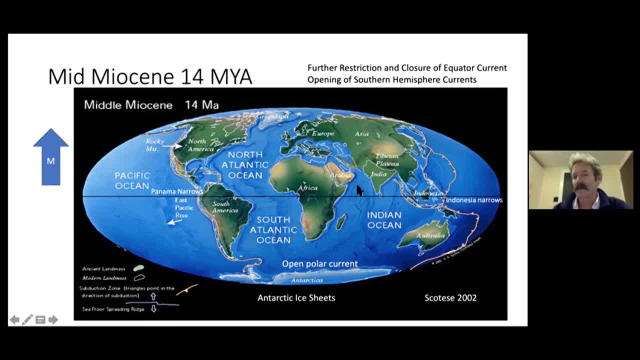 and into europe. we still have a passageway here, but it is barely open. we have a narrowing also of the panama canal area, so that large circumpolar area is not as open as it was. indonesia is also closing up on us. this all because of continental drift, and these big subduction systems are the the uh, the trenches. 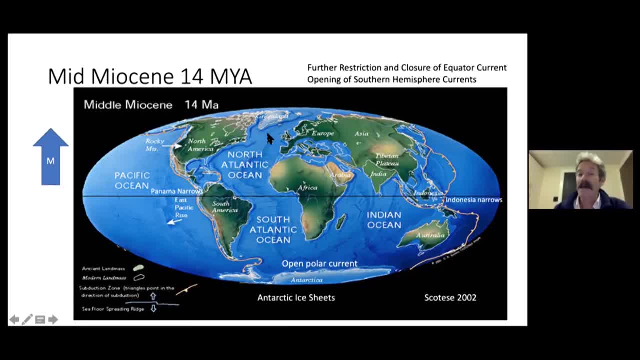 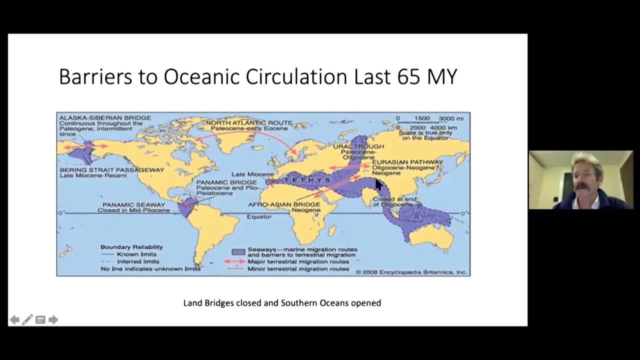 uh, the driver, of course, of that is along the axial portion of these openings where we have vulcanism happening on the bottom of the ocean all through here. so those barriers can also be seen in migration of animals. the migratory pathways you will recognize maybe as being things like the one over in the bering sea which had closed, of course, allowing 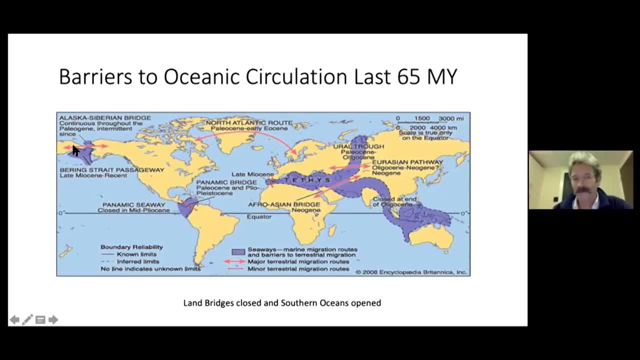 migration across of horses, of mastodons, of woolly mammoths, etc. and many other animal groups. some of the other ones- the panamanian one is classic for this but of course the timing of that- they weren't able to get across these areas in a very meaningful way until 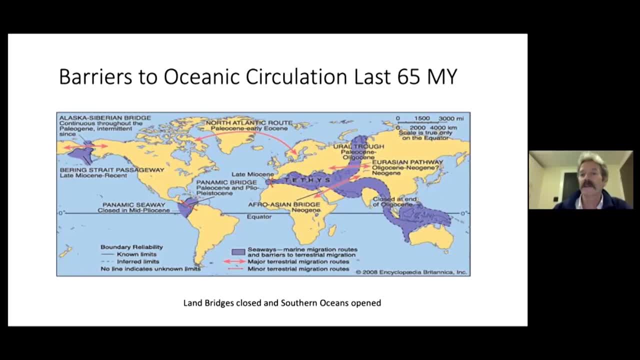 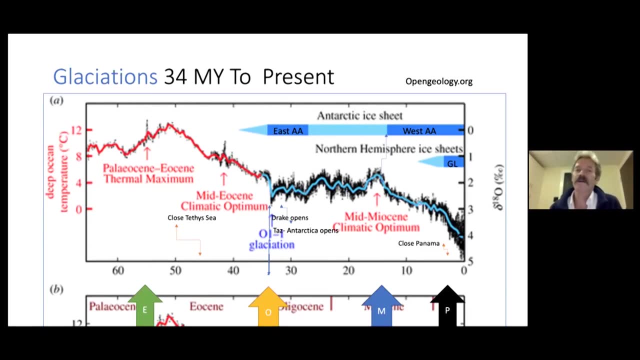 the continents drifted into the positions which closed those. what happens when you close those seaways? the one around the equatorial area specifically, was closed, the tethys sea closed. that's the oligocene we talked about, that eastern antarctic ice caps formed. it was a minor um destruction of some of that ice capping here and then the western and the eastern. 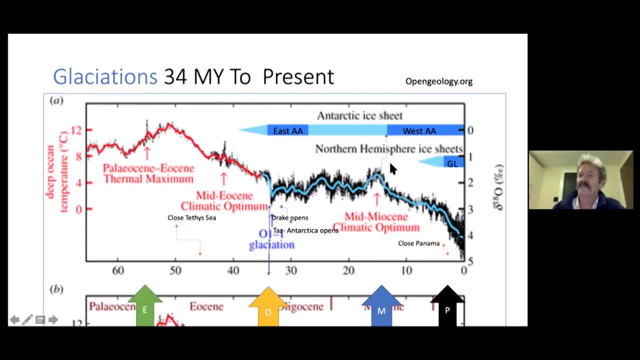 coalesced and joined and became a very significant ice cap at this particular time. here now, as we move into where we are now, the last thing i want to draw your attention is that panama is closing. right here you notice the very sharp drop in temperature, and all of this data is given. 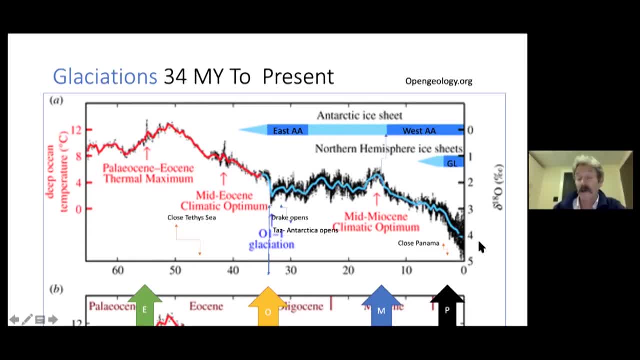 to us by organisms, organisms and sampling of those organisms for their oxygen: 18 isotope concentrations versus oxygen 16. it's a very accurate isotopic determination which is sensitive to temperature. the drake passage opened and tasmania antarctica opened, of course, within the period. 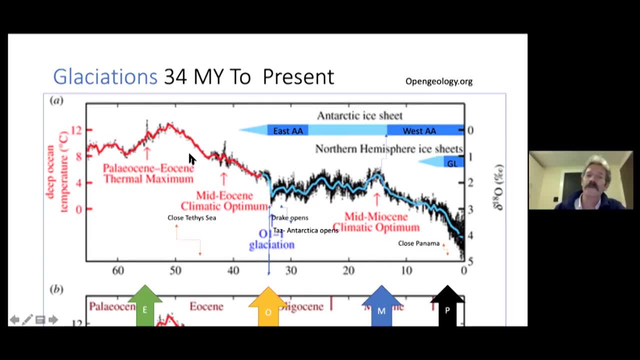 in the middle there, right when the big ice sheet started forming over in here, we had the thermal optimum and the tethys c was closing, closing, closing, shutting off the ability to make the ice axis form and move temperature around. look at how even and steady this is. we'll bring that to your. 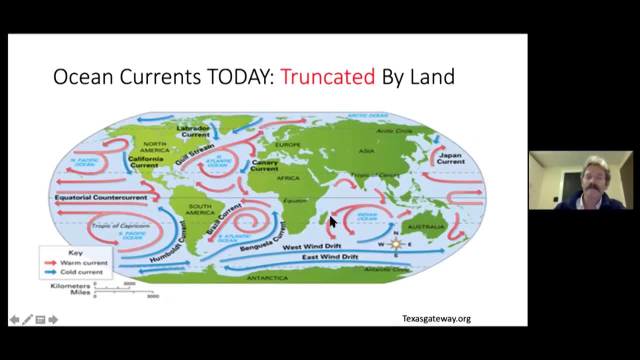 attention between o and m in the future. here the ocean currents today are very truncated by- you know- comparison. we can't possibly say that we can build up that kind of uh energy within the ocean systems to drive the energy and the climate in the same way, but we can to a degree over here in. 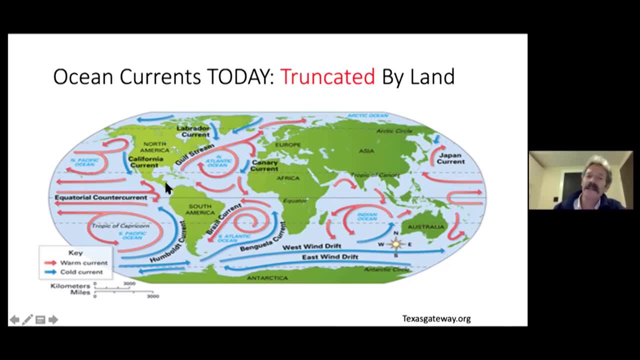 the equatorial currents, as i mentioned to you, you hitting the edge of south america, not being able to get through the panamanian canal area. they do drive el nino and la nina, conditions which affect the entire area here for its climate gulf stream is here and it affects all of europe and its climatic variations. if the gulf stream 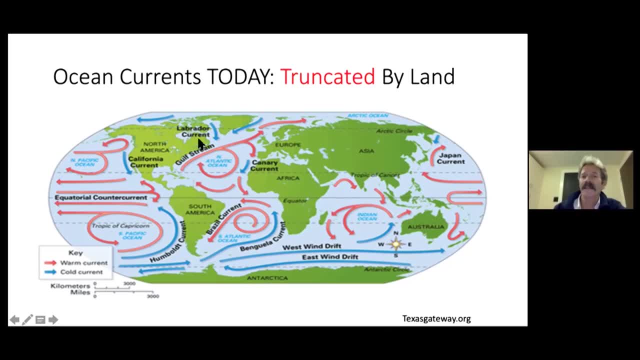 were to shut down, europe would freeze over the latitudinal component of europe. having all the warmth it has is all because of the moderating influence of the gulf stream current. there are other currents which we won't go into, which do also moderate, but they don't have anywhere near the 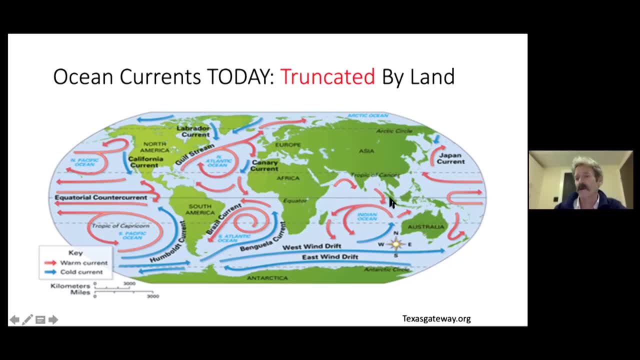 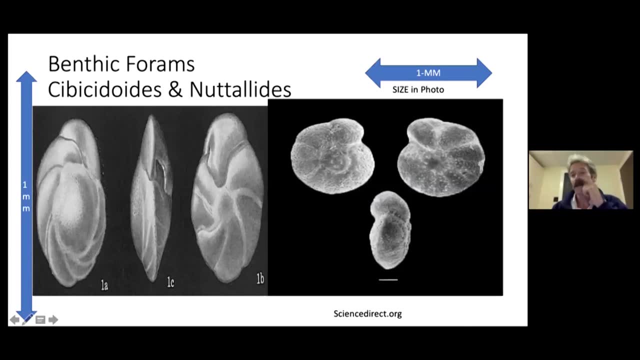 cumulative saving power or storage power that a current that used to move through here does in the past. these are the organisms we're going to try and study through. so we're looking at taking pieces from their shells: calcium carbonate, which stores the carbon and the oxygen from the past. from looking at these very small 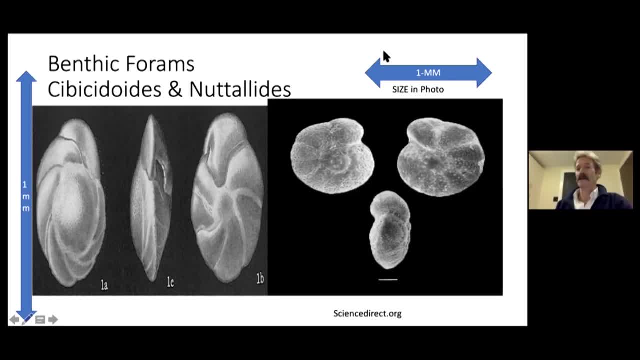 beasts. as you see, a millimeter is what we're dealing with here, and over here we'll be dealing with a very small size fraction that lived on the bottom of the ocean and received its food supply from the surface. it was looking for its food and it built it into its shell, and a shell has preserved. 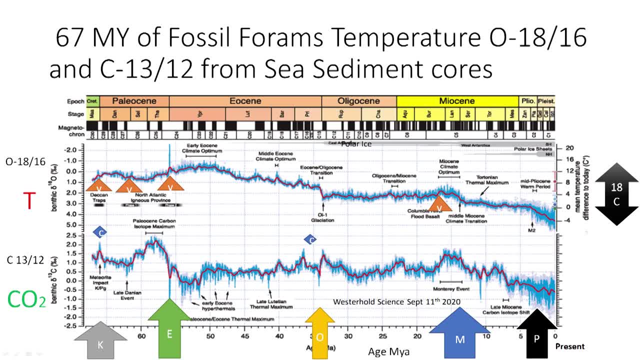 the state of the ocean at those times. 67 million years of fossil forum evidence. those were forums that we looked at. we'll look at the carbon and we'll look at the oxygen for those, a very complicated, complicated look. it was just done recently, september 11th of 2020. this is the most important article that i've. 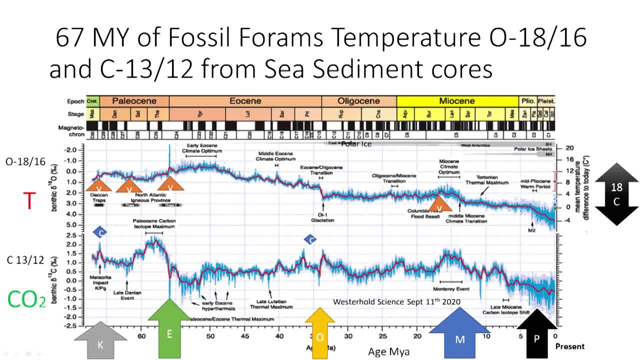 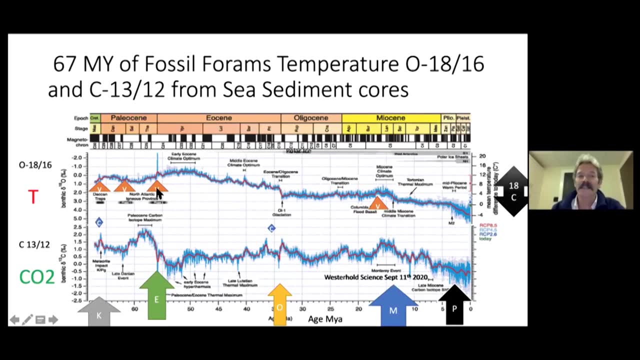 seen to comment on the developments of the ocean, um comment on this period of earth history that exists and it's integrated, of course, a lot of people's work from the past. The 20 authors here have shown us where the volcanic activity was. 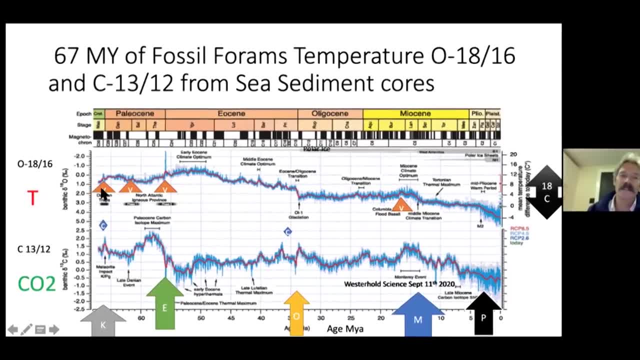 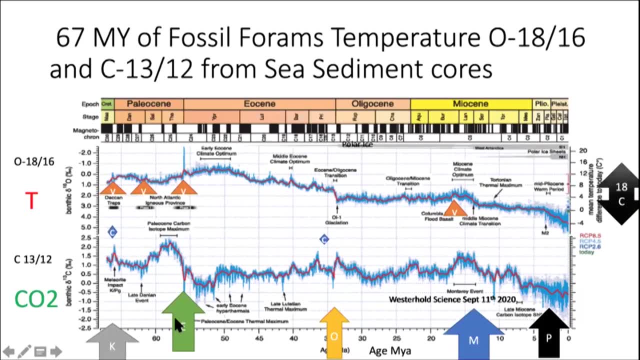 taking place. This is the Columbia River Basalts. This is the Deccan Traps. This is the opening of the North Atlantic. With respect to this time, we will be looking at time across the bottom of course, the age in millions of years, with the Eocene here, Oligocene, Miocene and Pleistocene. 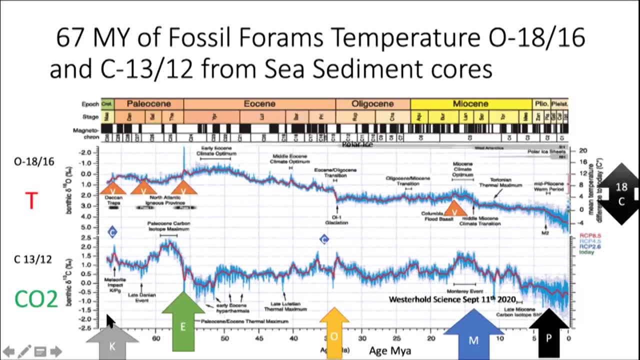 The Cretaceous. the death of the dinosaurs is on this side and we'll look at the impact of the Chicxulub crater. here. We'll talk about this lower scale really, which is carbon isotope ratio as CO2, just in layman's terms. for now, What we have up here. 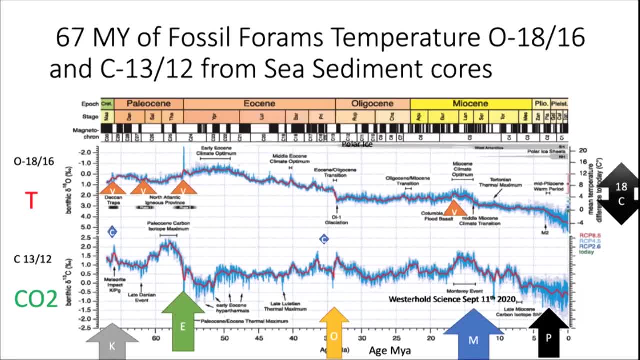 on the top is temperature. Temperature is given to us by the oxygen-18, oxygen-16 ratio which is within the organism's shells. The blue are the error bars. That would be the extremes within the measurement of the actual oxygen isotopes. within this, some really big departures. 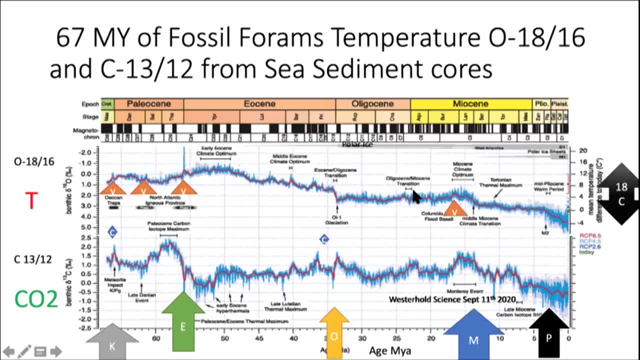 like this one, some other spikes. This is the very important portion at the Oligocene we're talking about. The lower one is we're calling it carbon dioxide. It is the benthic organism's ratio of 13 to 12.. 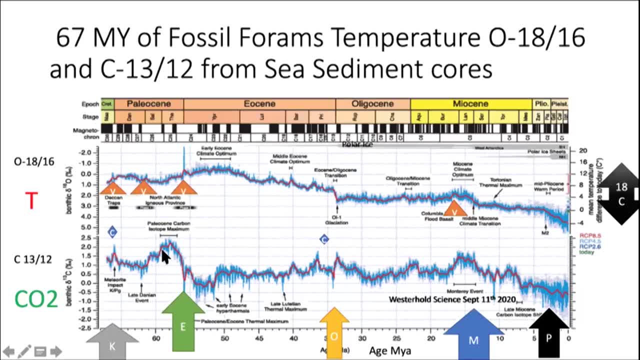 It has the impact crater shown here. It has some very radical changes as we're opening up the North Atlantic volcanic in origin. very likely We get changes after that plunges ups and downs. We're going to look at the comparison between these two data sets over. 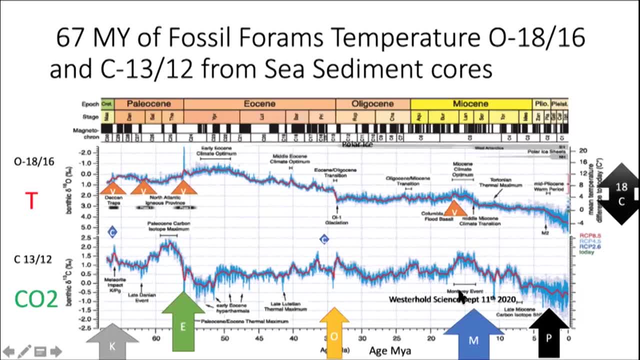 time, a very long period of time, through the work of these fellows here. Now you know that we were changing the continents through this area and looking at the geology of the situation. they didn't get into that in their paper. They did address the polar ice caps and when they formed. 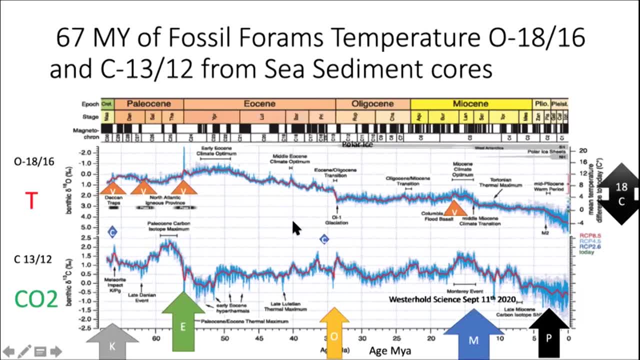 and when they broke down. They didn't get into that in their paper. They did address the polar ice caps and when they formed and when they broke down, They did address all of the other major changes that took place at these spikes within. 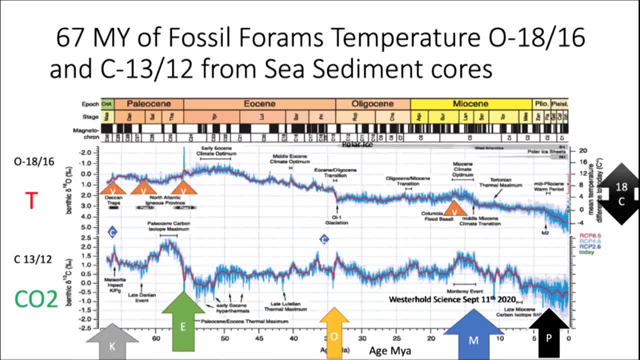 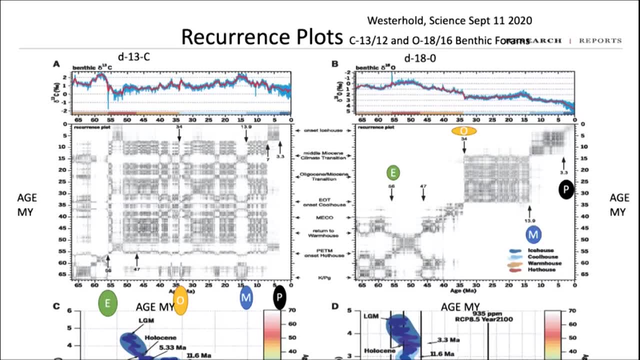 changes of carbon or changes of temperature. This is another part of their paper. I think this is a way we will have to start to look at a lot of information. that is, long time series with a lot of data. It's a technique generated out of chaos theory, Chaos theory. 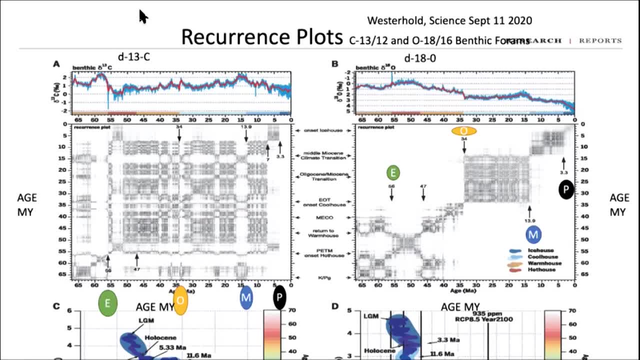 is to try to make sense out of chaos. People looking at these curves just in isolation by themselves couldn't have arrived at the conclusions that now can be made by taking these and playing them out through time. What we're dealing with here in a recurrence diagram is time. 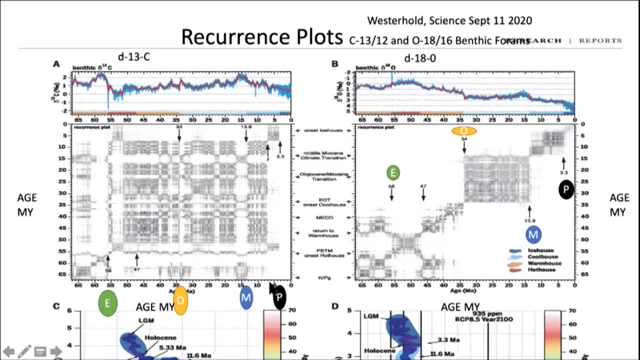 zeros through 65 million years. We're taking time here on this axis: zero through 65 million years. We're looking at the carbon component here as shown above. if I was to take this and turn it on its side and we had the zero now back over, 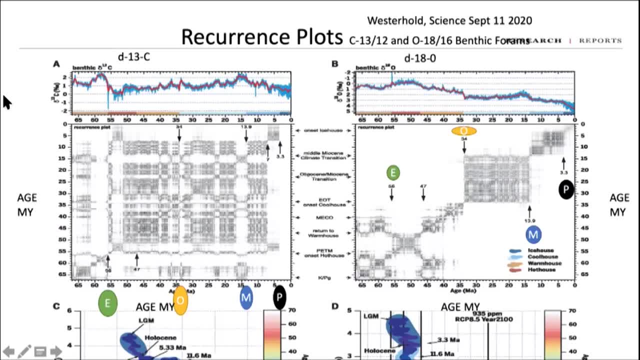 here and we had another one of these on the side. you would then see what the recurrence diagram is really doing. It's looking at when these events recur in time. I hope that's explaining it enough, but it's something that you should probably look into. It's a great technique, What it does over 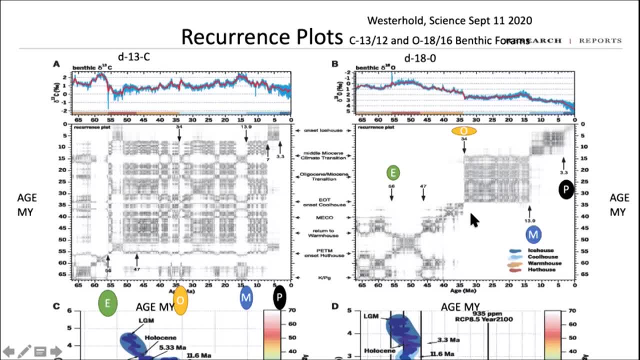 on this side is it looks at temperature. What is radical here, and the thing that struck me the first time I looked at it, was how different these two representations are. What we are dealing with is the direct comparison of change. Now, this is a very even area. I mentioned it as we were going. 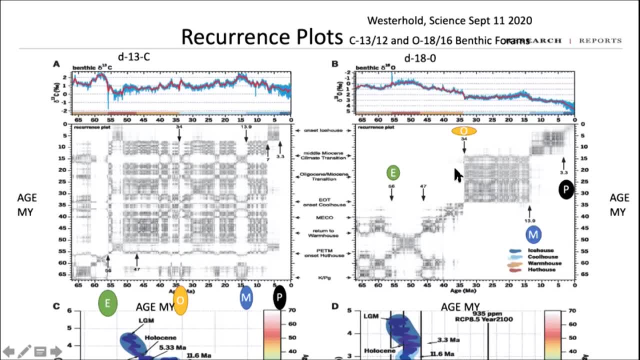 through it. This is a period of time which was very calm and settled. Then radical change took place. This is looking at the temperatures through that period. What we're looking at over here is the carbon that maybe or maybe not have had an association with the temperature. What is? 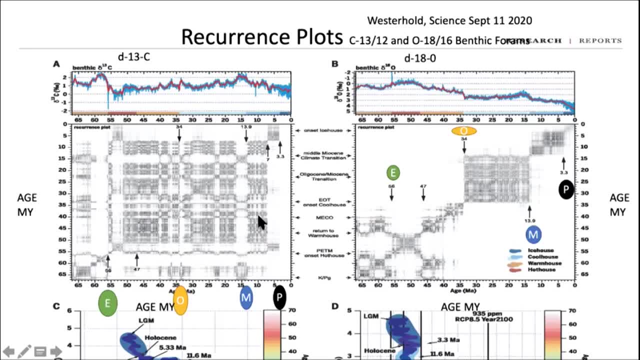 striking is that they are radically different. They share some of the same boundary conditions, but their pattern in general is discordant. It does not match. That was one of the things that leapt out at me in looking at this. I think 4M information on a recurrence plot basis that they generated. 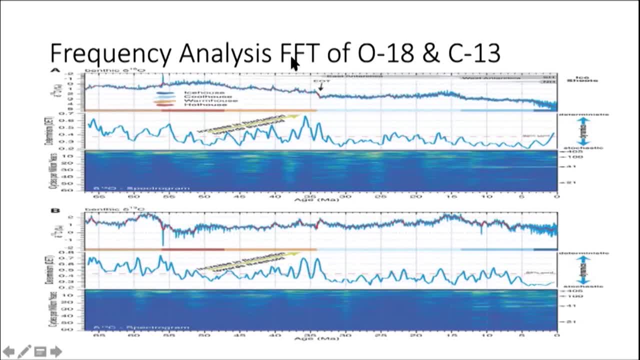 What they also found was in a frequency analysis, an FFT, which is something that most statisticians would look at in data of this intensity and this complexity. they looked at it for those isotopes as well. They found that there were streaks of frequency congruence, let's call it. 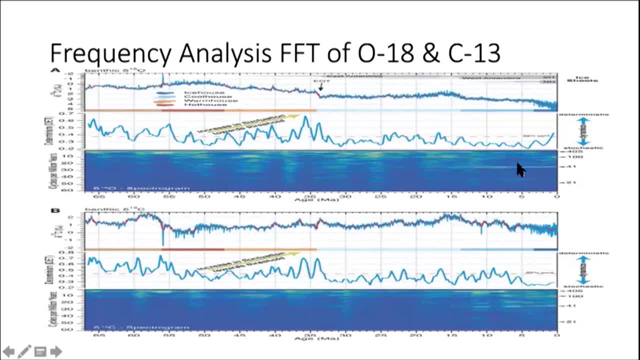 where one would overlie the other and reinforce it. Then there are areas where it's not reinforced at all. We can look at that in the two data sets. but the thing that they found independent of looking at the cycles of the Earth-Sun system, which is something we will develop in a little- 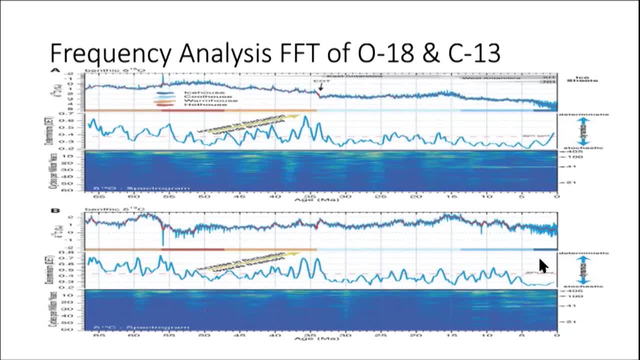 bit. they found independently that they could see in the data all of these, what we will now call Milankovitch cycles. The Milankovitch cycles will be talked about a little bit later on, but they're all to do with how close 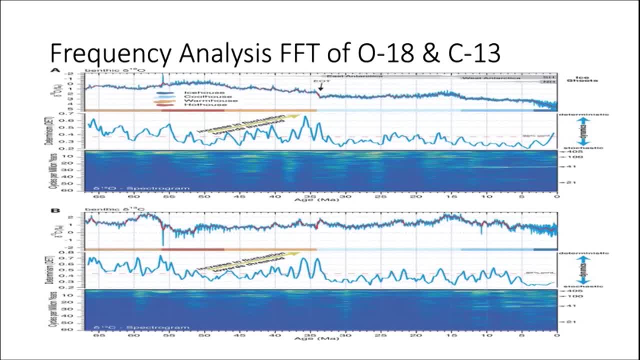 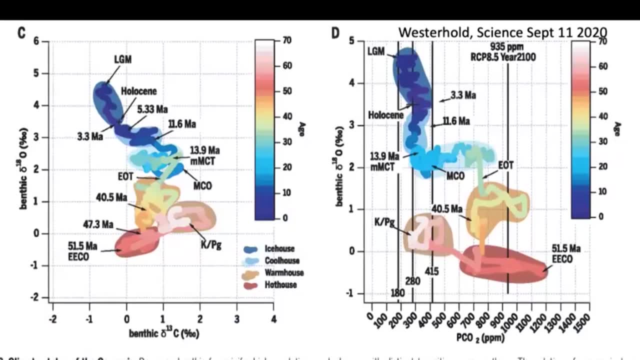 the Earth is how the Earth is tipping, et cetera, to the Sun. We'll move on from this one to a complex representation from the same paper, which talked about moving across CO2 barriers. What we want to do is modify a little bit of structure. 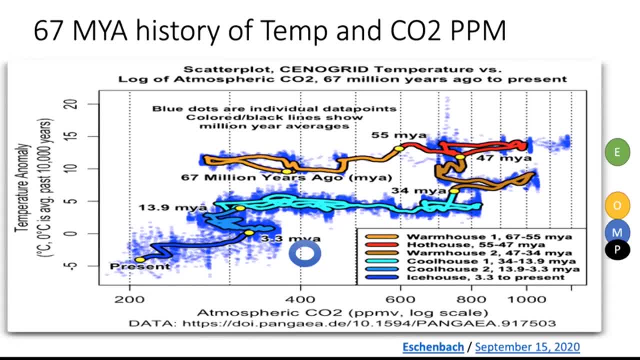 What we want to do is modify a little bit of structure. What we want to do is modify a little bit of structure of what they did there. We want to stretch it out onto a long logarithmic base here on the lower side. I'll go back quickly. What they had here was CO2 in parts per million versus temperature. 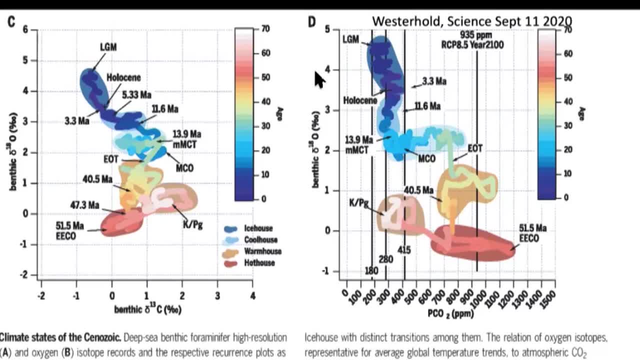 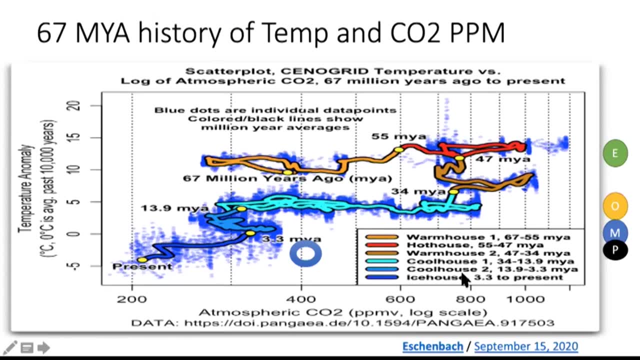 here. They put the temperature at the top, with the lowest temperatures at the top. I'm going to switch that around, is what I'm going to do. So with this one, this representation here by this gentleman, on September 15th, right after seeing their paper, he put together this And these blue: 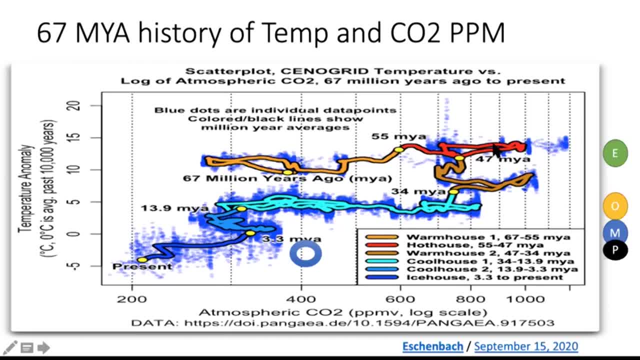 dots are their data points all spread out on a temperature anomaly versus CO2 parts per million by volume log scale on the bottom. What this is on this side is the temperature in degrees C for average in the past 10,000 years. So that means the last 10,000 years of time is the zero That's our current time back. 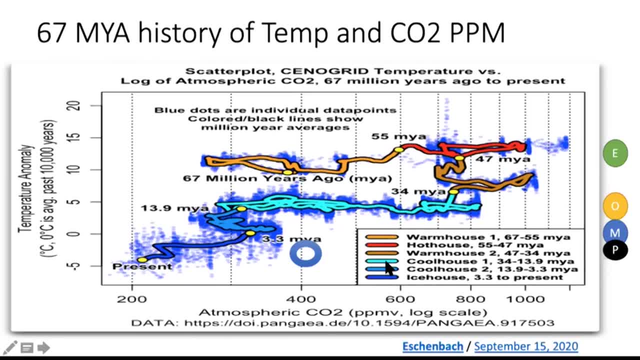 in the Pleistocene, that period of time where we have continental alignments, et cetera, that are modern. As we moved up here we were dealing with some of those old periods of time where the continents were into totally different configuration: the Eocene, the Oligocene, the Miocene. 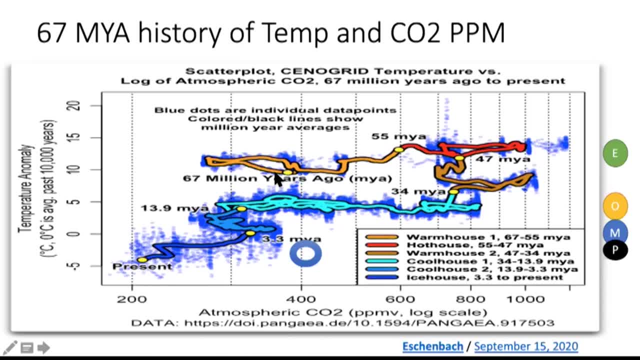 et cetera. As you see on here, the millions of years are quoted. So where do we start this graph? We started at 67 million years ago And we take an excursion out the left side and we move to lower amounts. 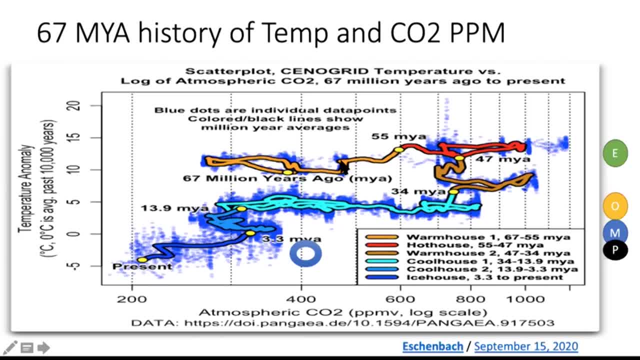 of CO2.. We then move back as we progress in time toward today to 55 million years ago and into the area of 47 million years ago. What are we doing? We're moving laterally through CO2 space. That means that CO2 could be any value between these end members And the 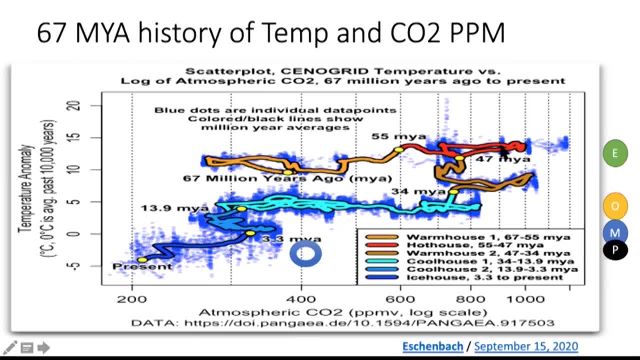 temperature didn't vary. The temperature stayed at a plateau. We call these steps or plateaus. Steps is something that I've used. How high did some of these steps get? 2,000 parts per million here in what they would color red in their representation? 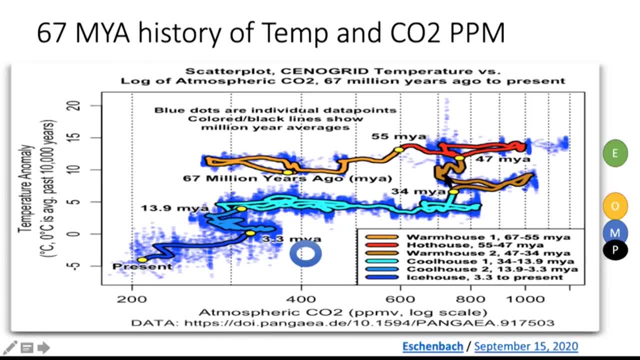 And he has done the same thing and honored that as well. It moved down quite radically at 47 million years ago to another temperature step which it lived at for quite a long time: 47 to 34 million years. It eventually moved to the one which I was calling the long steady period here down in the 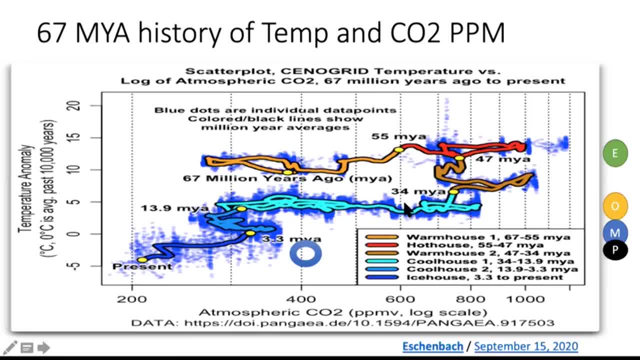 Oligocene. The Oligocene step itself varied between 850 and 850 million years ago, And that's a lot of difference between a number that is around the same temperature. So we're moving the temperature from 850 parts per million CO2 down to something that was less than 300, 280 parts per million. 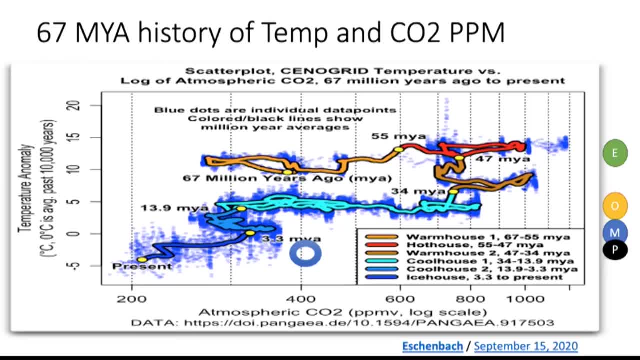 A number that is quite an interesting number from a glacial point of view. We'll talk about that later in part two. So all of these things are a little detailed to work with, But I'm hoping that what I've been able to illustrate will then help us to go to the present. This is a present built on. 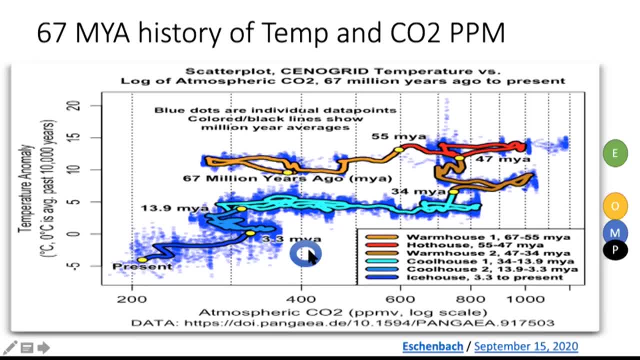 10,000-year averages. It's a present built on 10,000-year averages. It's a present built on 10,000-year averages, And what we see today is something here that changed or started to change, and go down at 3.3 million years ago, when Panama closed. 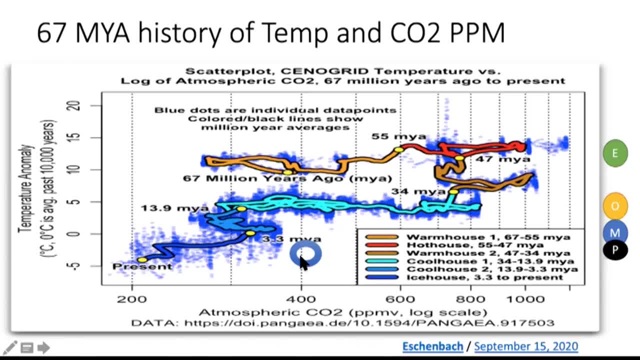 The blue dot is a rough area for 410 parts per million, let's say in the atmosphere as measured at Mauna Loa. So that is there. We are looking at a condition which existed in all these blue dots through this entire period of time, from 3.3 million years ago to today. 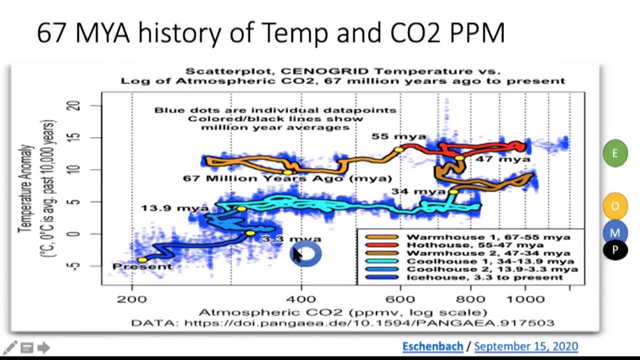 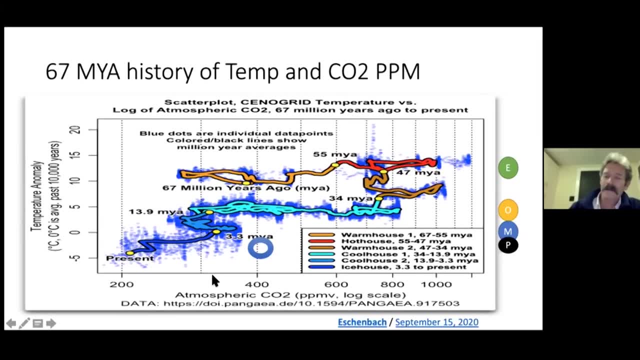 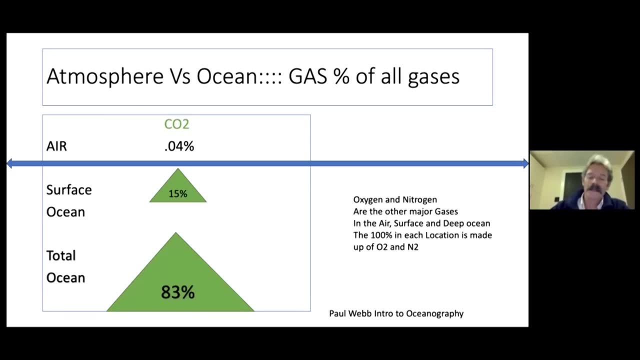 And then our comparison of that shows that we've moved out to 400 parts per million along that same step. What is going on with carbon dioxide? Why is it showing up all over the map And why does it move from some fairly radical numbers to relatively reasonable numbers without changing temperature? 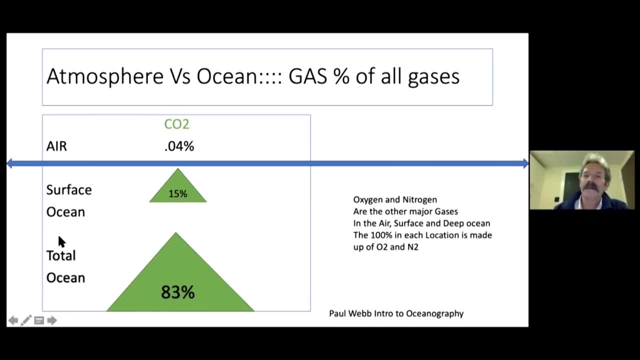 The ocean is a dynamic system. The less dynamic part of it is the deep ocean. The deep ocean which is shown here more in the total ocean, which is the combined number. If we look at the gases within the ocean and the percentages, we would have oxygen and nitrogen making up the rest of the 100% here for the deep ocean. 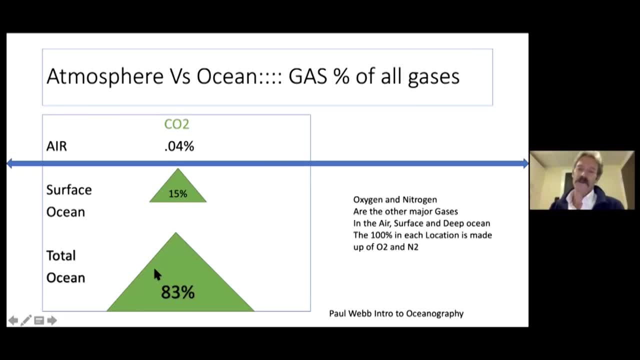 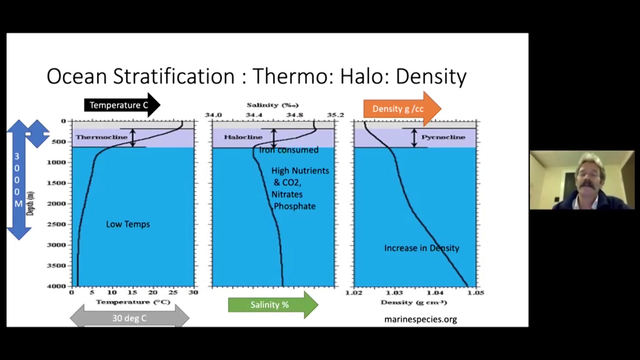 But the carbon dioxide is dominant in the deep ocean. Oxygen and nitrogen are minor players In the shallow. we have a small number as well of carbon dioxide compared to oxygen and nitrogen. What happens when we move that stuff up through drifting continents and creating obstacles for it to move across shallow seaways? 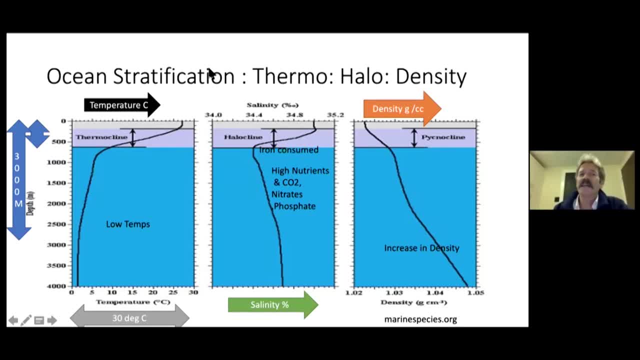 What I'm showing here is the stratification of the ocean. It's the thermo halo and density components. The thermo, the temperature is here. There's a thermocline, a very strong break between the surface temperature and the ocean. 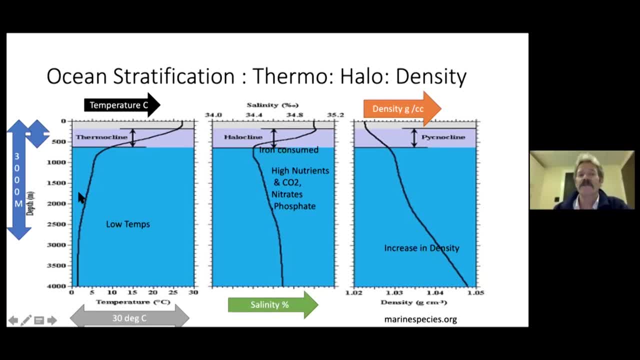 The thermocline is the temperature and the deep temperature. CO2 likes cold water. It is soluble in cold water. A lot of other things are too, and they stay there in the deep: The nitrates and the phosphates which feed fisheries, which feed life in the ocean. 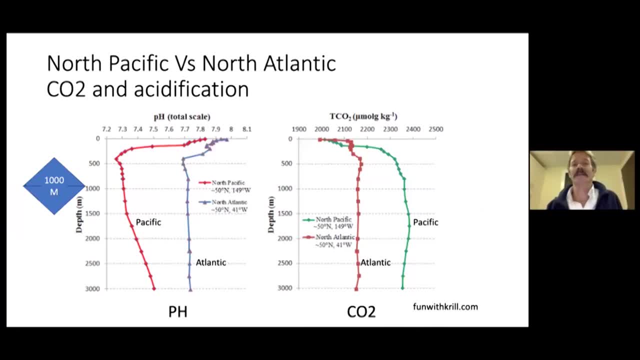 CO2 is a life-giving situation as well. If you look at the CO2 shown in the Pacific Ocean here and the Atlantic Ocean here today, they differ. This is because this is young ocean water. This is older ocean water. We'll discuss some of that in a little bit. 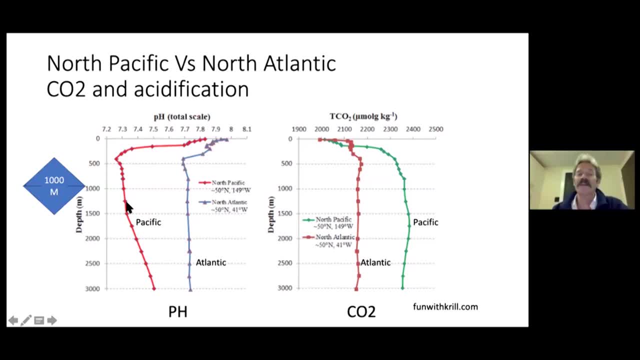 Shown on the pH scale. over on this side, the Pacific is radically more acidic in the deep ocean, Very non-acidic in the top, of course, As is the Atlantic, But the Atlantic steps over and is much less acidic. We will discuss why that takes place as well. 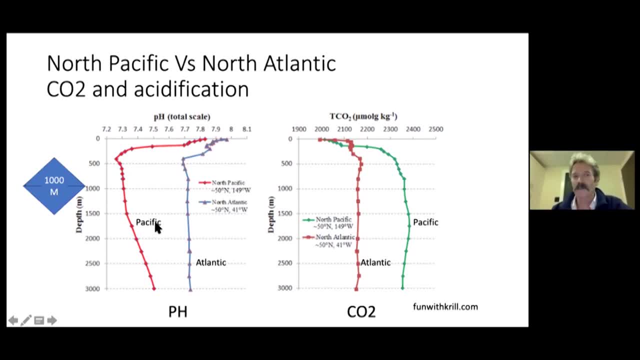 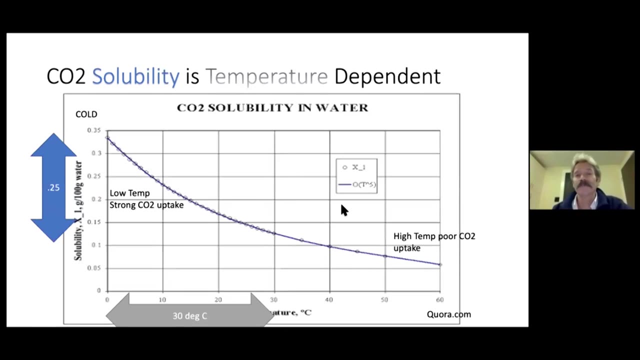 These are thousands of meters over here, as shown in the blue. So we're looking at pH and CO2.. Two things that we do have to concern ourselves with in ocean analysis. This is that solubility I was talking about. This is the solubility curve. 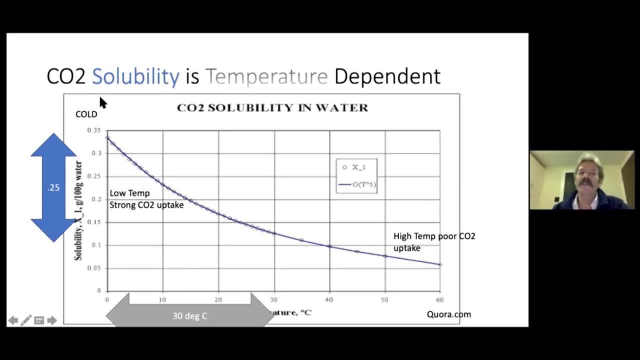 Which changes with temperature As we get really cold over here down to almost freezing at the bottom of the ocean and in the lower ocean. we are dealing with a solubility. The ability to take up CO2 is very high As we move into the higher temperature components of the ocean. we cannot any longer do that. 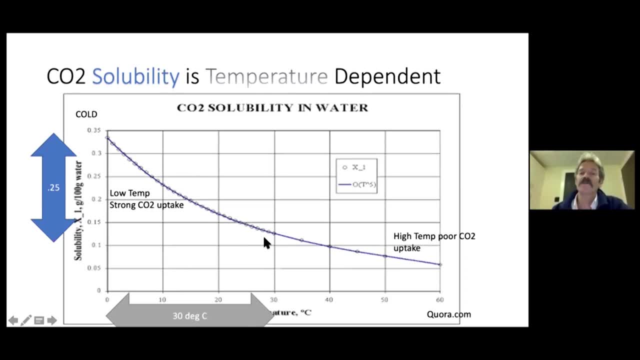 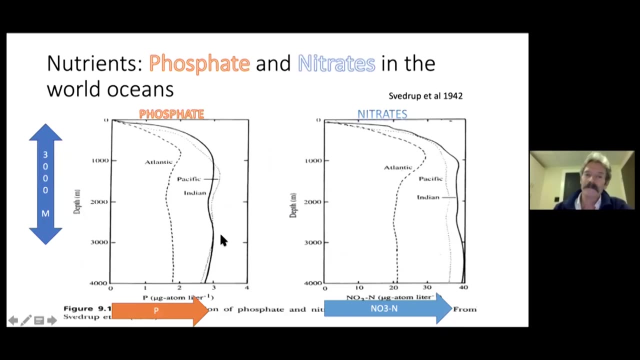 Hot water will not take up CO2 except by bio-remediation or bioremediation Within the shallow water hot water areas. So solubility is driving the storage of CO2 in the deep ocean. Phosphates and nitrates are also solved well, stored- sorry- in the various oceans in this way. 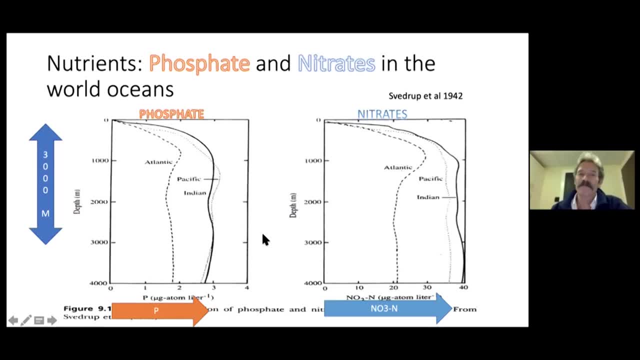 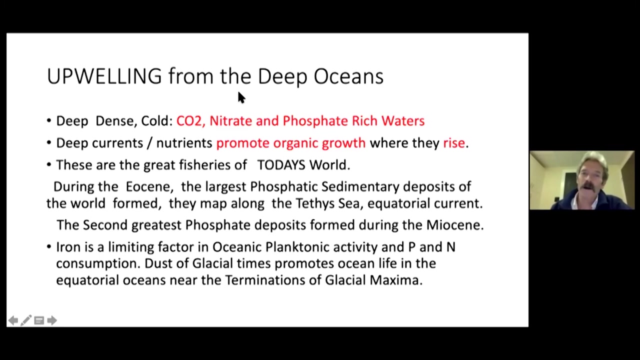 These are very important to the life in the ocean. It's living off of the old, dead material which has been taken to the bottom As it up wells from the bottom of the ocean, coming upwards in the temperature gradient area to the life area at the top where blooms take place, of the fundamental parts of the food chain of fisheries. 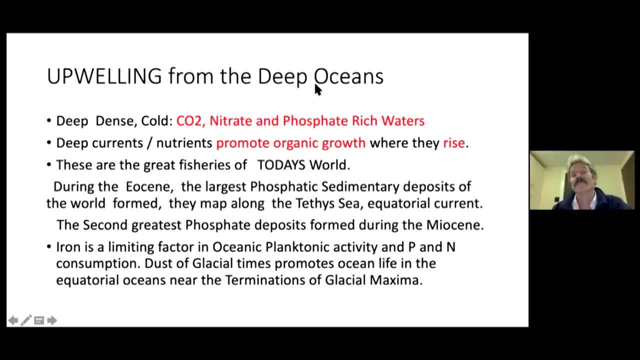 So upwelling- a word I just used from the deep oceans- is what's being discussed here. These deep, dense, cold, CO2 rich nitrates, These CO2 rich, nitrate rich and phosphate rich waters move up. 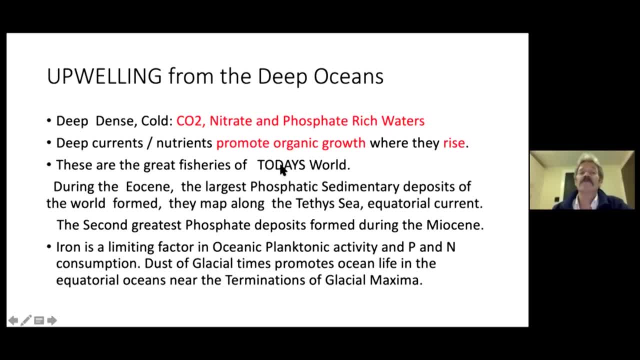 They rise And, as they do, they promote organic growth because of the nutrients they contain. Fisheries around the world depend upon it. El Niño changes to El Niña or La Niña, And with La Niña the fishery is vastly improved. 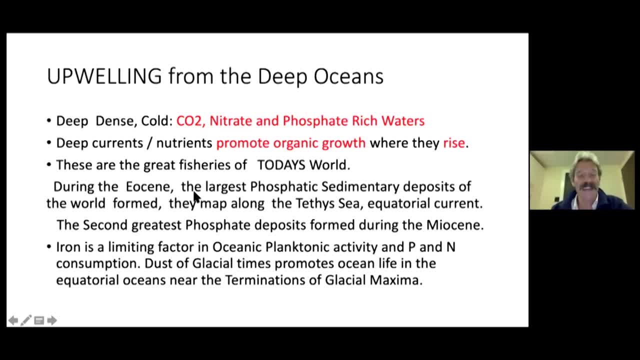 This is something that we And ancient Inca people knew During the Eocene. these large phosphatic sedimentary deposits have been found around the world. I used to work with a fellow who searched for these as a part of a fertilizer business. effectively, 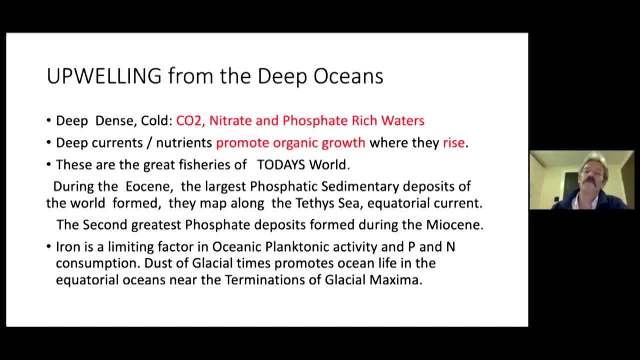 And in those large sedimentary deposits you look for the location of them And they are along that equatorial current, the Tethys Sea equatorial current. They map along that. Secondly, the largest ones of the Miocene also map along a current area which can be shown. 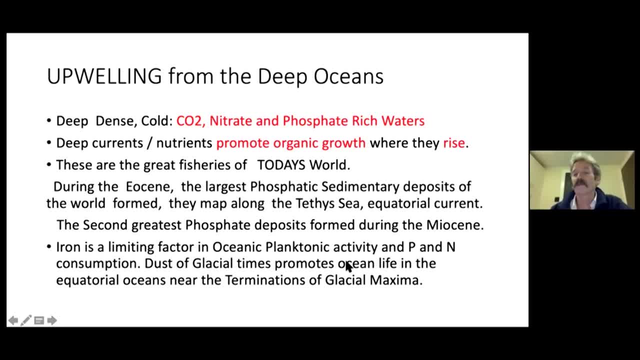 There are other limiting factors to growth within the ocean. The plankton within the ocean will be something we can discuss in part two, And it will be very interesting to see how they bloom in the presence of food. They need the phosphate, They need the nitrogen. 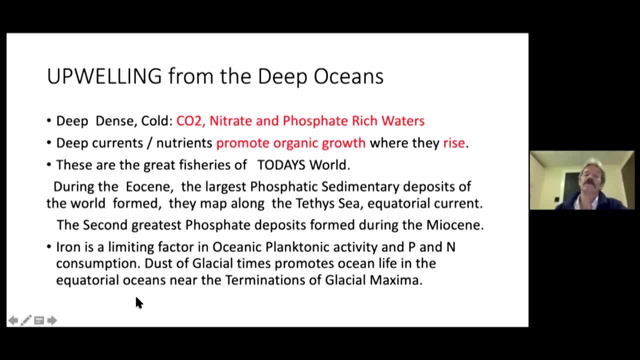 They need the CO2. Because they build the CO2 into part of their structures. So equatorial areas and oceans near terminations of the Maxima is what I'm referring to there, And we'll get into some of that a little later on. right away, 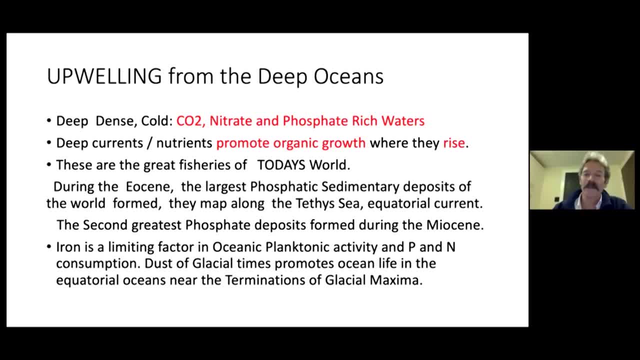 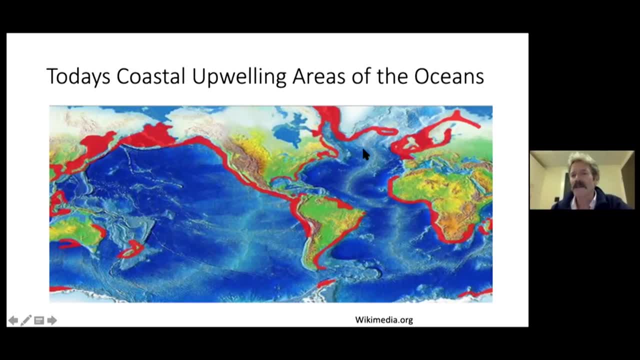 The dust component is something we'll be looking at. This is where upwelling takes place today, These red areas, And you'll probably know that there's a lot going on in the polar seas, Even much more than you would expect to have in these other areas of upwelling. 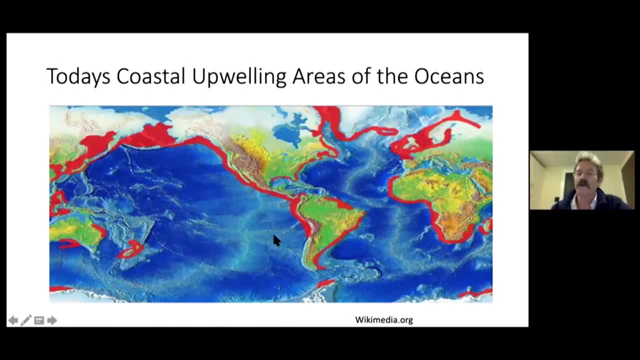 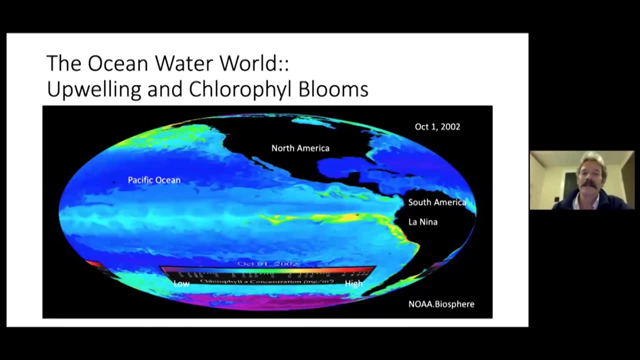 The polar component of that is quite important. Upwelling does take place in this area, And so this representation isn't quite up to date for that. This is a representation of the chlorophyll blooms associated with this planktonic algae that floats on the ocean surface and blooms. 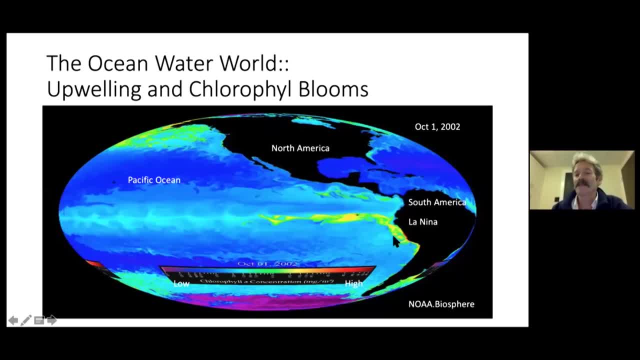 In La Nina times, Creating a tremendous fishery in this portion of the ocean. We also see some portions of it around in this one, properly from space. We're looking at not representation but rather some actual data of the chlorophyll activity at the poles. 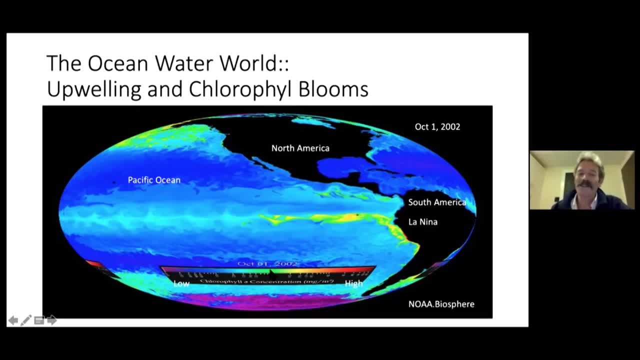 This one. it is obviously going to be a situation where October has to get in place, So this is the October bloom That we often experience. There's more blooming going on through here And, fairly, you know, intense blooming here. 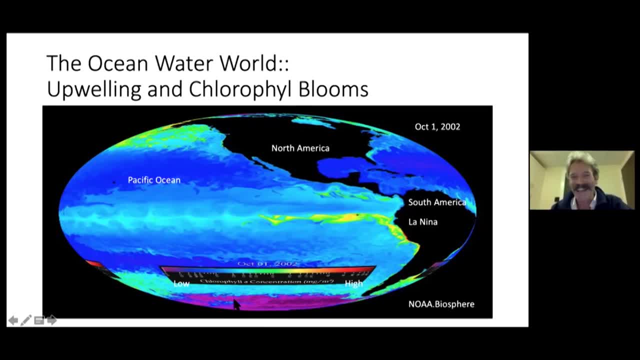 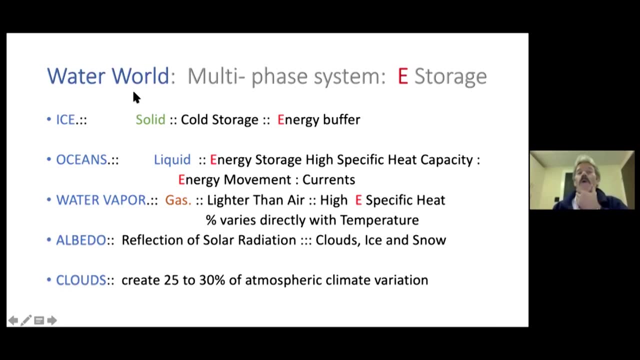 This is the ice, I'm sorry. So in this particular case, we're dealing with some other reflective qualities which NASA is picking up, But what we really want to focus on are those greeny, blue and yellow areas, So it's a water world. 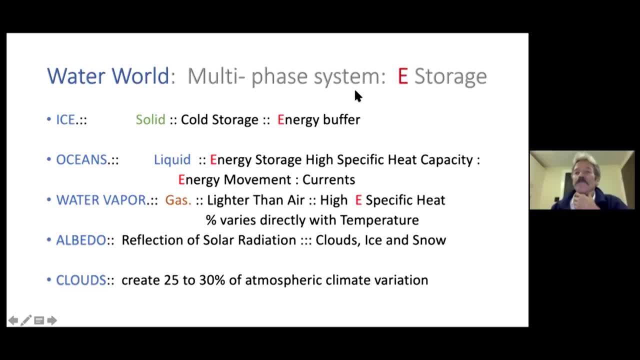 Is what I'm trying to say. In many, many multiple phases, water stores energy. We store it in ice, The solid form. We have cold storage, And it's a great buffer to isolate the poles effectively, to cause their own weather patterns and to make ice ages last until the sun returns to change that. 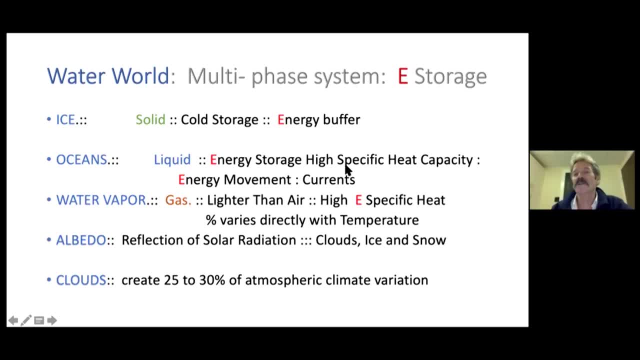 The oceans, That's the blue part, The energy storage there is quite obviously a very high specific heat capacity for water. There is no possibility of a gas like CO2 acting like a liquid here on the earth. It is not possible to store in CO2.. 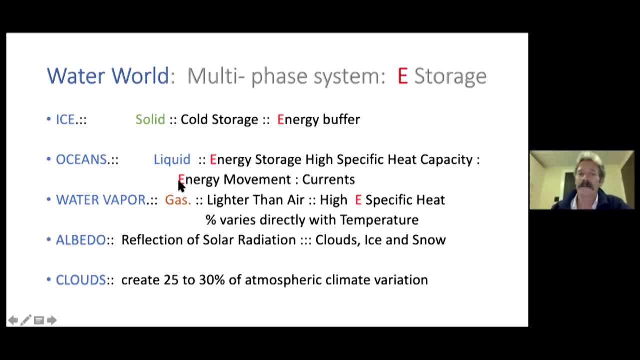 It is only possible that CO2 radiates away its energy, But the current is something we have discussed briefly And it's so important to this liquid transportation of that energy for the period of time that we're dealing with our climate change times. So water vapor. 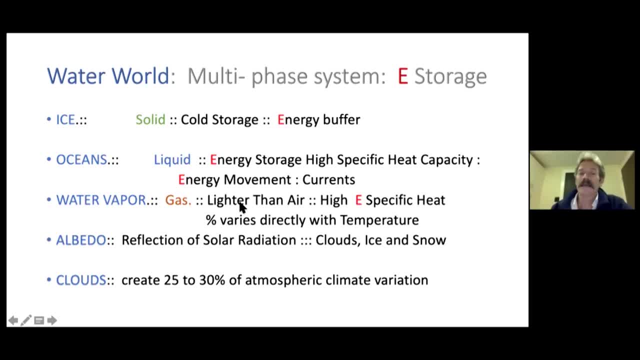 The gas part of this. It's lighter than air, Causes everything to move, Creates high and low pressure systems. It is the source of our weather In every regard, And our climate. It is a very high energy storage area. It has the ability to vary in its concentration directly with the temperature. 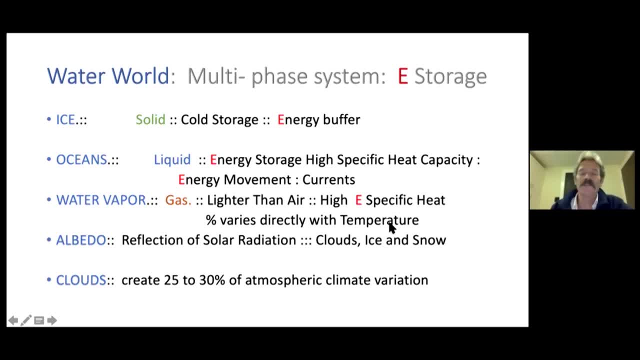 So it's not acting indirectly, It's acting directly with temperature, So it modifies, It, accelerates it immediately By getting into the gas, By modifying the temperature of the oceans, By melting the ice. Albedo is the reflective quality of the earth. 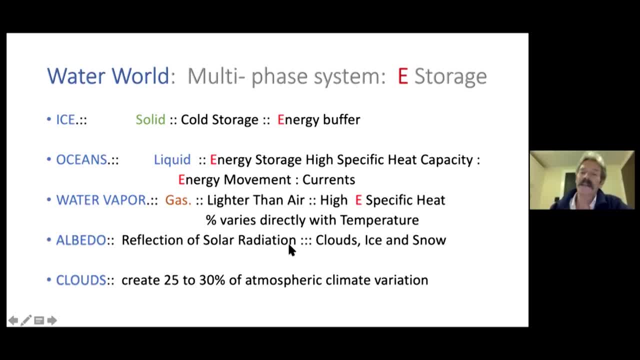 Is it reflective of solar radiations trying to come in and warm it up, Sending it right back out to the cold depths of space? What's going to do that? Clouds are going to do that. Ice and snow will do that. We'll look at albedo fairly briefly now, but more in later discussions. 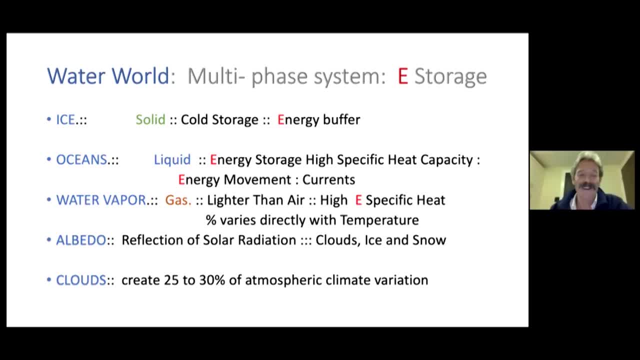 In another slide deck, I'd have to say Clouds. They can create 25 to 30% of the atmospheric variation on earth today And that is something that we will realize, or we should realize, is affecting all of the models that are being developed. 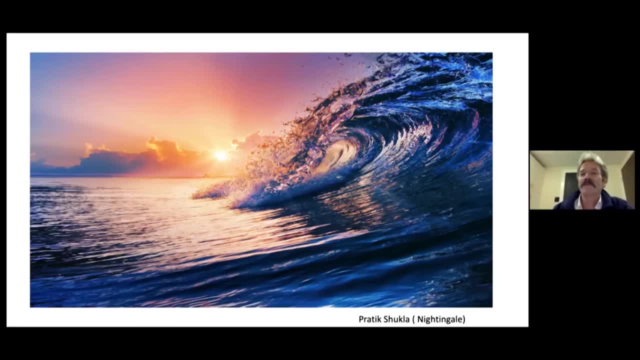 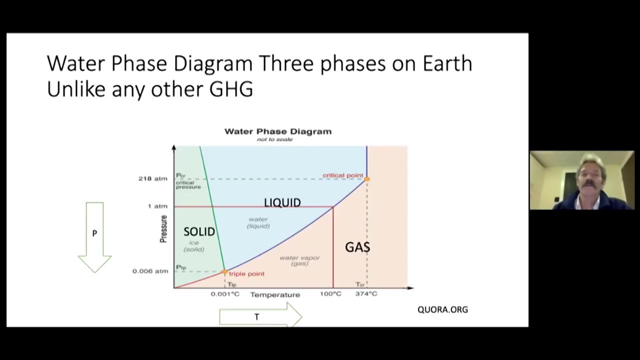 A beautiful picture showing some of the drivers involved in this climate world, And the one that we know very little about is really the ocean, And we need to study it much more, Of course, a phase diagram showing that we can move between these phases of water on the earth. 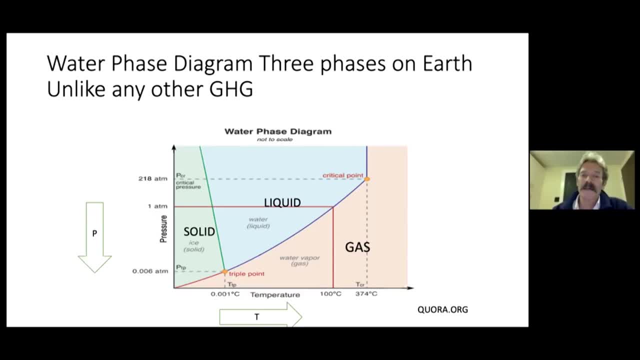 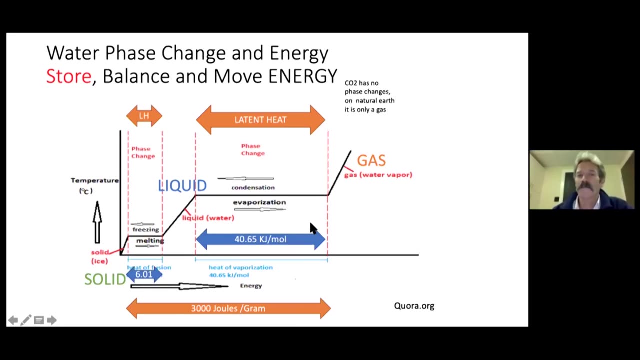 Our earth temperature As pressure changes. As temperature changes, The phase changes And in doing that phase change We move through tremendous jumps called latent heat. That latent heat is the way in which energy is stored Before it changes to a gas. 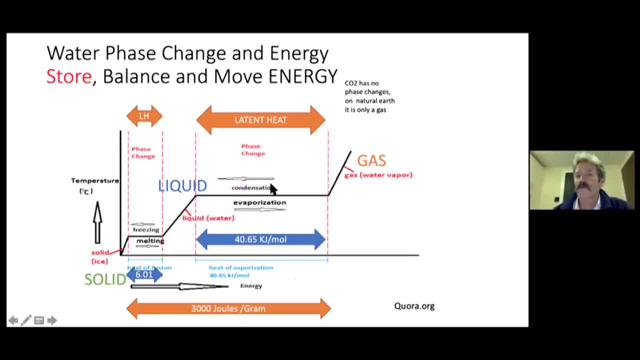 It stores latent heat From the liquid to the gas phase. CO2 has no such phase changes in the natural earth as we have. There is liquid CO2 on the bottom of the ocean Sitting in lakes there- Something else to discuss for another type of talk. 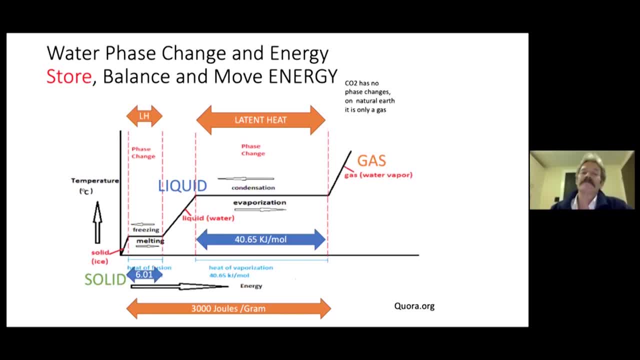 But it doesn't play any part in the surface energy storage system On earth. It radiates its energy- If it has any- And we will talk about some of that- The minor nature of it To the gas And the energy that is stored in the gas. 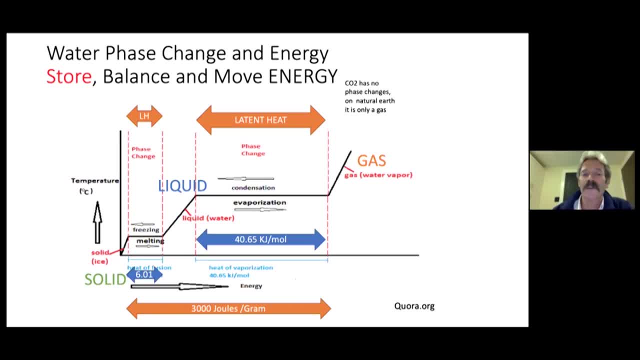 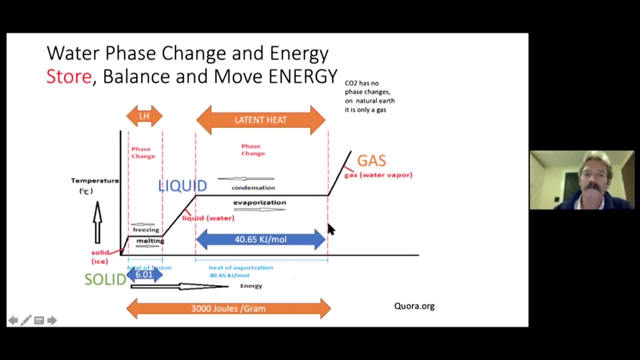 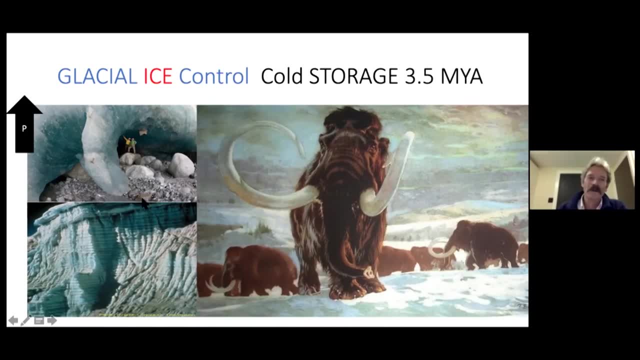 By the gas phase Of water In the atmosphere. The ice component, Let's go at that. Now we are going to move into that ice condition. We are going to talk about the glaciers And the controls And the cold storage concept. 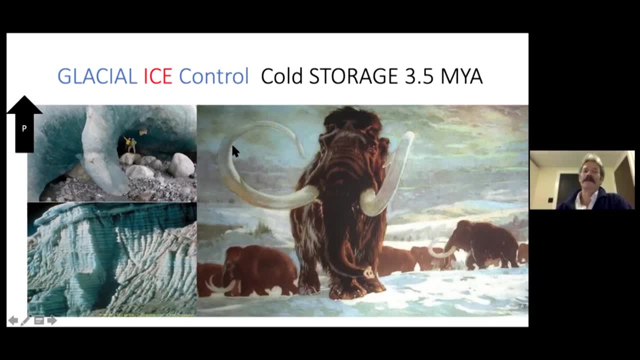 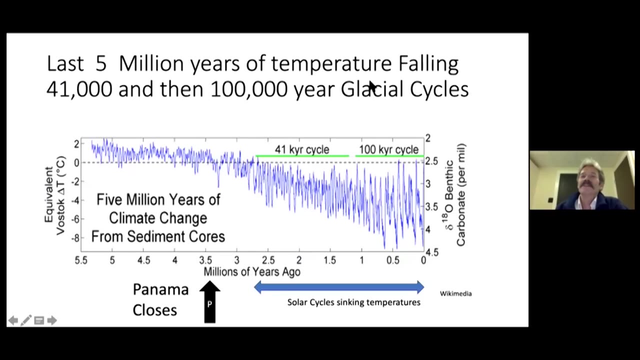 What we are dealing with From about 3, 1 million years ago. Panama closed. We're in the Pleistocene, all right, So there's a picture of the Pleistocene ice and some of the critters. Okay, the last five million years of temperature fall within which we're. 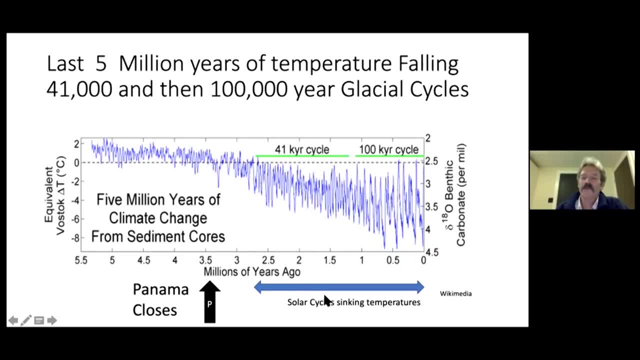 talking about the last three and a half. just now, the solar cycles are showing up in all of this in spades. I'll explain what that means in a minute. Panama has closed, and so we have suddenly changed the ability to move energy around the planet and to store it in the oceans. 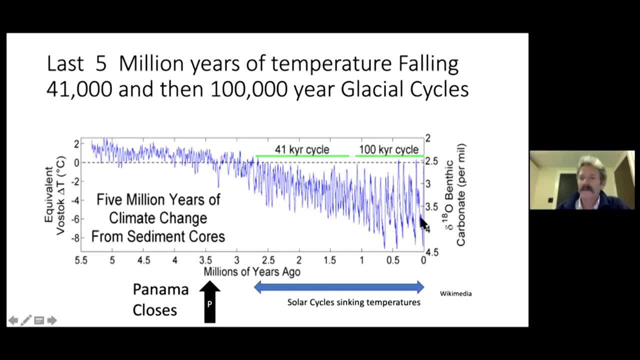 Extremely important. These cycles, these radical things that are happening here, have a periodicity to them. They actually happen every 100,000 years here, or 41,000 years here, and I'll explain that in a minute. I'll explain why that is. The temperature here shown in blue is all from the same. 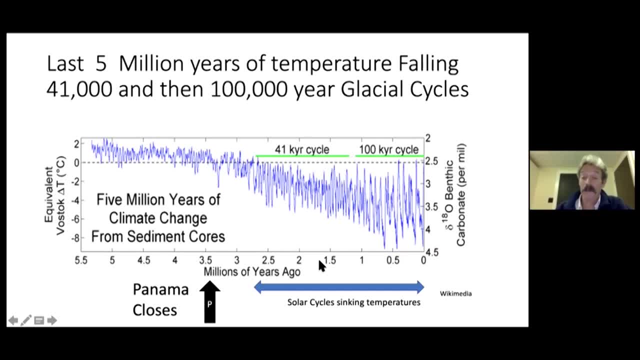 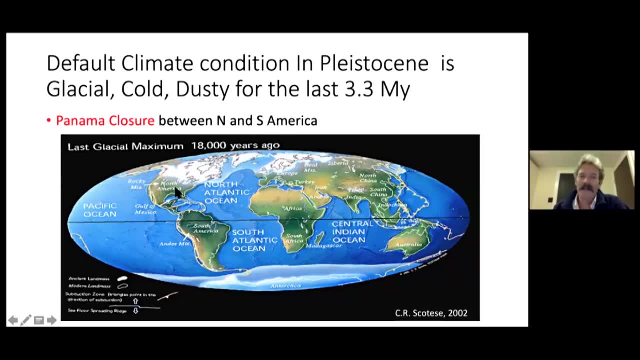 benthic forearms that we were dealing with in the past slides. So, moving forward from there, we go into a look at the Earth at that time, of course, with its large white ice sheets at the top and sea ice, sea ice and large sheets at the bottom of the world as well. so on the South Pole. 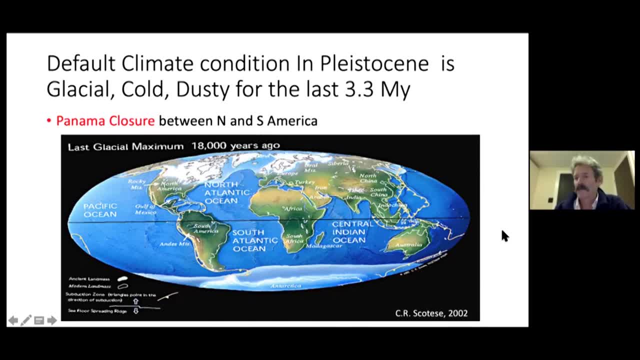 Once again, we're closed. to be able to circulate water and accumulate energy, We have to move it north-south, We have to get by these areas, especially on the southern side. here We'll look at how energy moves today and why such a big change at 3.3 million years ago, when Panama closed. 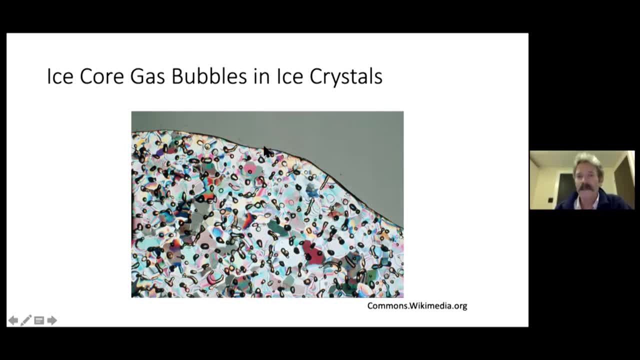 This is ice core. These are the bubbles in the ice core, and these bubbles can be sampled for their content. The other thing that can be sampled in this is its deuterium, for the portion of it that's an isotope of water, the hydrogen from it. So all of these isotopes within. 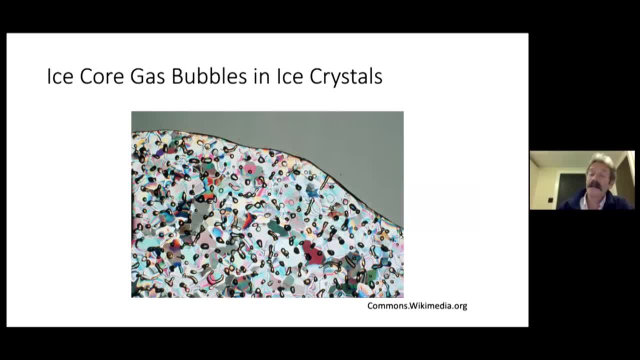 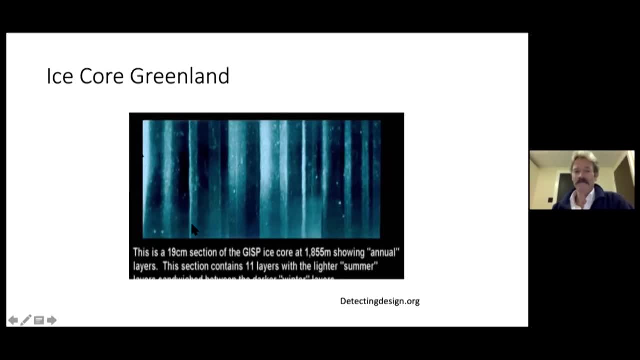 it start to tell us quite a story within ice, the same way it was within those organisms. So this is clean ice core from Greenland. This section shows yearly cycles- Light and dark- And the light is the summer cycle, The dark is the winter cycle, I guess. 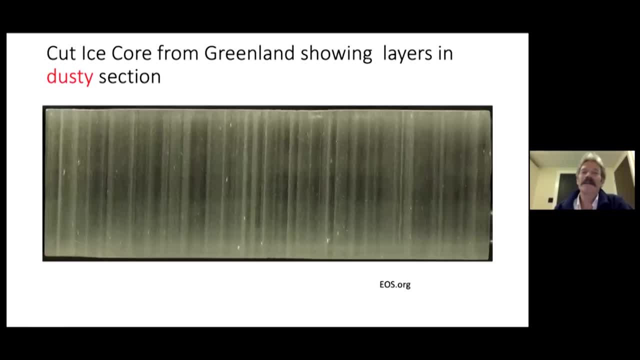 that's appropriate anyway. So what happened here? The dust moved in. This is something that hadn't really been realized very much in the ice core. It was sort of a secondary thought. Now I think it's much more important to the people studying it. They were much more interested in those isotopes. 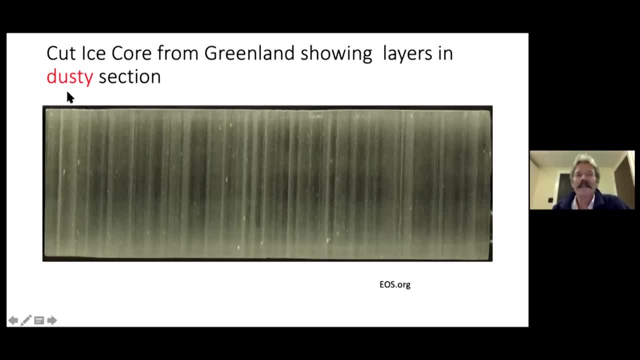 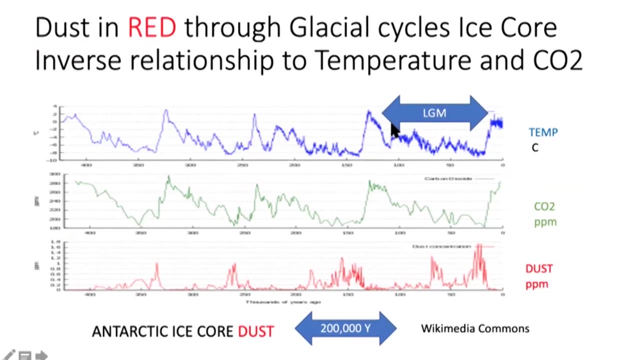 But what we? and in the bubbles themselves. but let's look at this dusty section. All of this is accumulated through a very interesting period of time. This is a picture of those temperature isotopes. once again, Remember them. This is from the 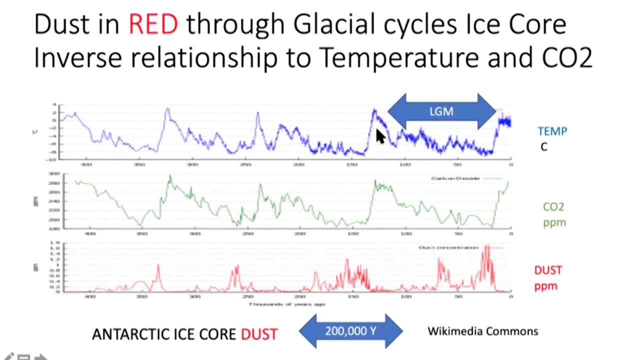 isotopic signature of the water and of the gas within the bubbles. So what we're dealing here with is something we're going to call the isotope of the water, And this is a picture of the LGM, the last glacial maximum That happened over about 100,000 year period, these being 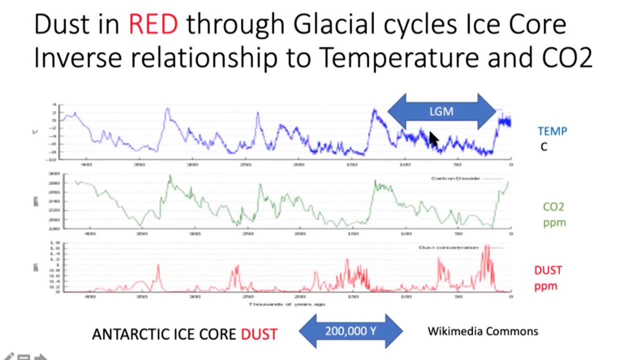 50 and 100,000 years here on the bottom between peaks. these peaks, These glacial periods roughly last 100,000 years of temperature drop before we radically move up into a peak. We'll get into those radical moves fairly quickly. We got into a lucky little piece of. 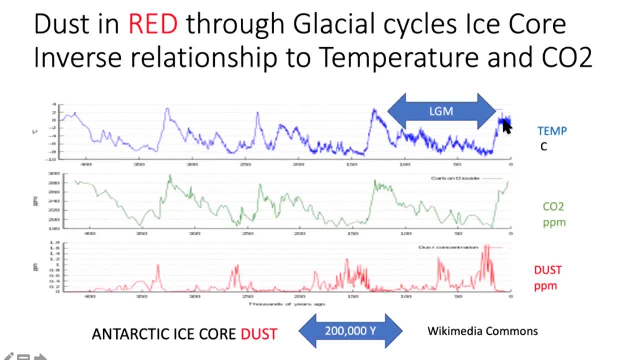 territory here, didn't we? We landed on a nice, warm island, away from the glaciation. What has happened, of course, is that CO2 has followed suit, related to what's happening coming out of the ocean. We'll talk about that a little bit later on. Now, what's this? This is the dust. 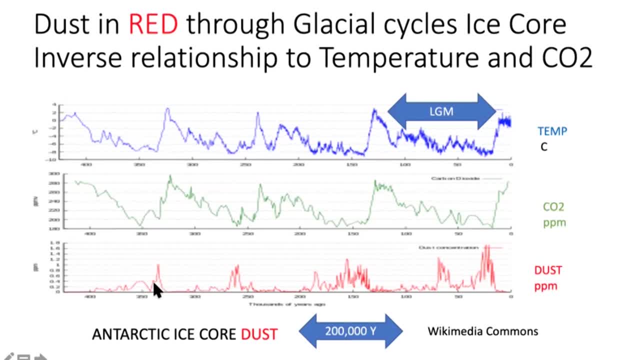 Something that should have been recorded originally, seems to have a regular periodicity to it And, a matter of fact, it seems to be coincident with the lows in CO2 and temperature. Okay, what that is? what is that? That is dust that accumulated in this ice. 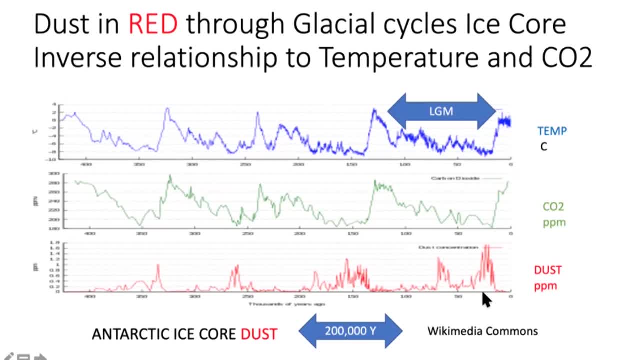 in Antarctica because of dust storms in the rest of the world. Why dusty, Oh my gosh. Well, when we're in a glaciation, the depth of a glaciation like here, the big maximum thickness of ice is on. The water levels have fallen around the world. 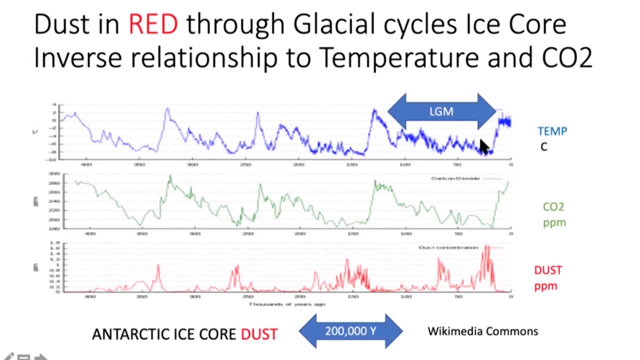 We've had 120 to 140 meters of change there. We've exposed shelf edges of the continents. We have also created great deserts, Deserts barren of life. trees, vegetation, Vegetation doesn't survive very well. when you drive the CO2 to the bottom of the system here and you cool everything. 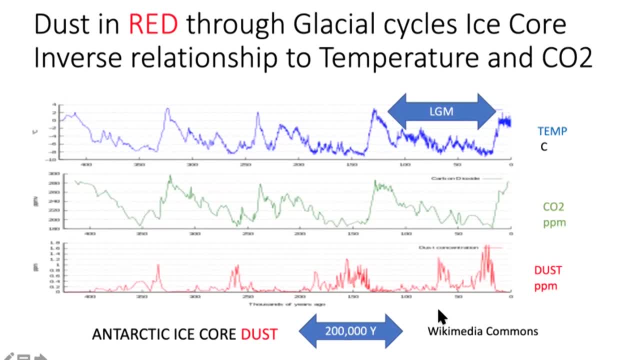 down. What we ended up with was dust bowls blowing around and being recorded for us in time, even at the South Pole. So that means that there were some tremendous movements of dust in other portions of the world at that time. Dust strongly correlates and is upward turning. 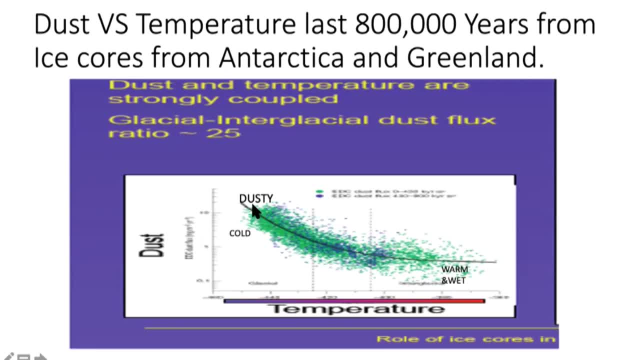 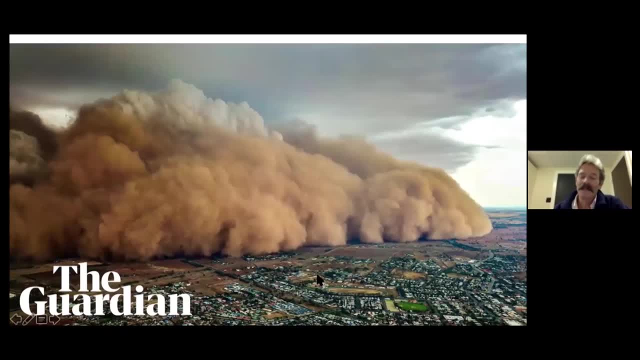 in an asymptotic fashion with cold, Warm and wet, no problem Dust today in Australia. These kinds of big dust storms go across the Sahara today, accumulating and blowing up into the upper atmosphere. These are well known and can be mapped, of course, by satellite, And there's very good satellite representation of that. 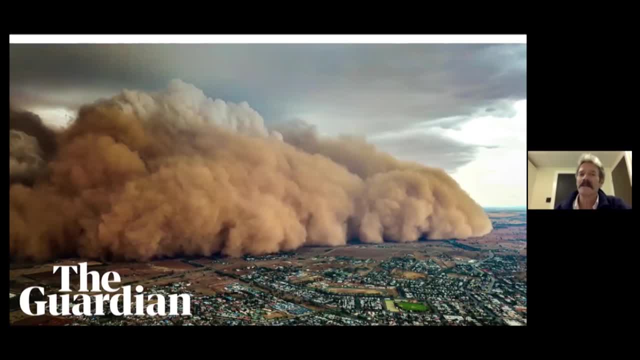 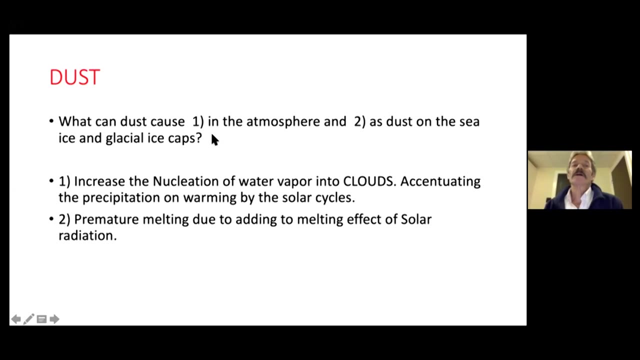 if you want to go into it and see what happens with some of these major dust storms that settle The heavier fraction, the lighter fraction, You can see some of the stuff boiling up high. That's going to go stratospheric. What caused it in the atmosphere? It was also going to spread over the ice caps. We'll deal. 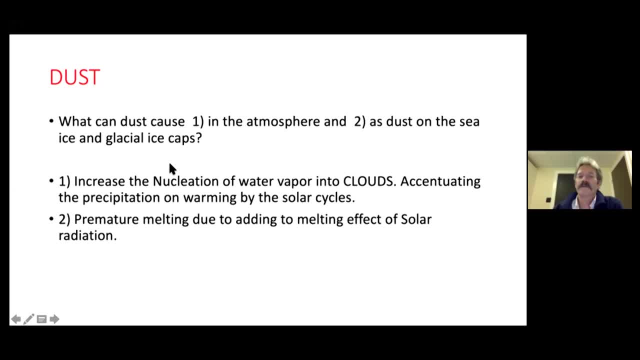 with that, It has an effect on water vapor in that nucleation can take place in clouds And cloud formation, as we mentioned, is extremely important to regulation of temperature and reflection albedo. It accentuates precipitation And so therefore this could. 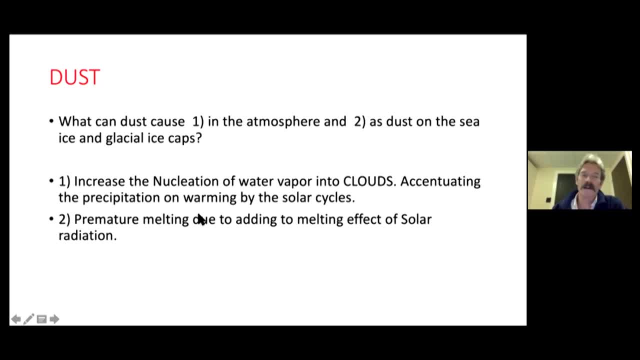 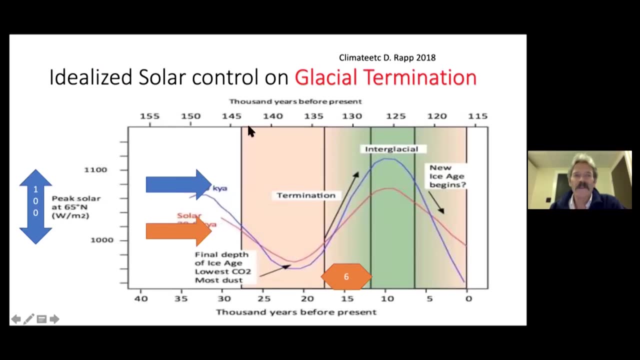 have been a very changeable time with a lot of dust involved. We want to get into what it does to the solar radiation and albedo effects. Let's take an ideal idea: Glacial termination now. So here they are, the hundreds of thousands of years across here. 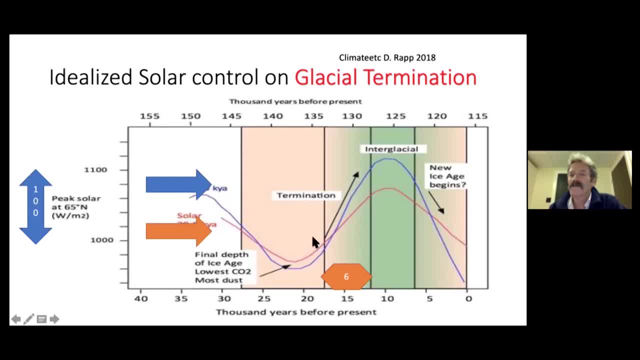 from present. This is the glaciation, just before we ended up getting into the last glacial maximum. This is something that would be called the Eemian. So during the Eemian, we look at all of these characteristics and we see that the solar 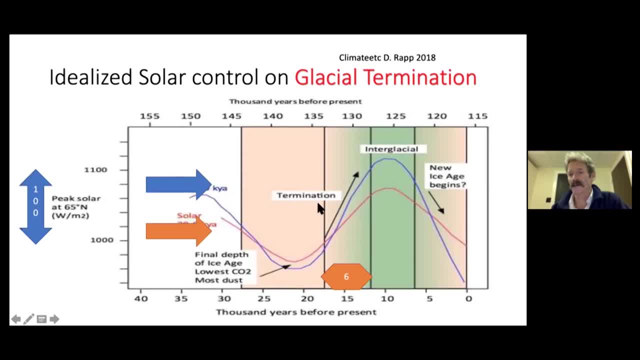 cycles were coming along and overlapping. during this period of time, Where they crossed and overlapped and complemented each other, we got the termination to the interglacial period. This only took a period of 6,000 years, whereas it took us 100,000 years to build that ice. 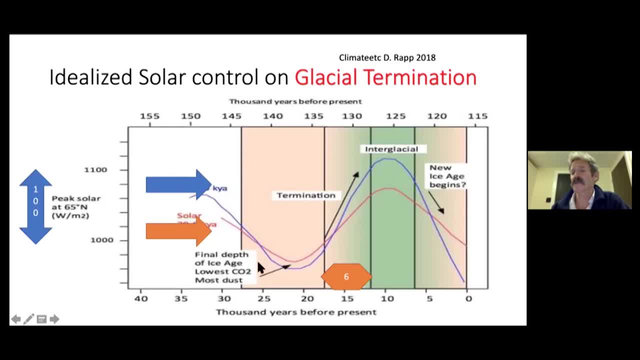 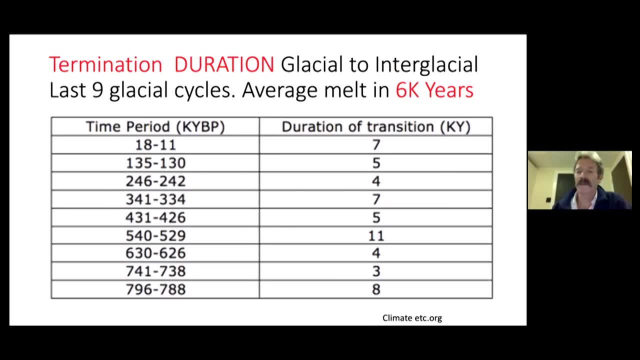 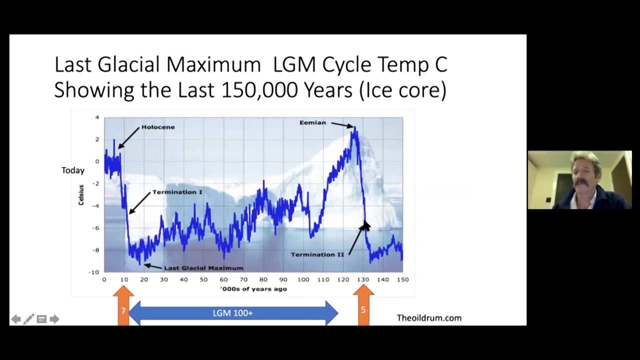 CO2 is at its bottom, its lowest here, Dust is at its greatest. Those are the averages for the last nine glacial cycles that we can map within the ice, So each one of them varies, but the average for them is the sixth which I was showing. This is the Eemian here, its termination from the base of. 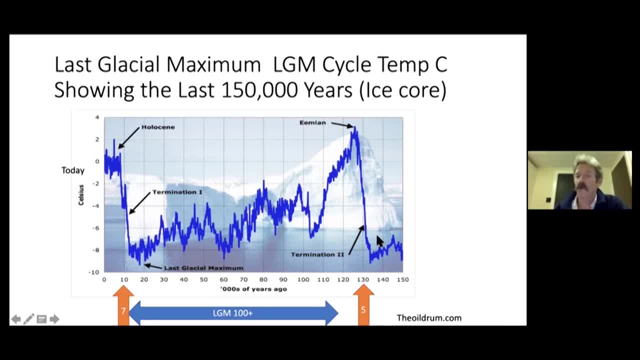 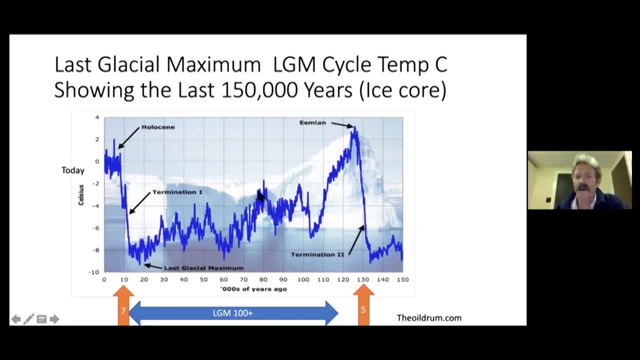 Gradually falling off, trying to recover, trying to recover, trying to recover. Well, look at these recoveries. Why didn't it make it back? The solar cycle system wasn't strong enough to do it, and perhaps the dust which collects at the very terminal portion of it wasn't great enough on. 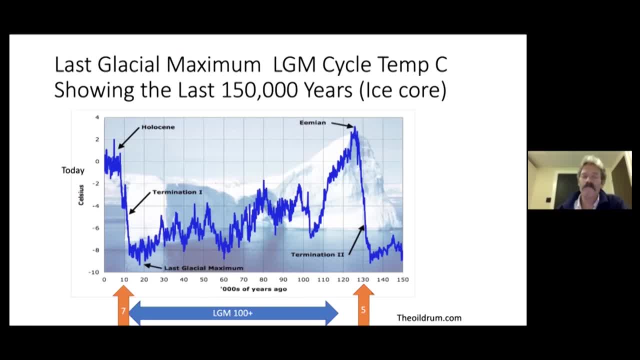 the ice, to cause it, to help it melt out. The last glacial maximum is shown here and we are living in that little island, A little island up here, once again, of warmth, Longer than, but lower temperature than, the Eemian. 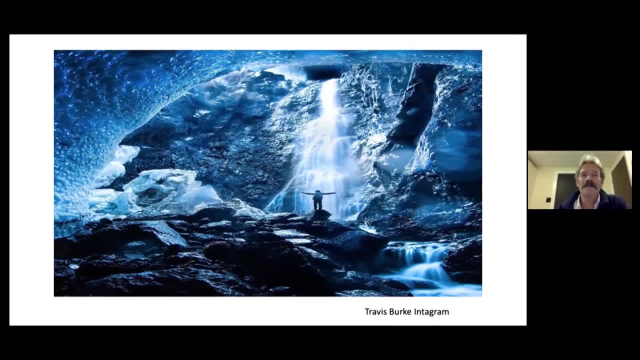 A bit of a rest for your eyes from all the graphs just to study the beauty of the melt out here. So a subglacial picture, a wonderful picture, with somebody who's really thankful that there's that. the ice is leaving as far as I'm concerned. 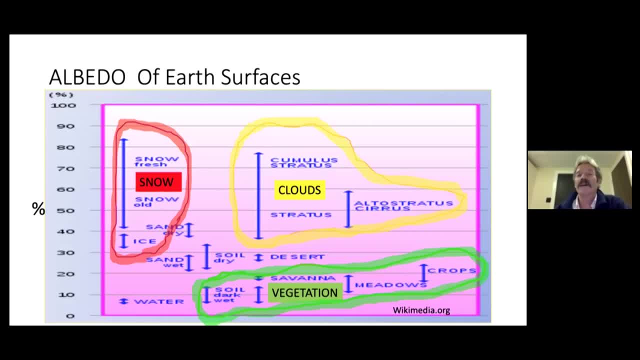 Now, let me take you back here, to kind of see what this is all about. In the form of a youtuberswitch or a developer's zoom in, it actually's kind of been something you might see simultaneously on campus. Which, you know, it's a fun ring dance on Earth, because, for mostтha � s, it's a 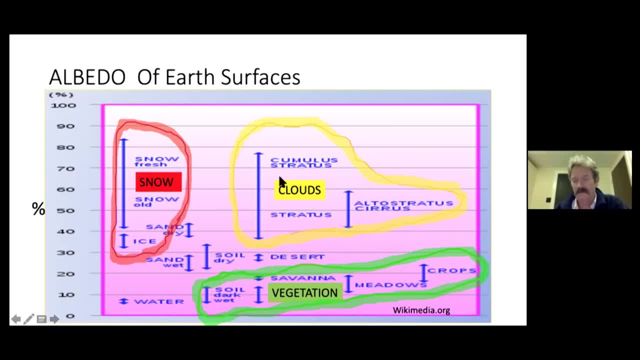 1964, or 알고 thing On earth as well. There's a lot of legislation is happening. It's kind of interesting why we need to look back at that year since then, right, Because in fact that's something that we kind of undergo, you know, Wow. 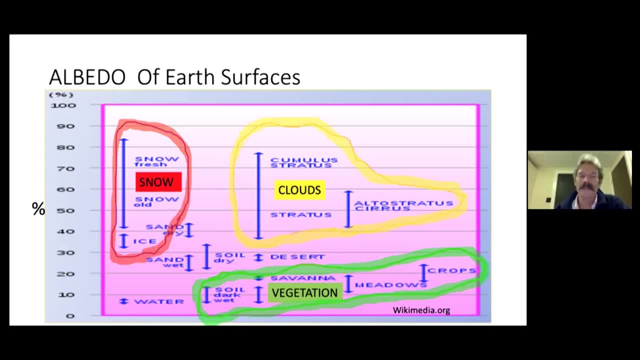 nationalism's been jumping in for quite a bit. let's take a look at that. So onSLock, there you have the larger unemployment attempt. You see the rent that's compared to a quarter wall being built in over the year, supposed to be. 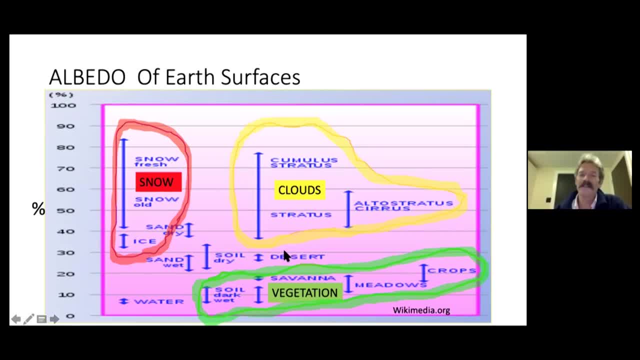 We've got deserts which actually register as something more reflective than vegetation: dark soils and water. You remember the water. We're trying to absorb energy into the water. We can do that. All the oceans, 70% of the earth covered by that water is absorbing energy because it's not getting reflected away. 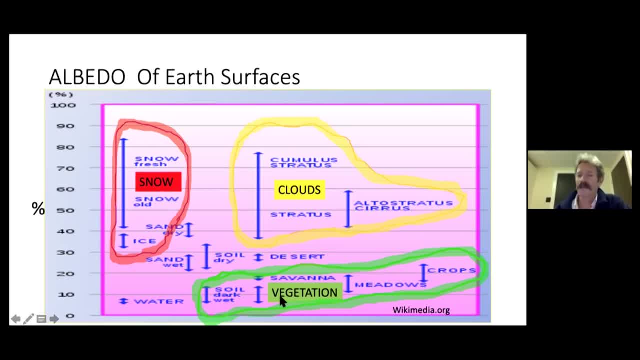 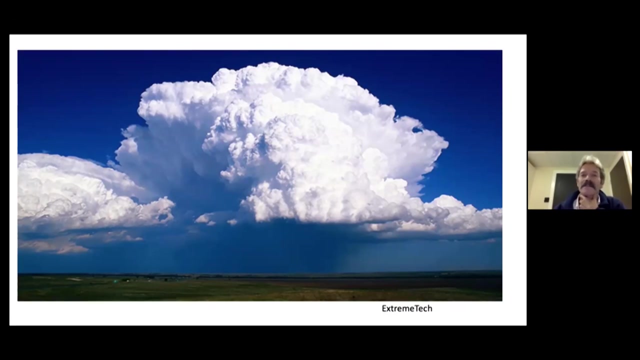 The vegetation is absorbing as well And that's helping us. when it's a very vegetated time, when it's wet and warm, Vegetation thrives. Vegetation dies in the glacial periods. Some pictures of that albedo Great blankets of this. 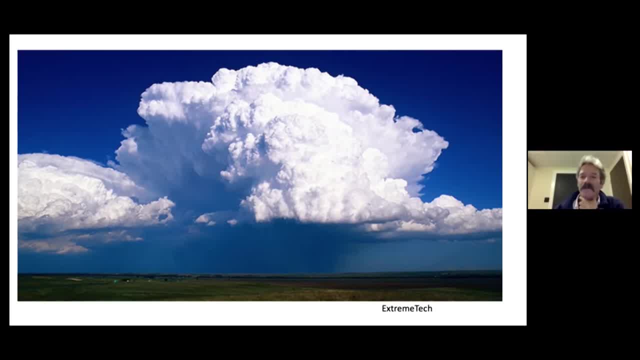 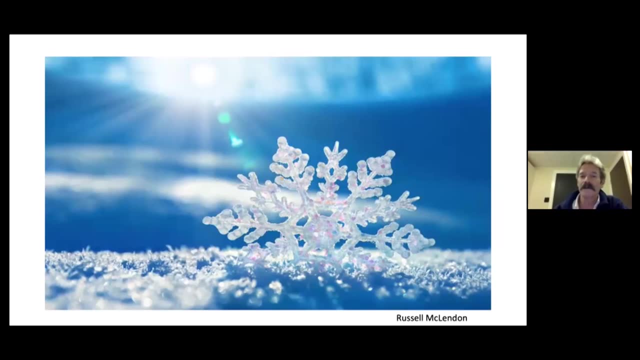 Even minor areas, of course, of cloud carver strongly affect the, as you know what happens Below them. we see tremendous contrast in energy and energy storage as a result of the influence of clouds- Snow itself- Just a pretty picture of that one with the sun involved. 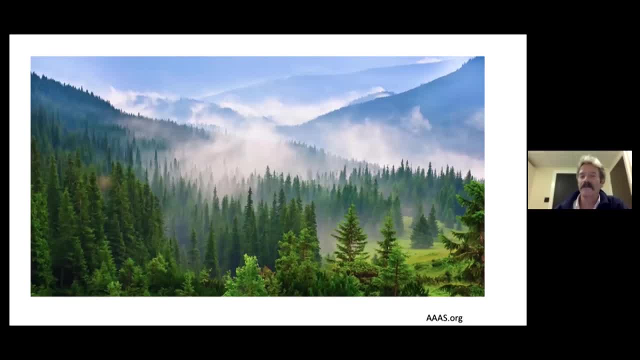 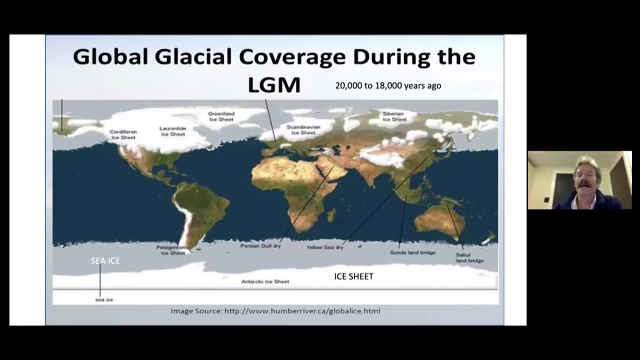 The forests here breathing back to the atmosphere, Absorbing a significant amount of the incident- solar radiation, of course. What did it look like in that last glacial maximum 20,000 to 18,000 years ago? we had some very high latitude deserts all through Siberia and into the Caspian Sea area. here they are pretty well coincident with what you're dealing with here even today, which is the large Sahara desert. 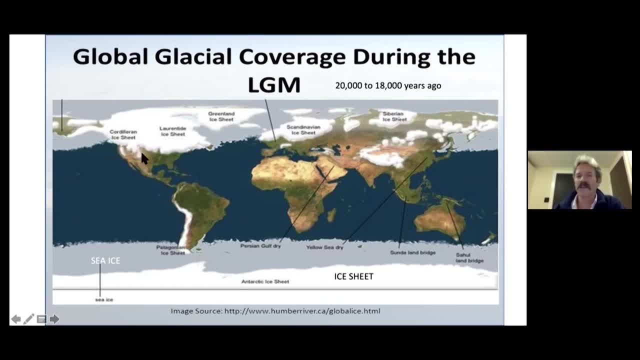 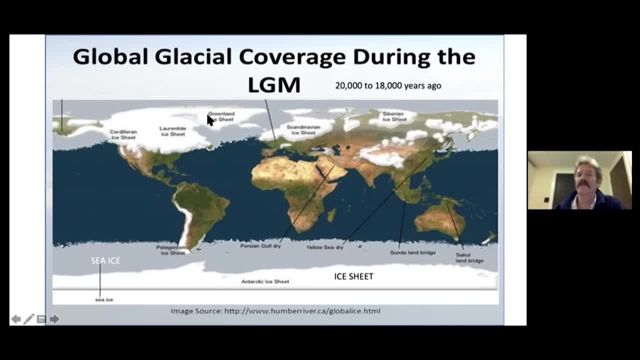 We have exposure of similar nature. These cordillera ice sheets are very important. Another thing I want to draw to your attention, which wasn't as visible in the last representation, was these ice zones here, sea ice. These cordillera ice sheets are very important. 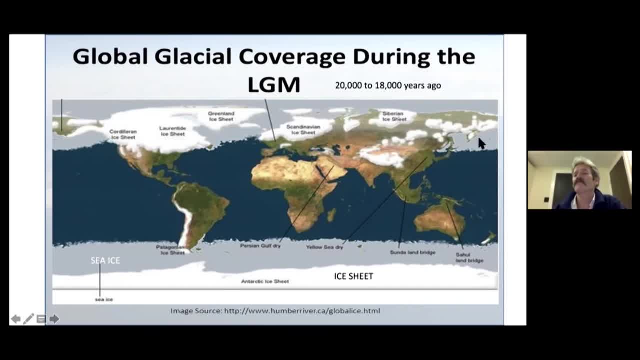 Sea ice would have been present over much of this, restricting the wind getting to the water, the ability to move energy into and out of the water. Sea ice would have been present over much of this: restricting the wind getting to the water, the ability to move energy into and out of the water. 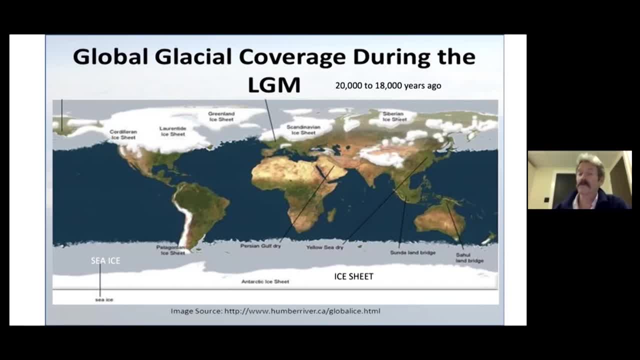 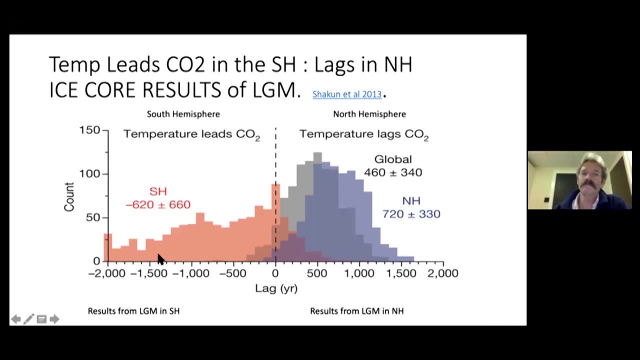 It is also the first thing to reflect on melt off in a deglaciation and would have gotten covered by a lot of dust. What we could do is melt that back, first very radically, and then attack the ice sheets. Does CO2 lead temperature or lag temperature- A debate that people, including this fellow- 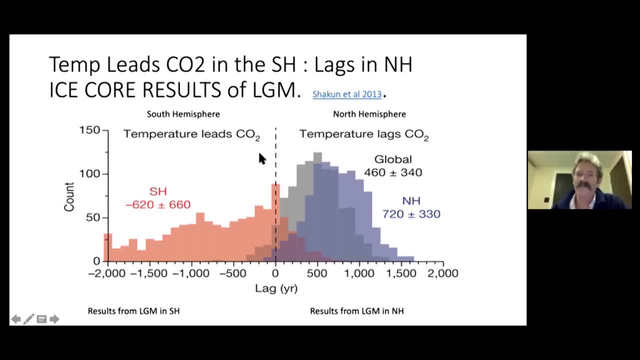 wanted to try to resolve. They hasn't resolved it. He found that in the southern hemisphere temperature leads CO2.. In the northern hemisphere temperature lags CO2.. So the CO2 signal they were picking up in the ice core and what he's reporting on here. 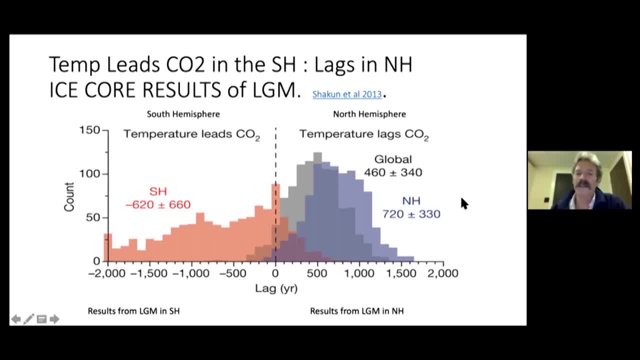 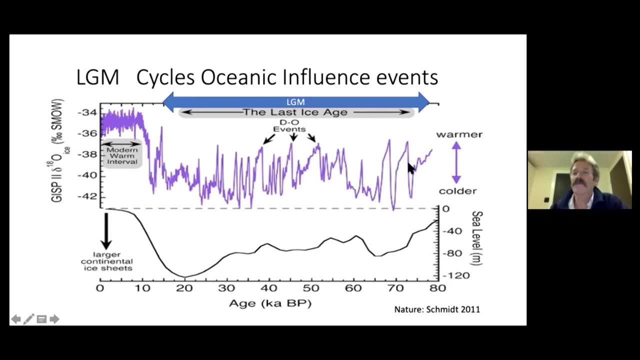 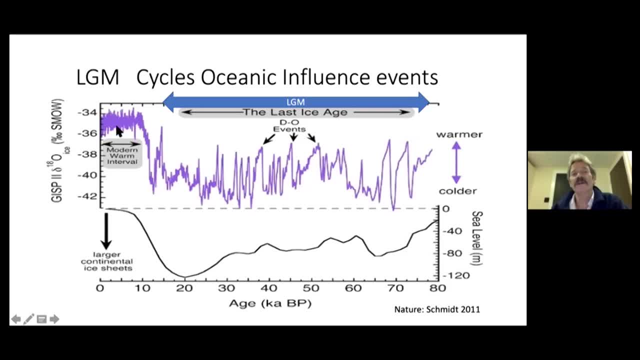 at maximum glaciation. These are the temperature fluctuations. This is where we are in our modern warm period. This is the Holocene and this is the little last glacial maximum. sorry, The last glacial maximum has spikes within it and those spikes are opportunities for the sun to 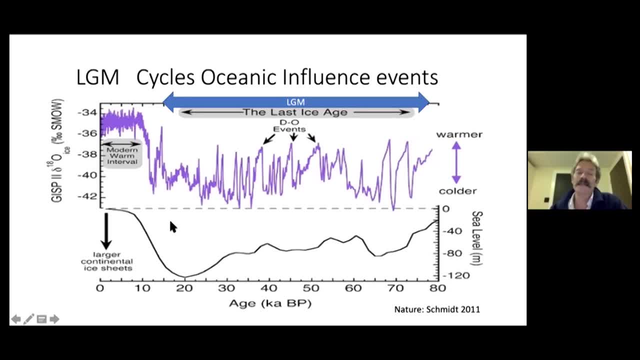 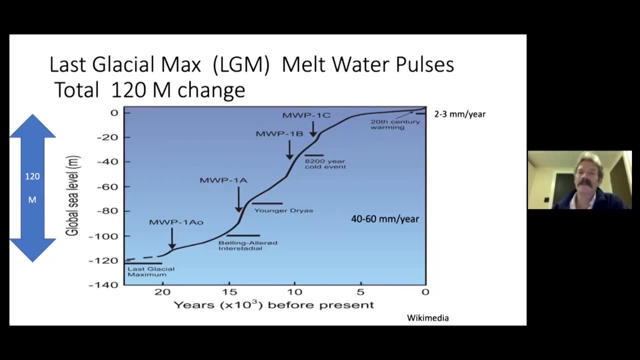 warm the earth enough to get us out, but not quite enough. That's why the dust and the accumulation here is going to have to be of much greater interest in the future. The sea level pulsed. It is on this small pulse back up here, but it moved in great chunks through this period of. 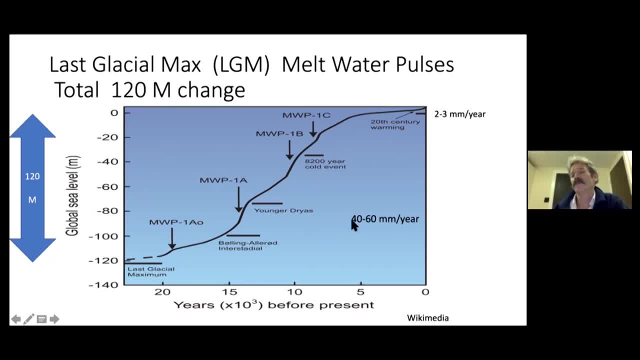 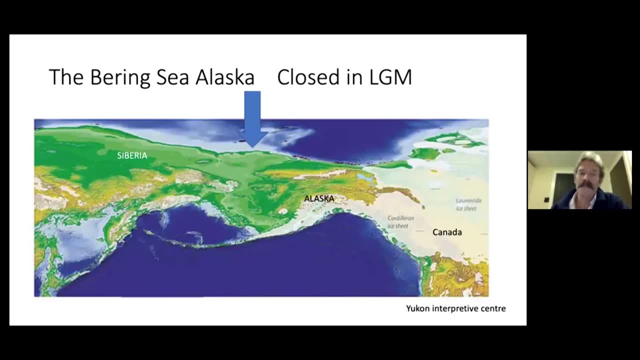 recovery from the last glacial maximum. It moved up and up and up at 40 to 60 millimeters per year. When the sea level falls, you close some of the Arctic. because of the Bering Strait, Sea level fall in a very shallow area here in the Bering Strait allows this to be completely isolated from the 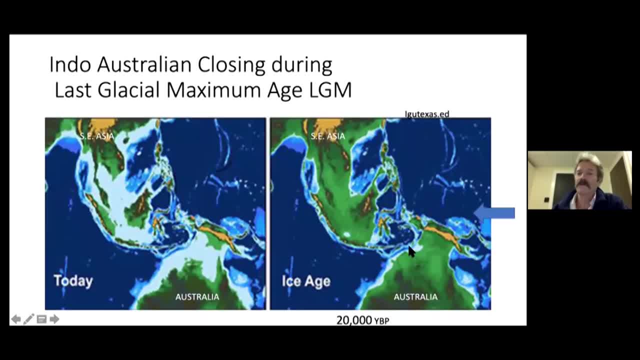 Pacific Ocean. Also, when you drop sea level, you affect the Australia-Asian area, the Philippine Ocean area, and you can see that the sea level falls in a very shallow area here in the Bering Strait. When you drop the sea level, you can see that the sea level falls in a very shallow area here in the 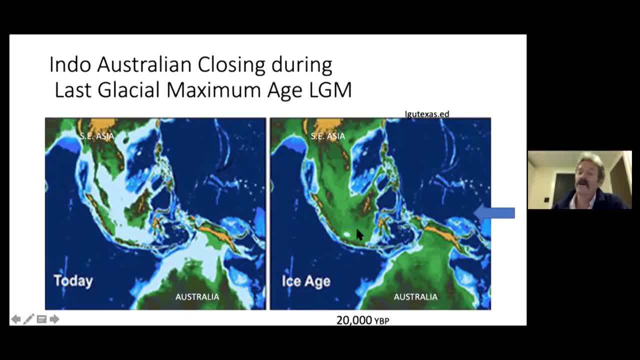 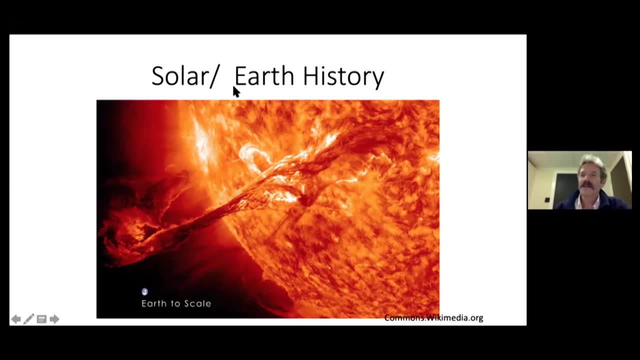 Philippines, the New Guinea area, here all essentially closing off or shutting down circulation which, if it were, through going through those periods of times, might be able to get us out of glaciations. The solar history and earth history. The next topic, the most 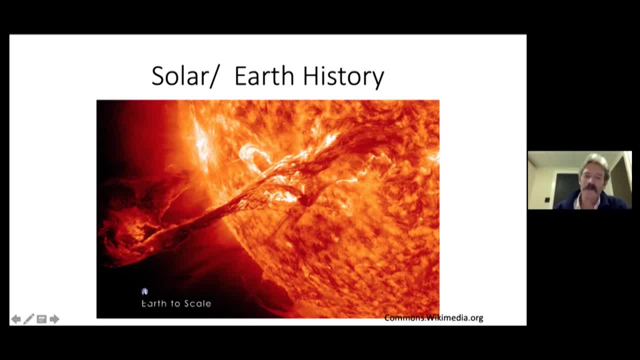 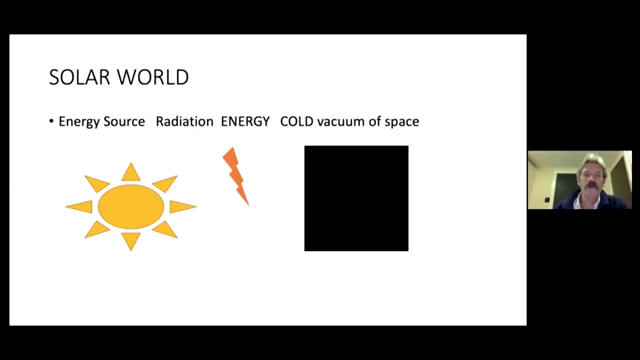 important one from earth's point of view. small little earth over here to scale, showing you one great example of what's going on in the solar system: great big sunspot, active magnetic flare. The solar world acts through radiation to get its energy to the earth through the cold vacuum of space. Those 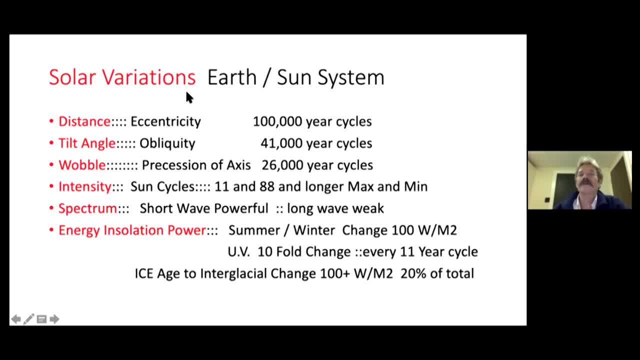 variations in the Sun that are most important are dealt with here in the Earth-Sun system. The distance, how far away from the Sun are we? The eccentricity, we'll call it, The tilt angle of the earth itself on its axis, the obliquity. 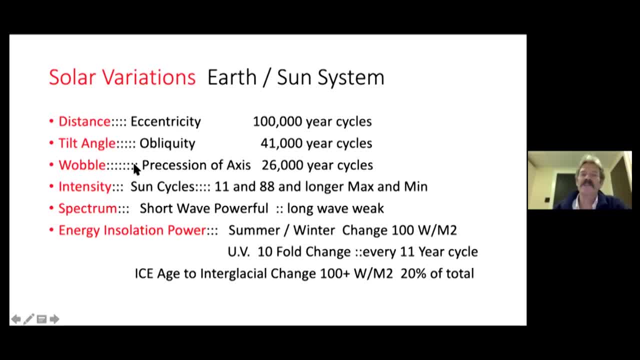 The wobble, the procession of it like a top through time. This is the period of time that each one of these shows up in something called the Milankovitch cycles. This was a construct, a theory in a sense, before demonstrated in a lot of data now. 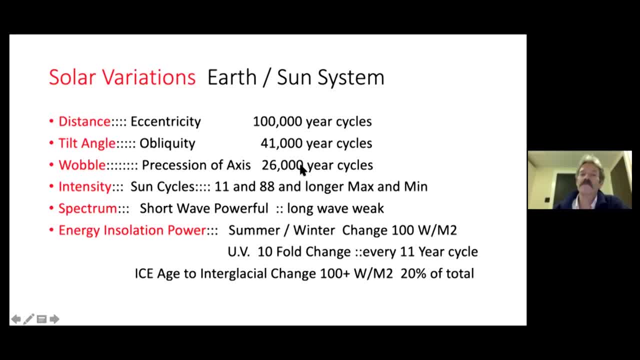 Including the data we just went through at the beginning of this program and this talk, So these cycles can be reproduced in the data and can be shown to be part of the theory. This is how the world progresses is by putting a theory together and then finding it in the evidence. It's a little bit like Einstein. 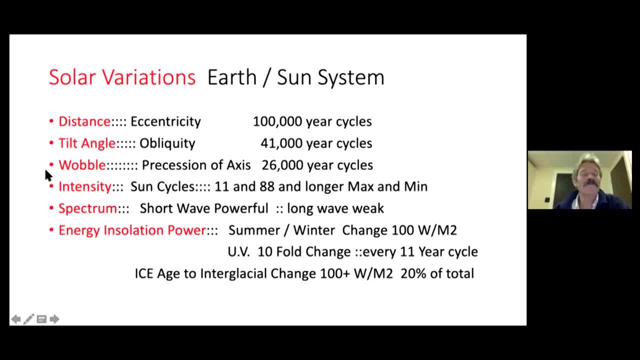 bending the solar light from behind the Sun and proving that his theory of relativity was correct. It's a theory until it's proven. I think we need to remember that in everything we are doing as well. We need to continue to have that evidence-based component to. 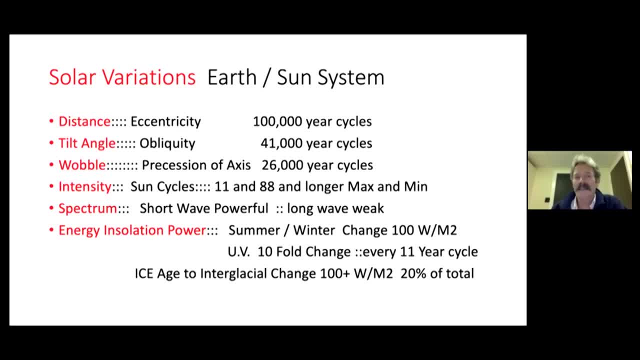 it. Intensity of the Sun varies. That intensity we will deal with on the 11 year cycle. We won't address the 88 year cycle. but there are longer ones which will also allude to in this particular portion In a second talk. we will try to look at those in. 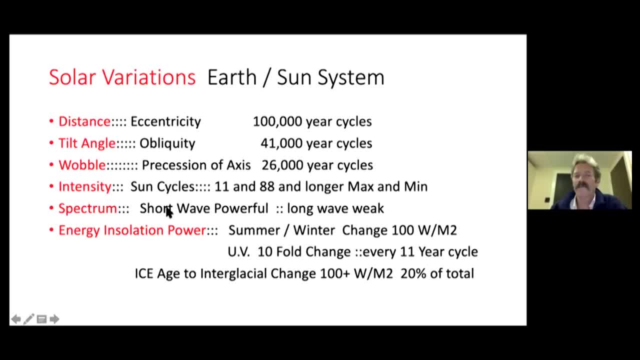 more detail. The spectrum of the Sun does change from the very short wave powerful waves to long wave weak waves. That is an important component of how we address energy flow from the Sun and what we receive, what we don't receive through our atmosphere, The energy. 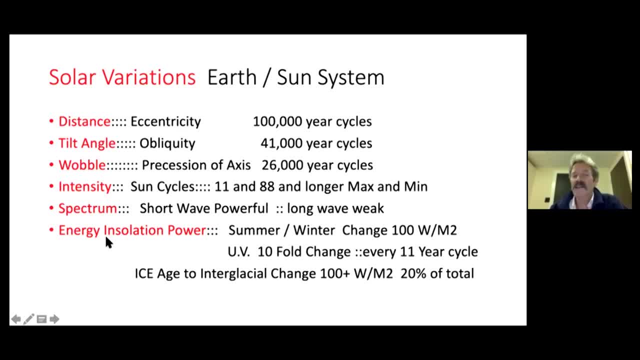 itself is insulation, we are calling it. its power is measured in watts per meter squared, And between summer and winter we experienced that. now We have experienced a change of 100 watts per meter squared. So that gives you a sort of a layman's view of exactly what's. 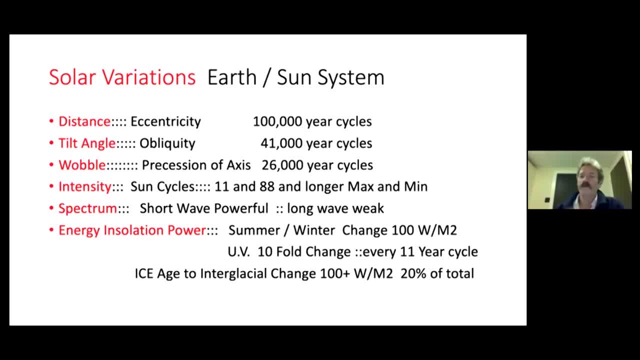 happening here in terms of change into and out of glacial periods and that kind of thing too. It was on a lot of those former graphs and it would be important if you review this again: The ice ages to interglacial which I was showing on those only 100,000 years of the insolation, the energy output of the sun- about a 20% movement in that, based on what happens to these factors and whether they all work together or work apart. 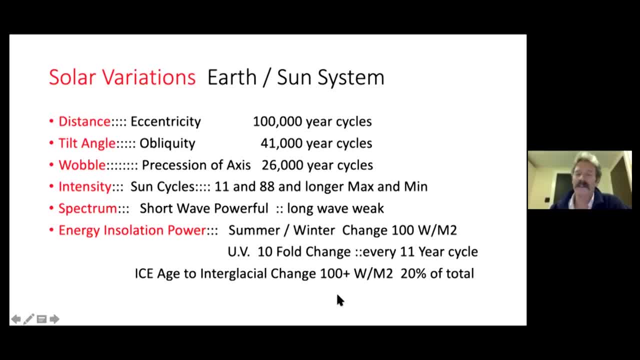 We couldn't always recover from a glacial event. It kept sinking deeper and deeper into it, And that is something that clearly shows up today. We can't get out of these very quickly. We're getting into 100,000 year cycles, not 41,000 year cycles. It's lasting longer. 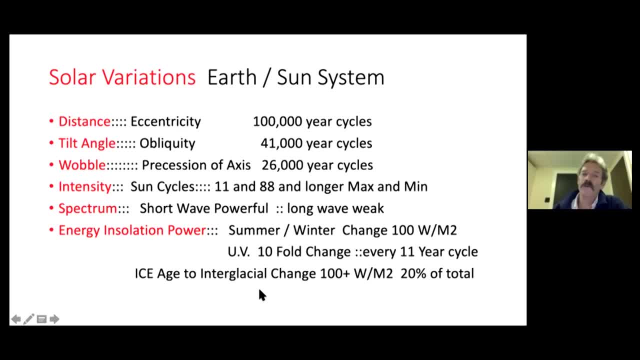 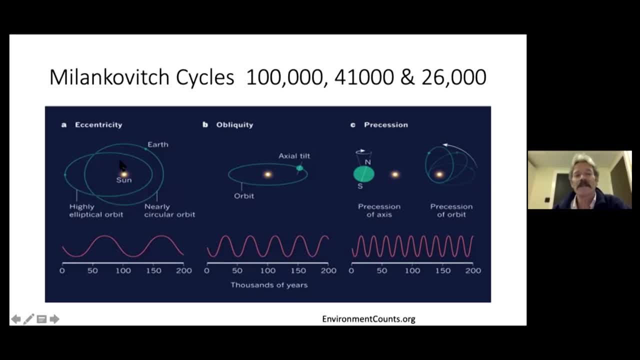 We're not getting out of those glaciations as fast as we might have at one point. This is that story- the Milankovitch cycles: 100,000.. 41,000,, 26,000.. This is the eccentricity: moving from a circular orbit to a whole optical elliptical orbit, an oval. 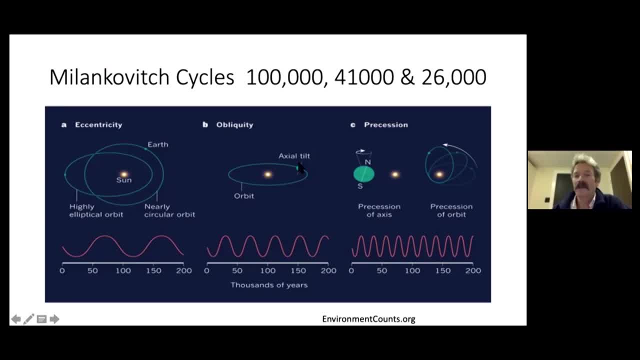 This is the axial tilt, demonstrated by the small axis. here It changes, And this is the periodicity of its change, All very well documented: 100,000 years, This is 41,000 years, And now we're going to go into the 20%. 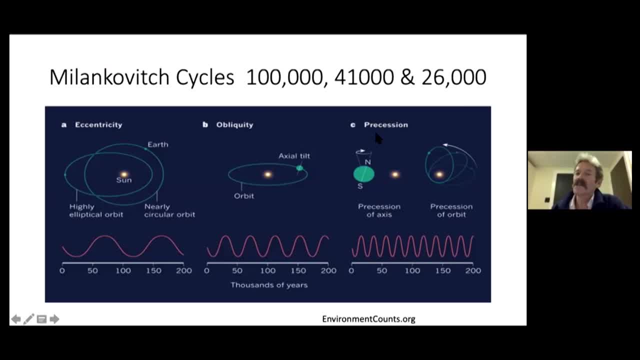 26,000 year cycles. That is happening because of precession. The pole is not always pointing to the pole star. It moves around the sky looking and pointing at a whole series of other stars within the universe, within the Milky Way. 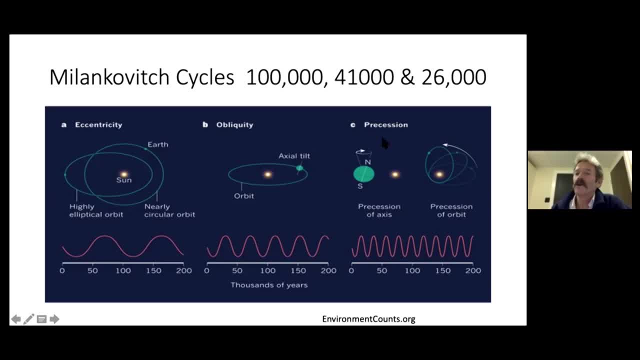 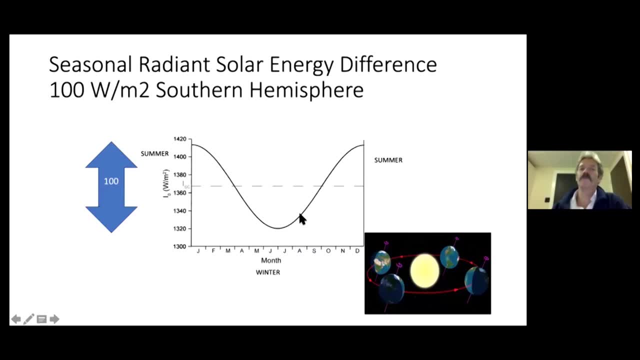 And so, as a result, we have something we call precession, like a top will precess. So those are the three main ones. There's another one, but we won't even go into that. It's more to do with planets and how Jupiter influences the sun and also the earth. 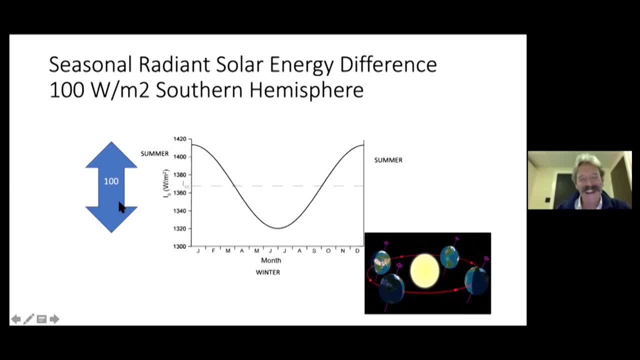 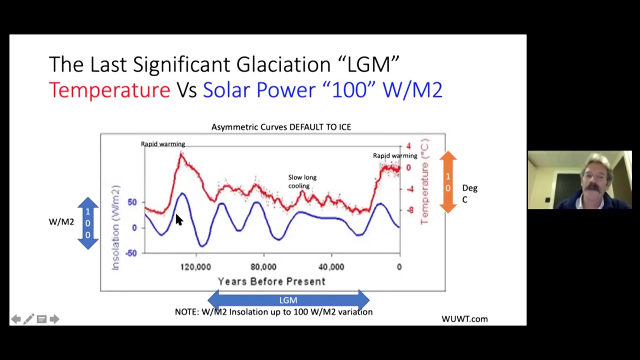 So the 100 watts per square meter that I've referred to is here shown in the southern hemisphere as a radiant solar energy difference between summer and winter. This is their winter and this is their summer- Summer over here. So what we're dealing with there is exactly what can happen here. So once again, here's that: 100 watts per square meter. 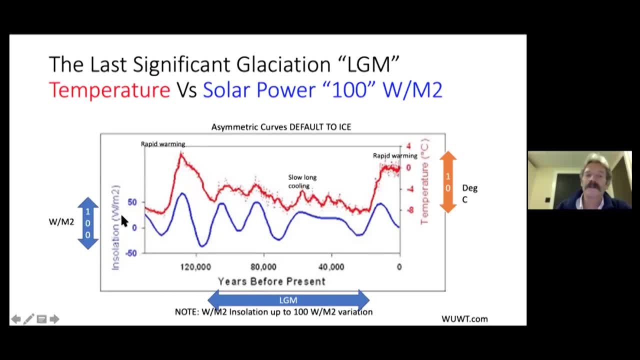 This is the incident: solar radiation in watts per square meter between 50 and 50. And this is what we see at 65 degrees north latitude. This would be the insulation. So we're getting that much variation As we move into this rapid warming. this is the combined curve of all of the contributing factors of the Milankovitch cycle combining to create a single curve. 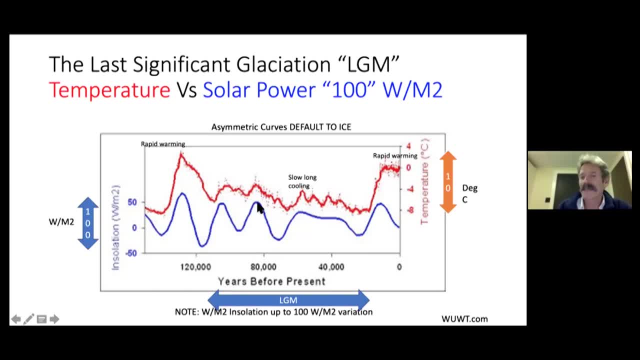 So this curve doesn't quite make it. You see how it does try to respond here and here and here and then falls off and then comes back and actually makes a big difference in another warming. here It's the coincidence of those curves That makes all the difference where, 100,000 years into it and we're 6000 years out of it, there's a big degrees centigrade move here between the top and the bottom of 1010 degrees centigrade. 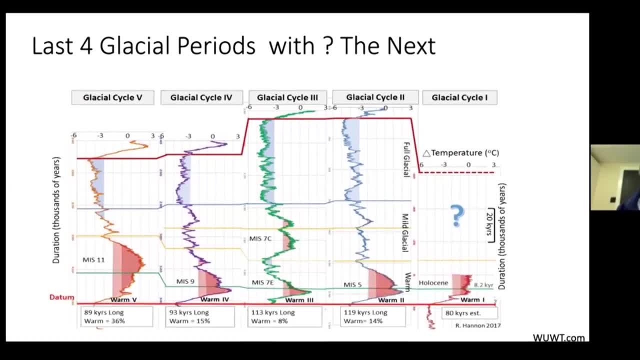 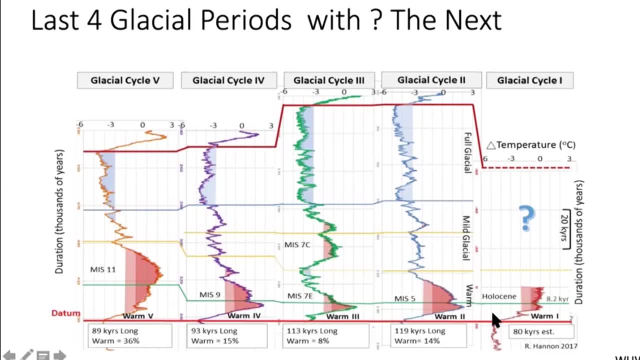 If we were to take all of the ice cycles that we talked about earlier, or some of them, we had nine before we go up to number five here, counting the one we're getting into here as the beginning of number one. That one Is: this is the last glacial maximum here. 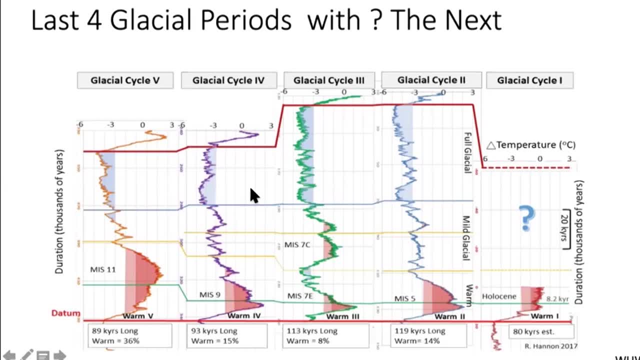 If you look and try to glance between these curves, you see lots of things that are correlative. you could correlate this event between these various areas stretched out over, this case, 500,000 years. That means that there's something else tying them all together. that's something is the sun, in the solar efforts that it makes. 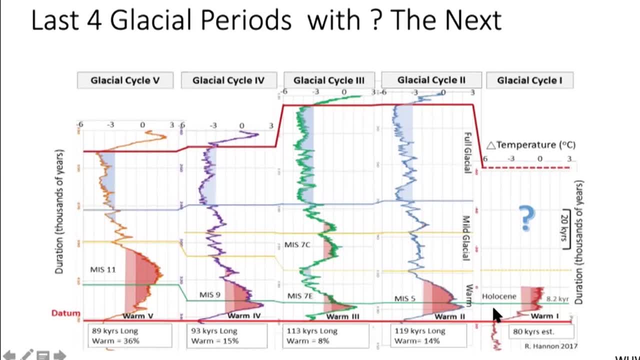 Are we Or are we not in a warming period that is going to last very long? Another thing which this one counts to: to look at 36% of this, it looks like it was in the warming period 15, 814, and we don't know here. 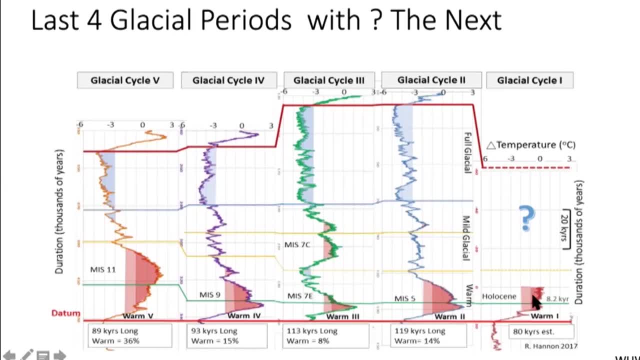 According to Mr Hannon here, This may go on. It may terminate it, it may have a great duration before we plunge off the other side. This is the termination. I have to call this one the inception of another glaciation. So where are we now? 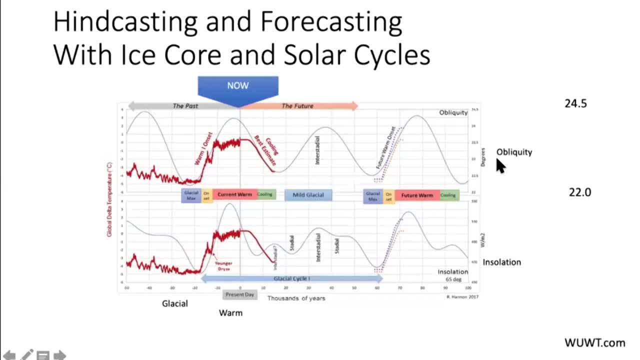 This is where we sit, on the obliquity. remember that was the tilt of the earth- and the insulation, the total insulation, at 65 degrees north. This is the future And this is the past. We are living on this little plateau here. 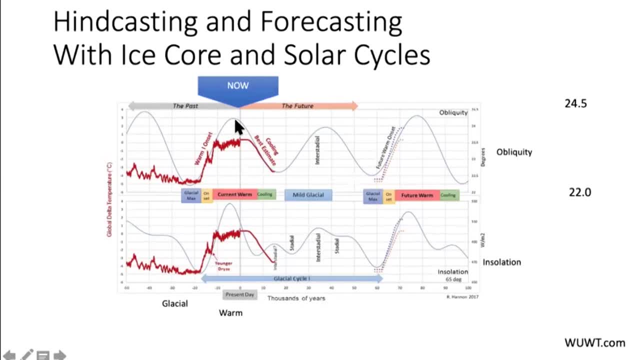 Past, the peak, it would appear, of the obliquity. This is the future And this is the past. This is the future And this is the past. Now moving down into the city cycle. Now moving down into the city cycle. 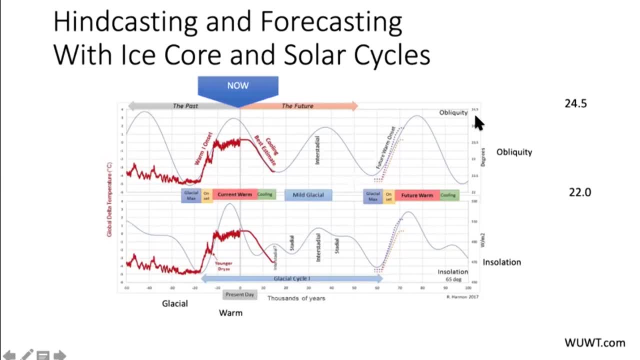 Moving now down into a different one. Now, that means we've moved past 24 degrees of tilt, going back to, we're Going back to. we're 22 degrees And we're at 21. And we're at 21. Now. 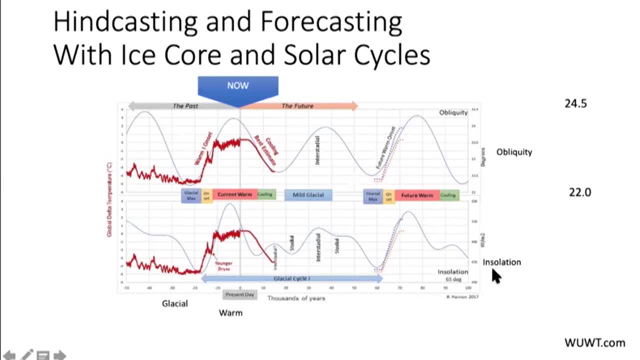 So what we're dealing? 21 and a half. So the other portion here is the insulation. that'd be the combined total. Now that means we've moved past 24 degrees of tilt, going back toward 22 degrees, Going back toward 22 degrees. 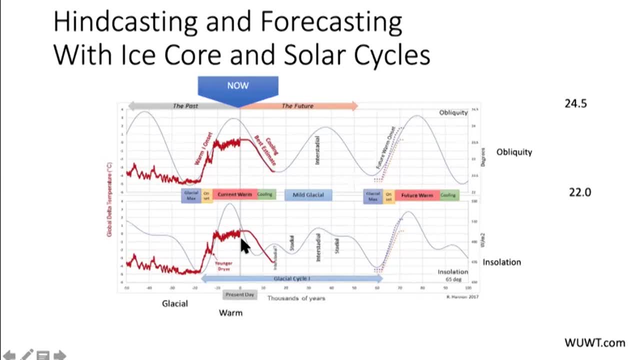 And we're at 21 now. Yeah, we're almost at the point where that's dropped to a stage where it's going to be pretty critical. What about this one here? We're going to have to get into thinking about that. that might try to extend it a little bit longer. 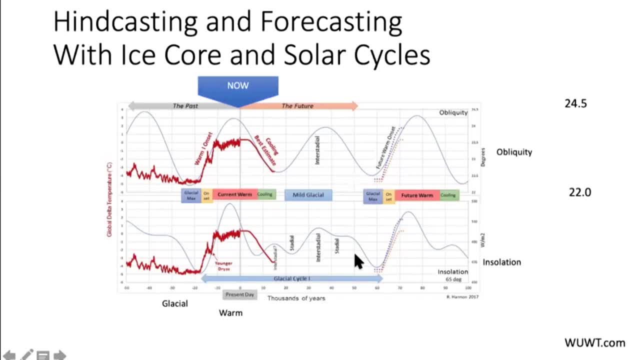 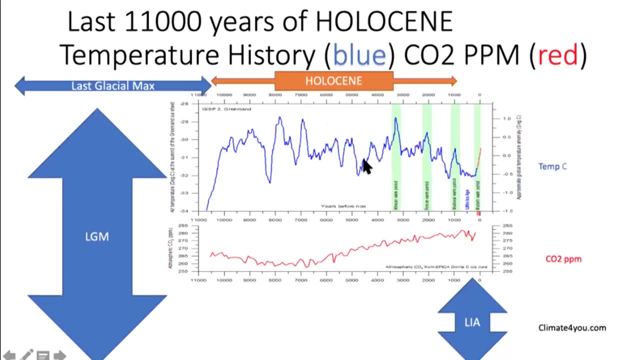 So we're not sure where we are in time. It's not a perfect extrapolation, but it does give you a little bit better feeling that we may be into the warmth for a little longer before we hit the cold. Now, that little island that I was talking about, that we live on now, was warmer at one time up in here. 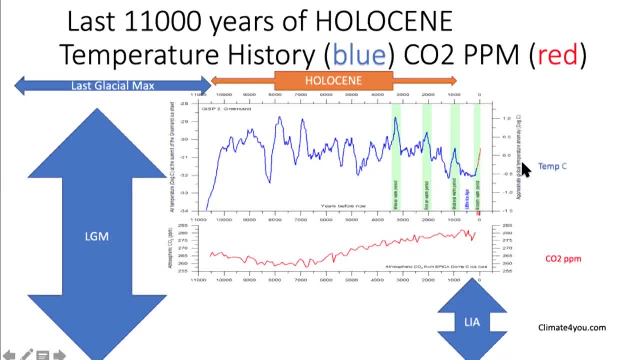 This is the temperature curve in blue. So what we have now done is we have fallen off of that temperature high toward the little ice age period which we just came out of. What are these other green things here? Well, those are pieces of the Holocene that man was civilized during. 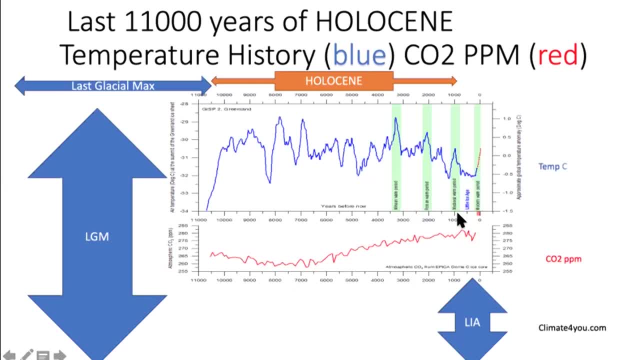 The Minoan period, the Roman period, the medieval period and the modern period. What was happening with CO2 through that period of time? before the modern period, CO2 was acting inverse to temperature. During the early part of the Holocene, the temperature was high. 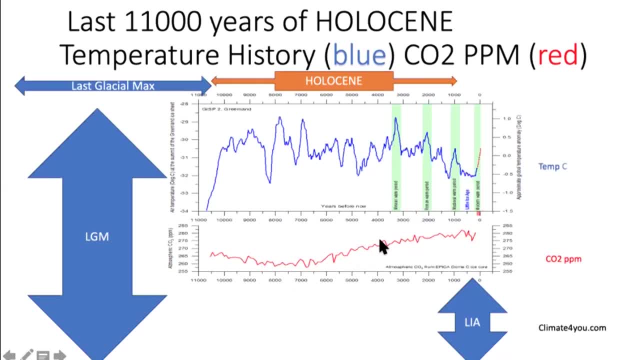 The CO2 was lower. It then eventually started moving, And then it collapsed fairly strongly into the little ice age as well. So juries out a little bit in the really near-term fine tuning On the bigger scale. once again, we see it all over again. 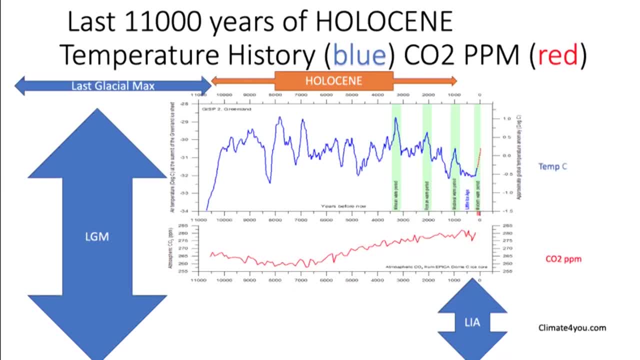 The same asynchrony between the CO2 and what we need to do is to think about breaking this down and looking at it in much more detail. The little ice age, The last glacial maximum CO2 temperature- Those are the players that we've chosen to work with right here. 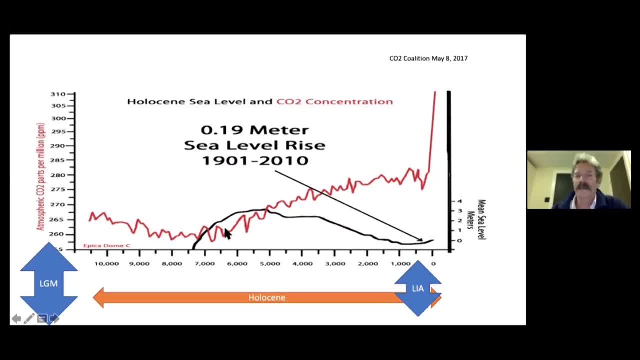 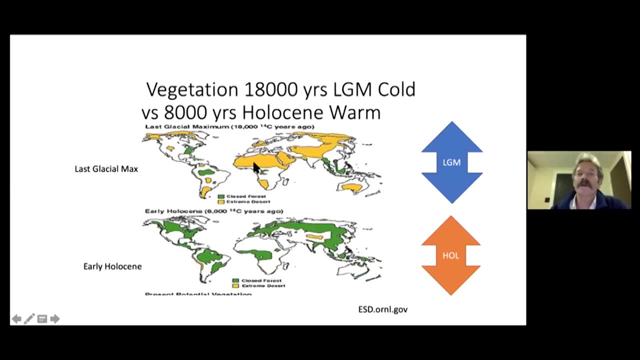 This one brings in the sea level curve as well, showing that CO2 is responding differently than even the sea level issues that we were dealing with here. What did it look like when we were in the depth of a glaciation? We just were at the breakout point now of the last glacial maximum. 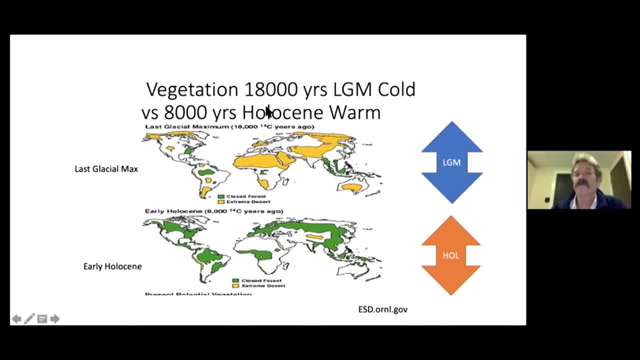 We just were at the breakout point now of the last glacial maximum, Of the last glacial maximum 18,000 years ago. So deserts, as I mentioned to you, very large, continuous desert systems on the top of the world. 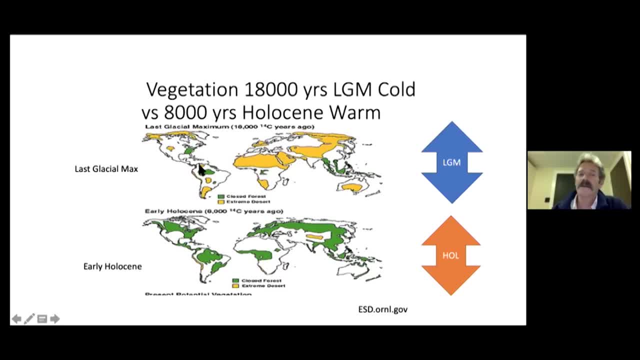 And also close to the south pole portions, Small and hanging on. in the equatorial areas we have forested areas. Now we move into that beautiful warm period at the beginning of the Holocene where we were at a temperature higher than we are today. 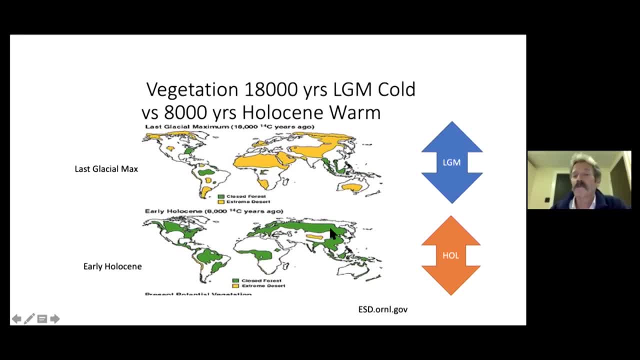 Where we were at a temperature higher than we are today day. This is the green area that represents the forested components of what was around at that time. Desert was restricted, although it should be shown in this area of extreme desert. So what? 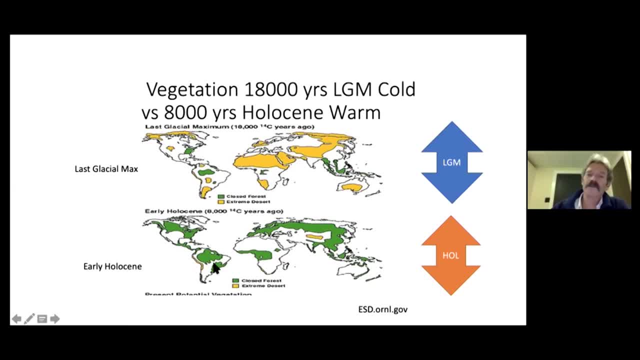 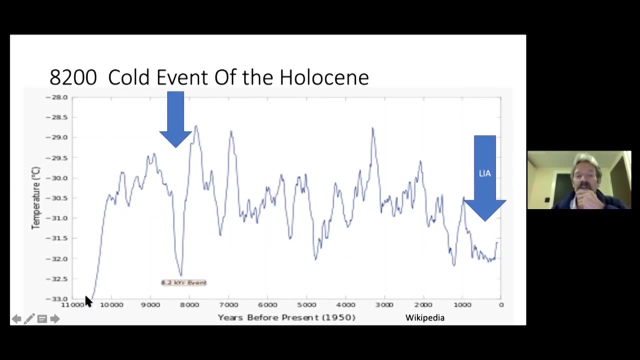 we have is a radical difference that we want to appreciate in terms of relative importance of temperature to our existence. We have here a piece of that Holocene as well. between 11,000 years here and the current time here, Little Ice Age is this dip. We'll talk about it in quite a 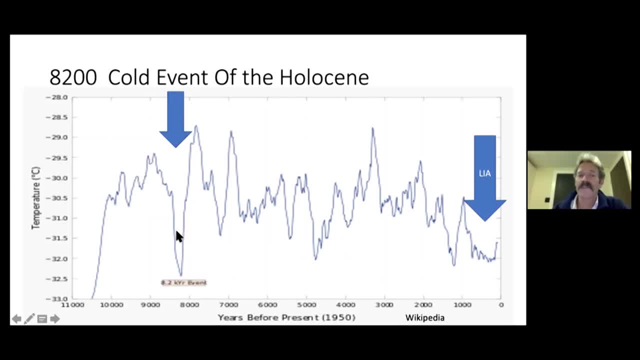 bit of detail. I haven't the time, unfortunately, to deal with this one as much as I'd like to, but we'll do a little bit of justice to it. This was a dip even lower than where we were in the Little Ice Age. 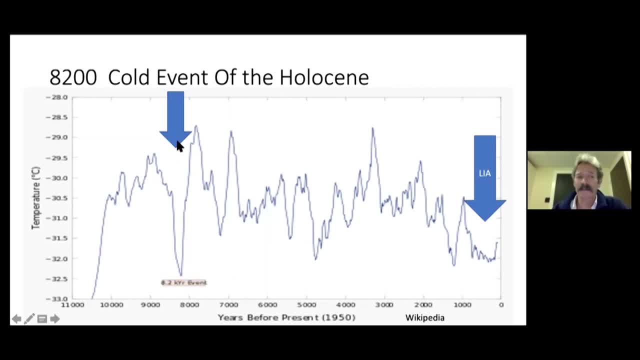 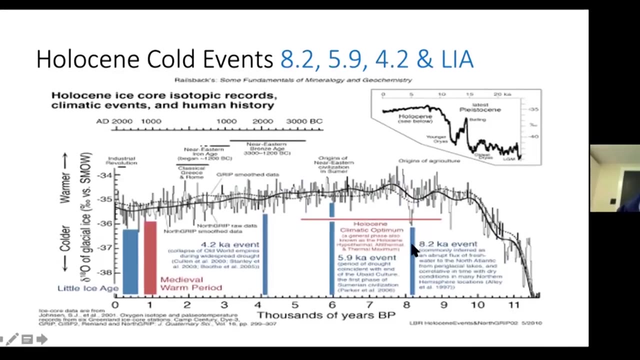 This dip is likely related to the oceans. as a giveaway, Some of these other ones will be dealt with, or we will try to deal with them in that second lecture. This is the Holocene. I'm reversing the scales on you here and I'm sorry about that. 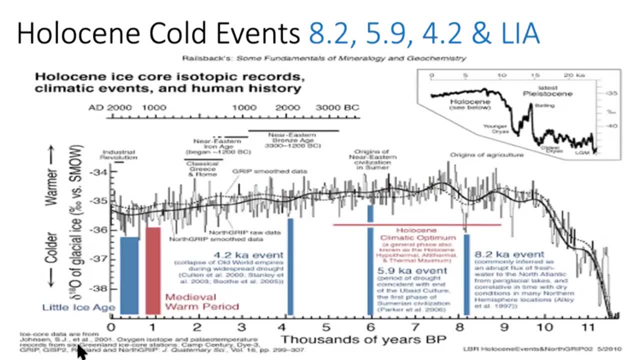 The representations seem to always bop around between zero on this axis or zero on that axis. We have a little dip here. This is the Holocene. This is the Holocene. This is the Holocene. We have zero over here this time. This is the current day. industrial revolution, as it calls it. 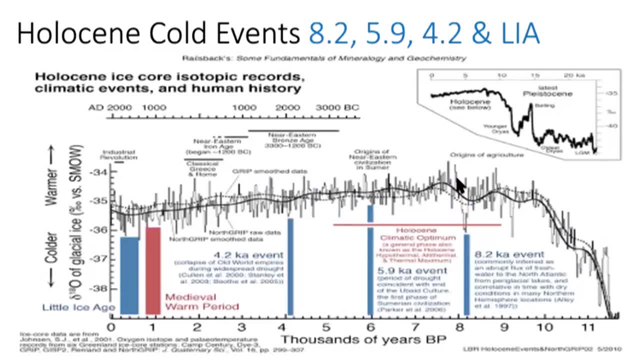 here The classical, Greek-Roman period, on back through history. You see how much higher we were in the past and the origins of any agriculture would have been back in this period of time. This is the Holocene climatic optimum, as it's called. These are those cold events. This is the 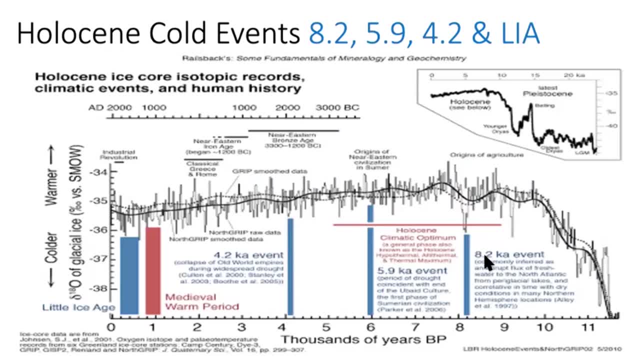 8.2 ka. That'd be thousands of years. This is the 9.5,, the 4.2, and then the Little Ice Age. Each one of these is registered within the rock record, within the ice record. We need to also recognize that we have just emerged from. 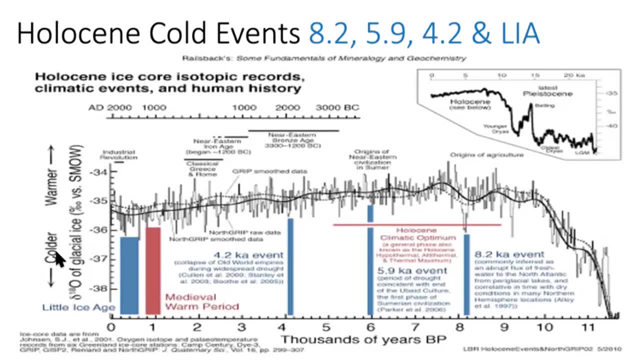 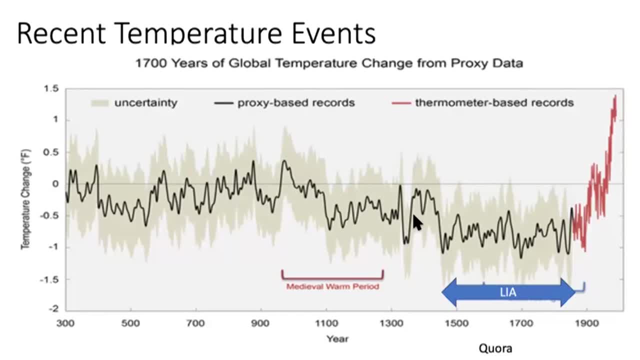 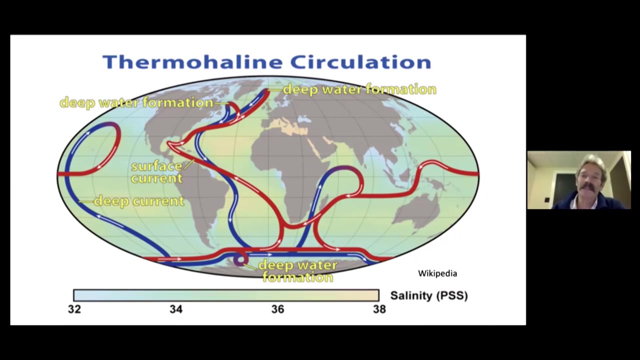 rest of the story, The Little Ice Age and the variation in the uncertainty of that reading is shown around a medium. here We're not showing that uncertainty back out into the thermometer-based readings on this side. What's gone on when we truncated that wonderful conveyor belt of heat? 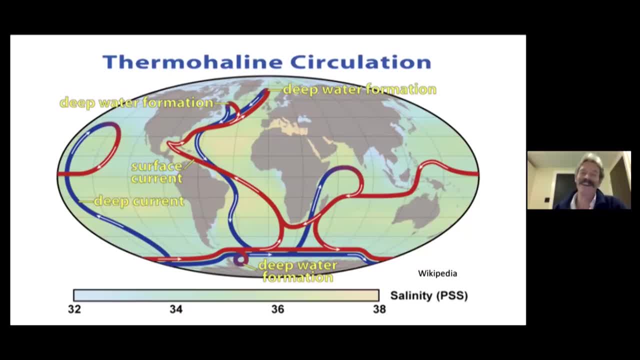 that was going around the equatorial area. We couldn't get it to the poles. What happened to it? It degraded into this. This is the thermohaline circulation pattern of the deep ocean. This would have been the Gulf Stream coming north here, dumping its water and 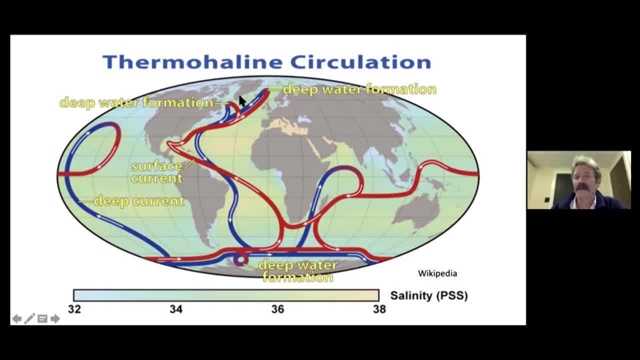 melting what's going on in the north here, bringing it down as a more dense current into the deep ocean, Running it all the way down to the southern ocean, where some of it upwells and some of it circles around and blasts out into the Pacific. That's the circulation pattern that we're on now, Not very. 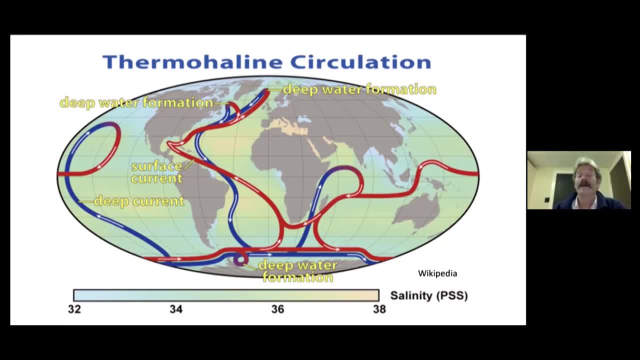 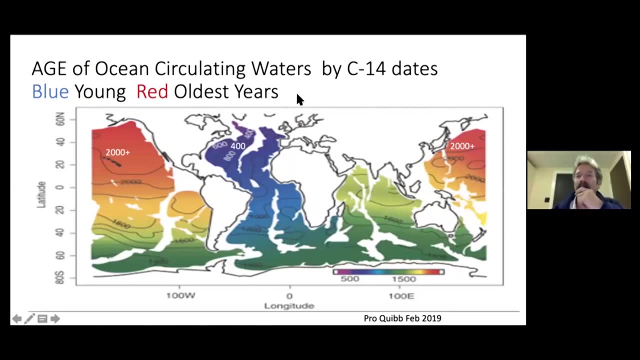 optimum to go ahead and deal with our issues of understanding why temperature changes and climate changes are so important. We can look at it on an aged basis by carbon-14 dating, a dating method which has a half-life of about 6,000 years or a little bit less. We can look for 2,000 years here, 400 years here. 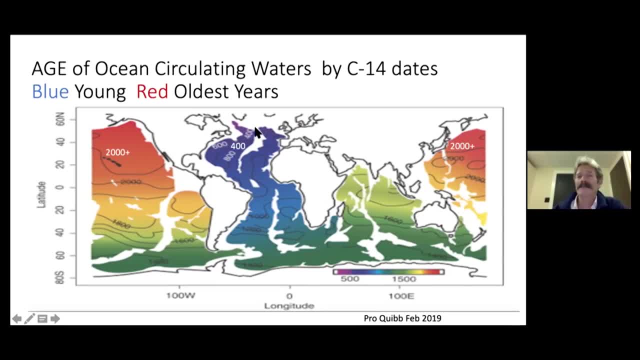 This is the North Atlantic. This is where the water begins its life and starts to collect again the carbon from the atmosphere at cold temperatures. This is the North Atlantic. This is where the water begins its life and starts to collect again the carbon from the atmosphere at cold temperatures. 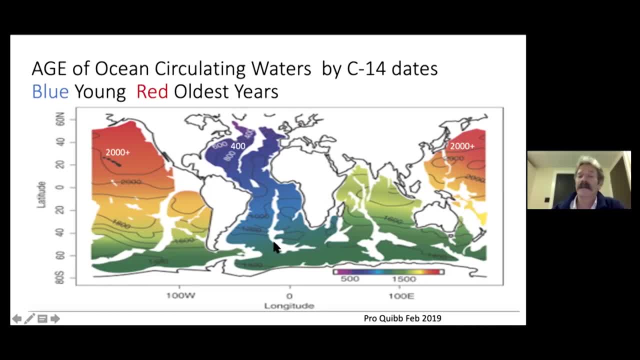 This is where the water begins its life and starts to collect again the carbon from the atmosphere at cold temperatures. It moves down, moves around the Antarctic in its major current system here, stays in that current system and also helps promote a lot of life within that system. Then it eventually moves into the 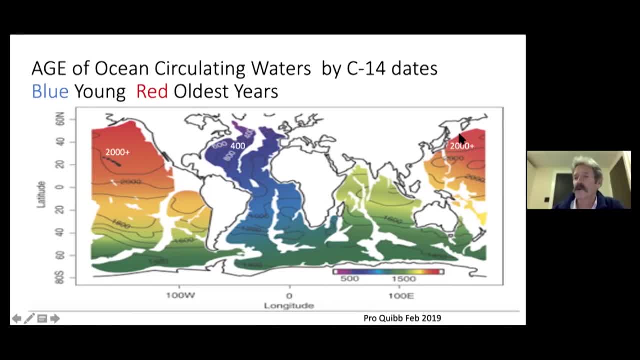 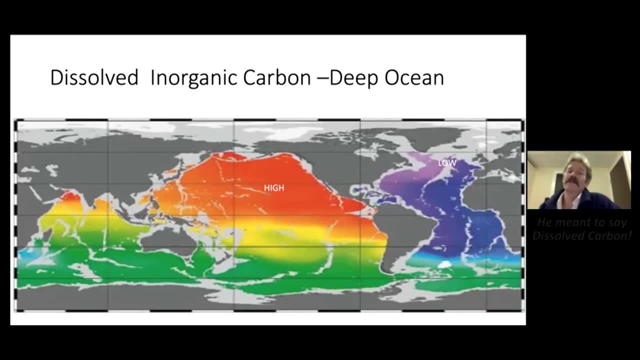 extreme northern portion, in the northwestern portion of the Pacific, here, where it is the oldest water that we know. This is what happens with this dissolved oxygen, in that sense as well, The high is in the Pacific, The low is in the Atlantic. So these are the deep waters and their dissolved 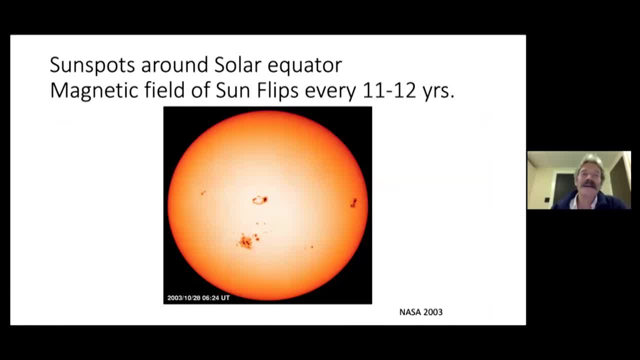 oxygen, inorganic oxygen that's in it Sunspots. around the solar equator There's a magnetic field that flips on the sun every 10,, 11, 12 years. These are the sunspots as we see them on the surface of the sun in our NASA shot. 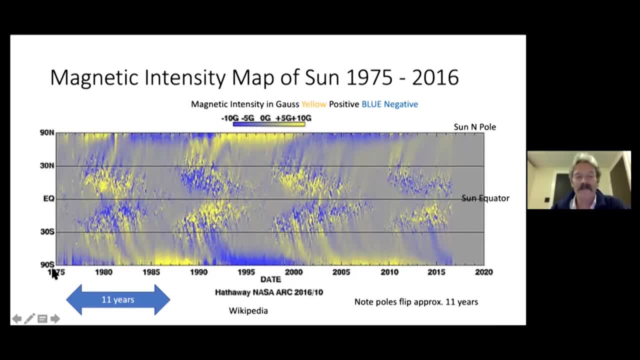 This is stretching it out. We're taking it over time, from 1975 here, when observations of this sort began, right through 2020.. We're looking for the sun equator to be here on this stretched out version through time. So once again, we're taking 3D space and making it into 4D space. 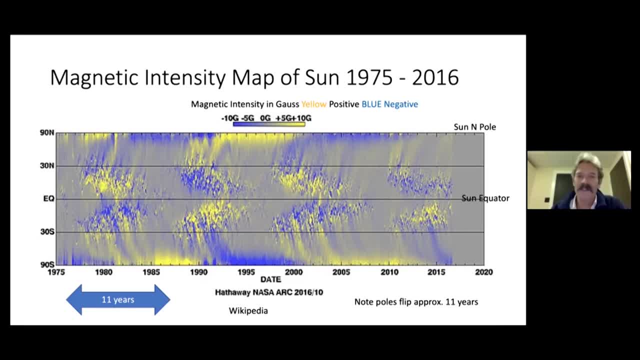 on a representation that shows polarity of the sun in colors: Blue negative, yellow positive. 11D year cycles, migration of the sunspots through time toward the equator, north and south, coming on like this- the arrows of sunspots, we'd have to call them, and then polarity flipping to yellow. 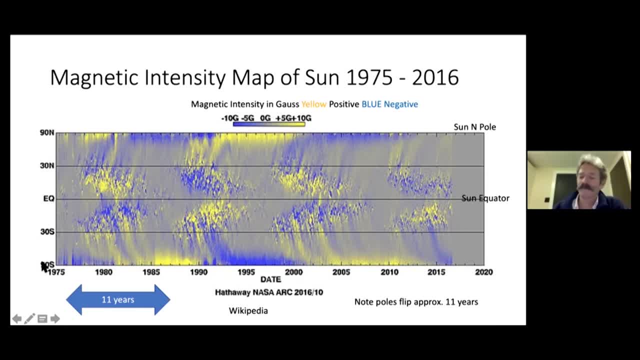 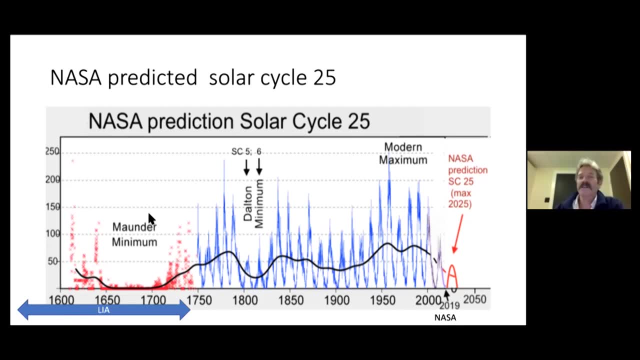 from blue every 11 years. that's a lot of variation. what does it do to us on earth mass's prediction of where solar cycle 25 will be? and we've been counting these for quite a long time, as you can see, this was five and six. um, this is when we were just looking at sunspots back in. 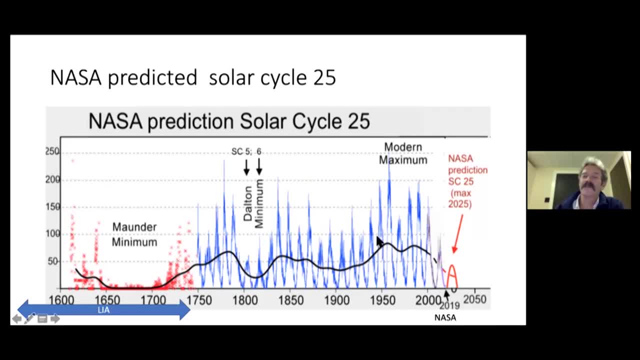 here, so it doesn't have the fidelity of this series of curves which show extreme numbers of sunspots in some of these peaks, talking about 250 um and down to 50, and then down to zero. oh, what's this period of time? well, the little ice age. guess what? this is where we're. 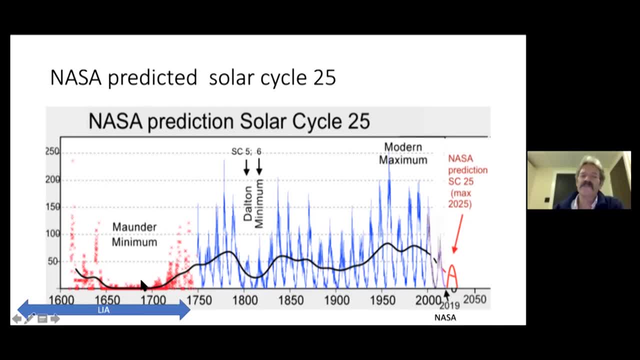 building our models. coming out of this was a solar um hole. this is the motor minimum named after the fellow who saw it first. dalton got his name on this one um, the modern maximum. we haven't really got a person's name associated with, but we're coming off of that to a degree right now. 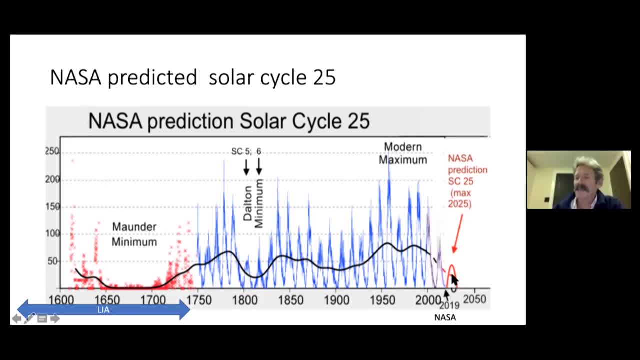 so we'll see what happens next. so we'll see what happens next. so we'll see what happens next. will these cycles continue to fall? will we mimic what happened in the dalton minimum or will we do something that hadn't happened in the motor minimum? would we have the potential just from? 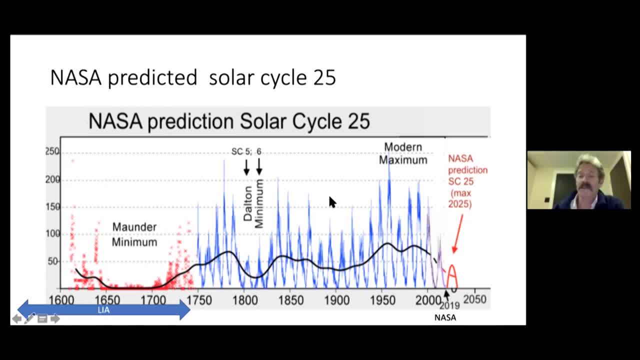 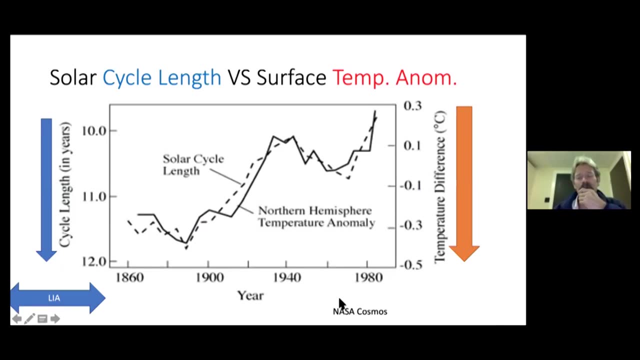 the solar cycle? um changes, uh of energy. would we put ourselves into a position of having another little ice age? if you look at that solar cycle length, this is the solar cycle length was anany way. we use similar planes as an older paper is in this picture- an older paper. my apologies from nasa. though they were able to correlate. 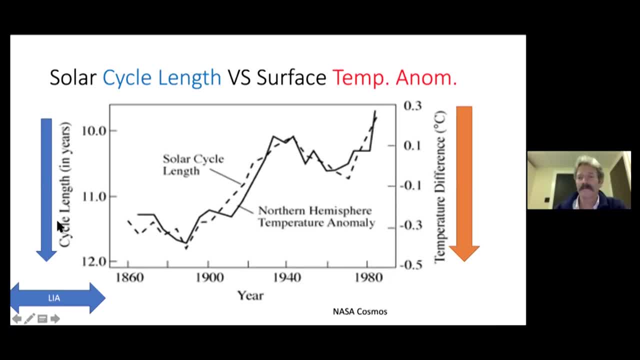 um the temperature inverted to the solar cycle length. so what uh we're we're dealing with here is a, um, a coincidence perhaps, between 1860 and 1980, but nasa was fairly convinced at that time that that was a major determinant of what was happening to um on the ocean. um, so, uh, the temperature. 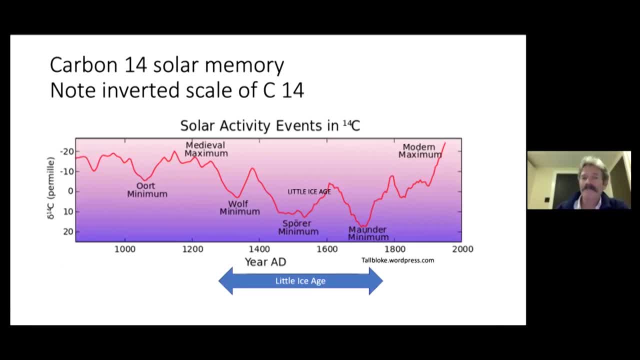 our climate temperature. These are some of the ways in which we can move back in time using that carbon-14 to see the changes in the sun's activity level. So there are many other names here. I won't go into all of them. 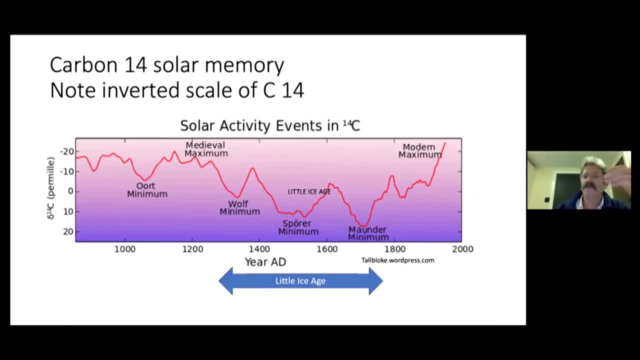 but each one of those can be parsed out and compared to a lot of other proxy information that exists within our inventory, within the ice, within the rocks as well, And this is the direction which we have to move in really finding out where we have come from. 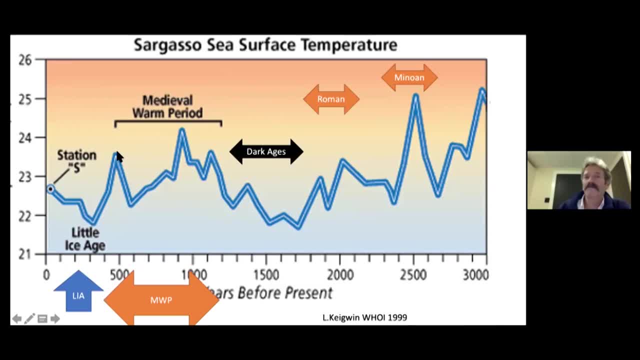 to know where we're going to In this one. a chord out in the middle of the Sargasso Sea was looking at the sea surface temperatures by material that had dropped to the bottom once again. So here they were at that time, just after the little ice age. 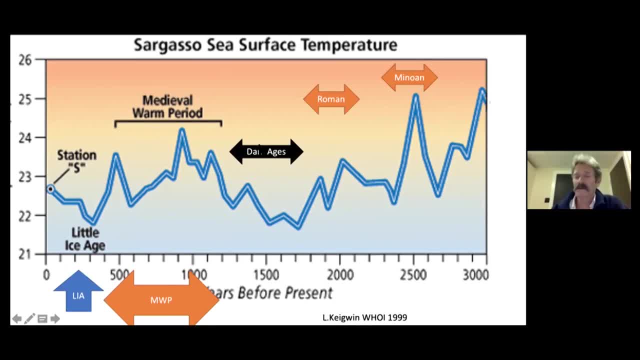 they looked at the medieval warm period. They saw the dark ages, another period of time which we haven't mentioned much. They saw the Roman and the Minoan warm periods within this ice core from Hui, which is back out on the east coast. 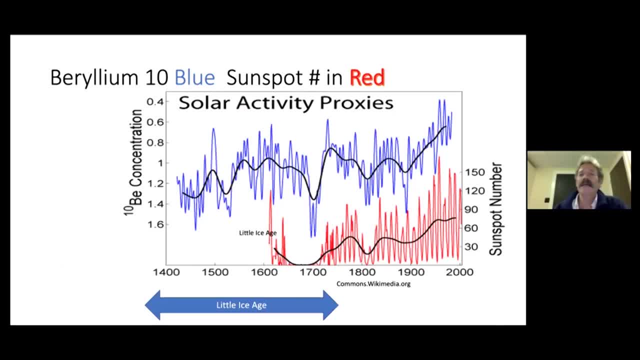 And this is Woods Hole. Beryllium is another substance we can use. It's a radioisotope from bombardment of oxygen and nitrogen in the upper atmosphere by cosmic radiation And that can be used as a proxy of solar activity, and we'd have to explain that in more detail in a later talk. 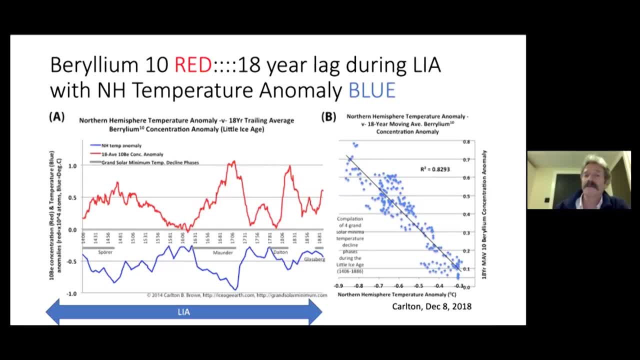 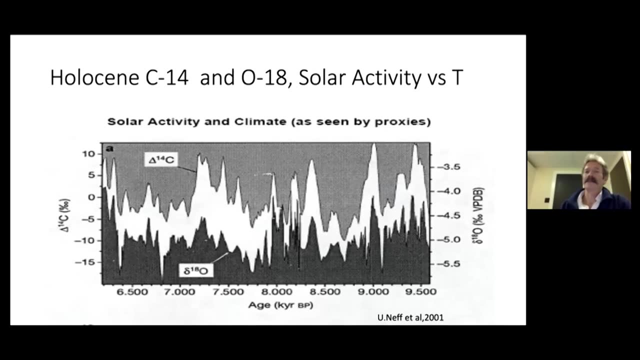 That has a bit of a delay to it- an 18 year lag to it- but it's very coincident, as you can see from some of this corresponding work here. So it's going to be a valuable tool. When we look at just the carbon-14 over parts of that. 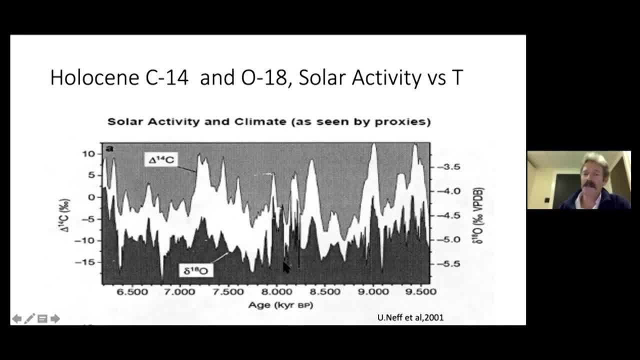 as the proxy. what we're looking at is the temperature proxy here. carbon is not involved here. It is here. This is the oxygen isotope, the carbon isotope. The carbon isotope and the oxygen isotope are showing a coincidence. 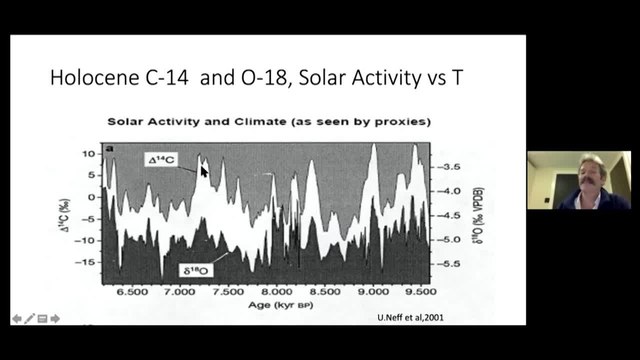 This being the carbon-14, showing us the activity of the sun, not the carbon dioxide, to make this very clear. So what we're dealing with is using this proxy to support this one and to perhaps find other things that are going on Within the system. 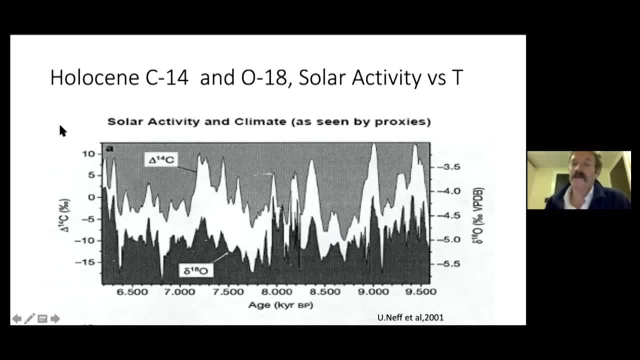 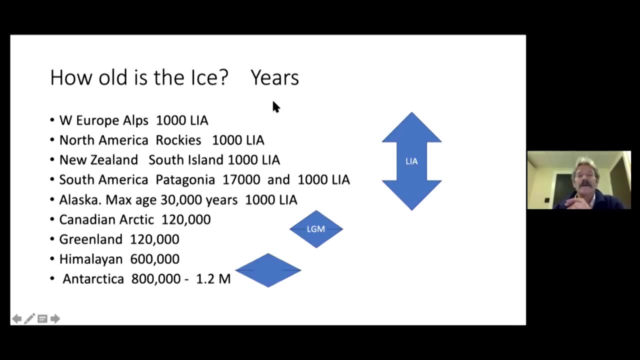 So there are other isotopes that we can use to corroborate what happened through the Holocene earlier than when we've really started to intensely take it apart. This is one which we have preserved in the geologic record of ice. These are the ice fields of the world. 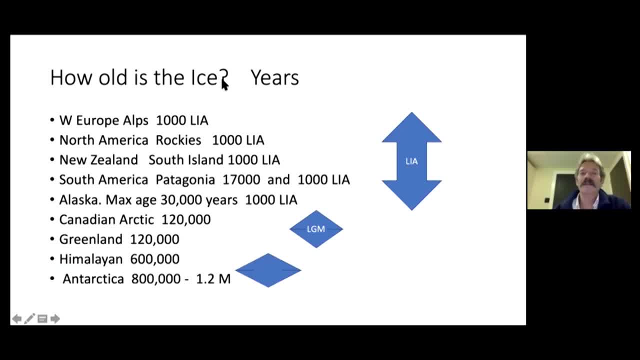 that are very familiar to you, hopefully, We're dealing with. how old is that ice? It's not very old. That's the the final answer on this particular slide. The Little Ice Age is this symbol here and this one here. What we're dealing with in the Alps is Little Ice Age ice. 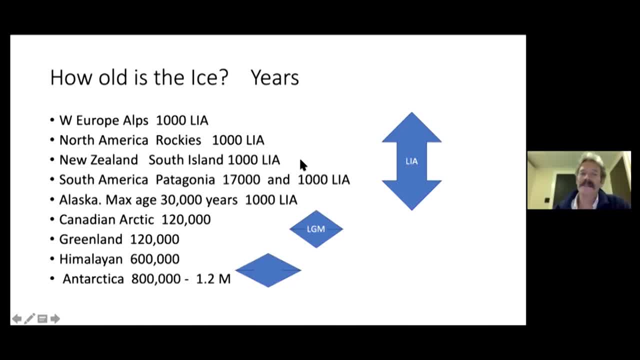 What we're dealing with in the Rockies the same, New Zealand the same South America and Patagonia: the same. They have a little bit older ice. there They were able to find 17,000-year-old ice, but that doesn't really make it too much. 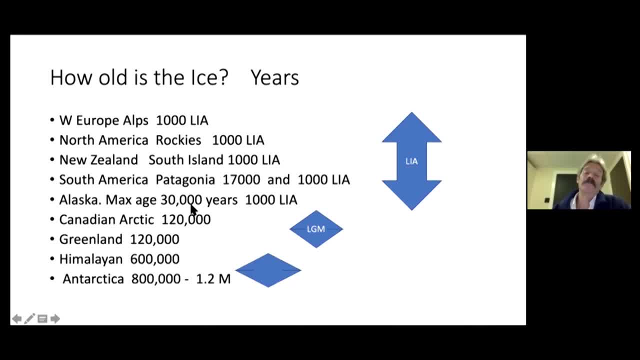 So we're dealing with a little bit older ice. there. They were able to find 17,000-year-old ice, but that doesn't really make it too much. But in Alaska, a place that a lot of people go to see, ice melt now on cruise lines. 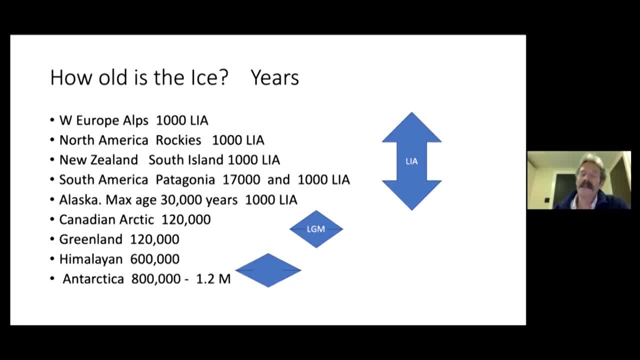 30,000 years is the oldest ice that's been able to be found in Alaska. Most of it, most of everything that's being seen and viewed, has been created during the Little Ice Age, not before. This is very recent ice. What about the Canadian Arctic? 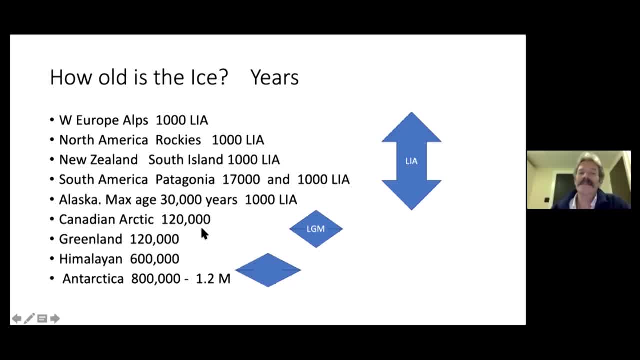 A little older for sure, more like Greenland. This is the last glacial maximum. That's all we got there. We don't have anything else. That means it melted off before. Greenland has been ice-free 120,000 years ago or slightly longer. 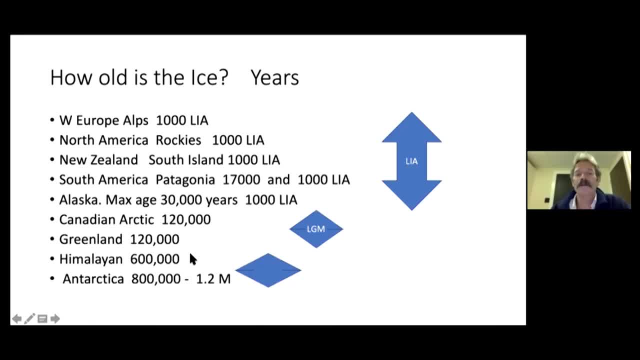 The Himalayas. a much bigger polar ice cap has been in existence 60,000 years that the oldest ice has been found- Antarctica, the oldest of all, up to 1.2 million. Some of the ice core is really only 800,000 years back. 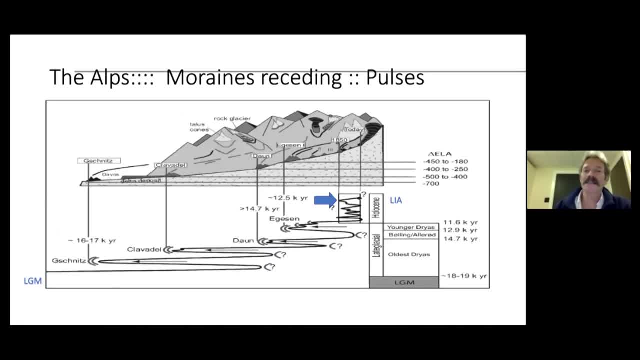 So that's a very long time. That's a very meaningful issue. moving into the next slide, The Alps. how do we know this? The glacial morainal deposits of the rock that are deposited within the area of the Davos, Swiss Alps. 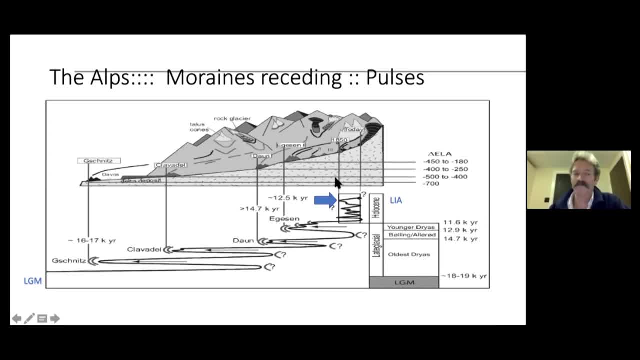 show this recessional stepping through time. The time is shown over here of where they belonged. We are looking with the blue arrow now at the little glacial, the little ice age. So the little glacial ice age is melting out today. moving back with this particular line, 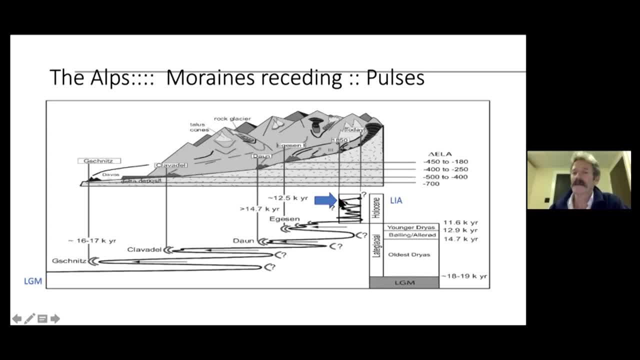 And was it a maximum here in time? There were, as you see here, a lot of other similar mapped occurrences within the Swiss Alps, So this isn't the last one. You remember we had all those other coolings. They have to be mapped out, understood and correlated with the ice. 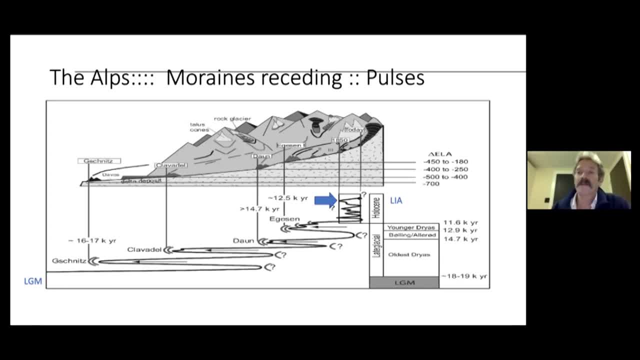 They have to be mapped out, understood and correlated with the ice. They have to be mapped out, understood and correlated with the ice And with this information to properly understand what the Holocene is made out of and how climate varied there. 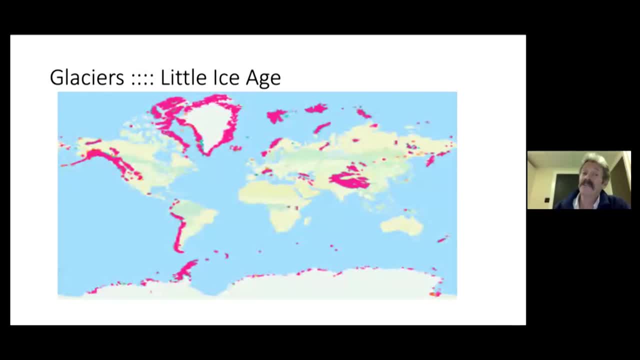 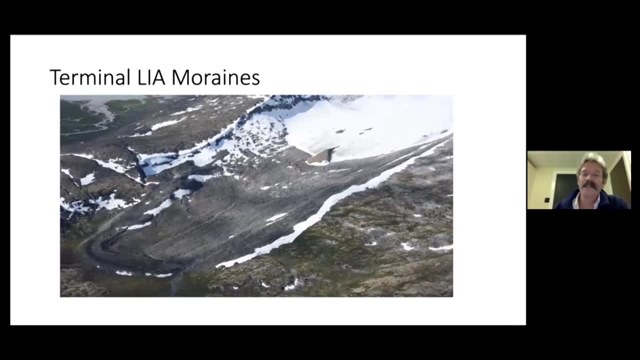 These are the areas where glacial ice is melting now and just formed during the little ice age That's not long ago. This is what a terminal moraine looks like, just for ground truthing. This is the tongue of rock. ground up rock. 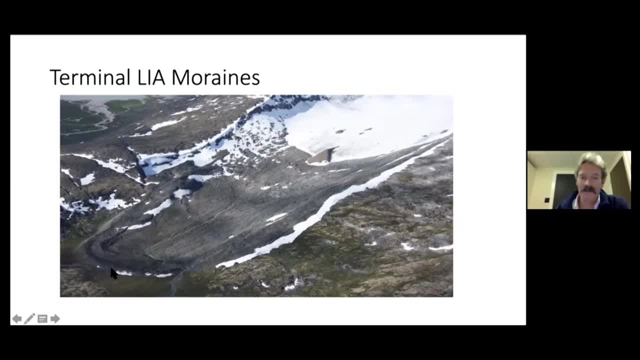 that was brought down to this point during the little ice age advance, Maybe, you know, in the 1600s, 1700s, toward the 1800s, And then it actually started to recede And it moved back to here, and moved back to here, and moved back to here. 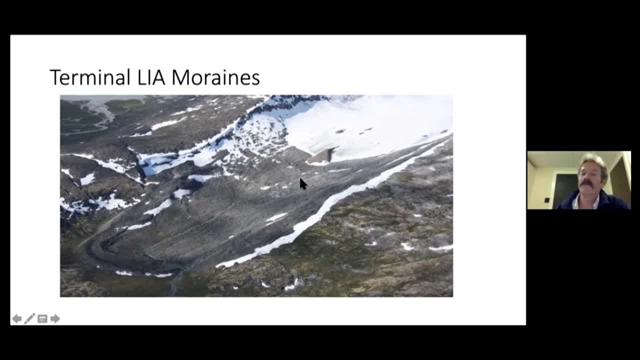 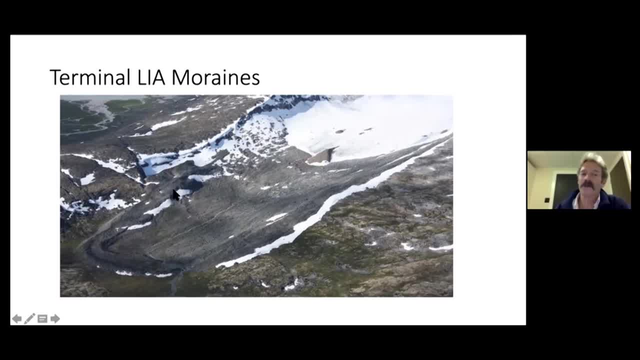 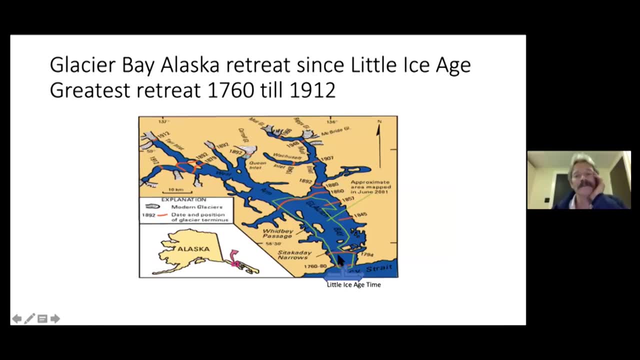 But the last one is this one: here that we see the little ice age morainal deposit, Alaska. We're going to go to Alaska in a cruiser. We're going to go into Glacier Bay. We're down here in the Panhandle area, as you probably know. 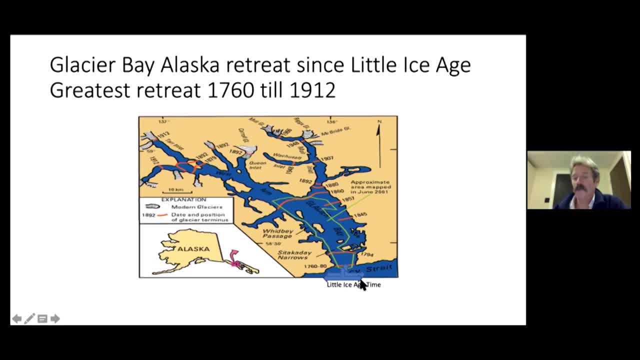 This is Icy Bay out here. Icy Bay at some point in the little ice age was completely chock-a-block full of ice. It was iced over. Couldn't have made that trip at that point. These are the lines by geological examination and carbon-14 dating. 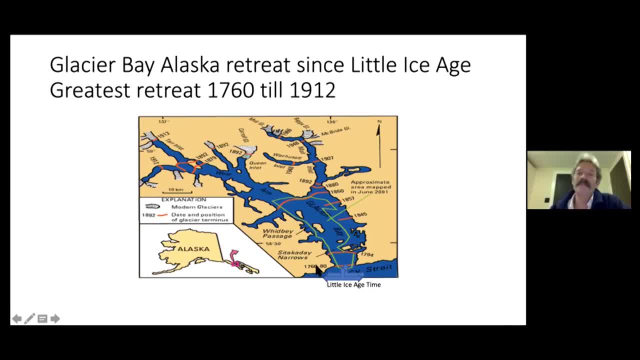 between 1760 and the top of the system, 1966, here even 1912, back in this particular arm, the west arm. This is the one which is a little bit more recent, But, as you will appreciate what's really interesting. 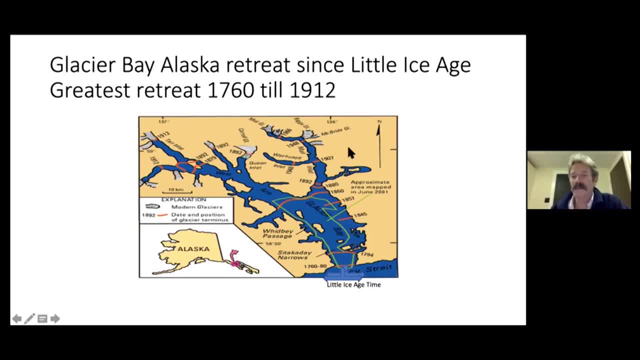 what's really happening here is we're seeing old retreat. The entire area was full of ice. It is all retreated. And when did it retreat? Oh, that's really interesting, isn't it? Oh, and how far did it retreat? 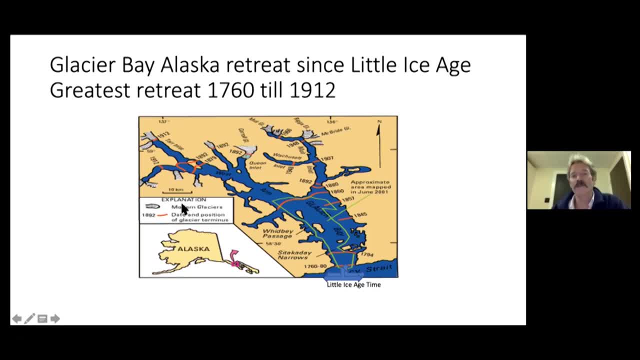 These are kilometers. 10 kilometer increments or bytes are shown by this symbol, here And when, All in this period of time- Really almost all pre-industrial, isn't it? What was going on before the industrial era that could have started to influence the early meltback? 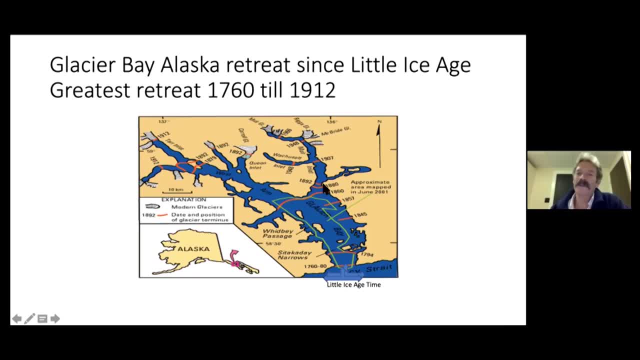 When I talk about early meltback, we're talking about the industrial era. back in here And on this arm I'm talking about it gosh, yeah, back up in I don't know about, in here someplace anyway. 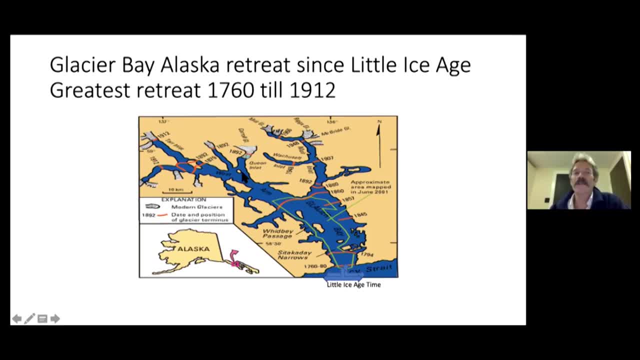 Hasn't actually got it broken out perfectly there, But what we do have is evidence that retreat advanced before anything was going on. We were recording, We were recovering from the Little Ice Age, which was, as you remember, the motor minimum. 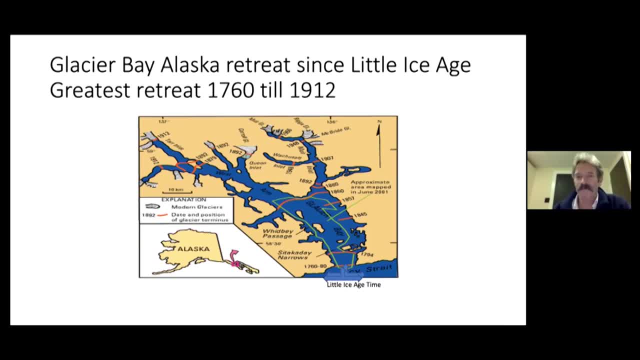 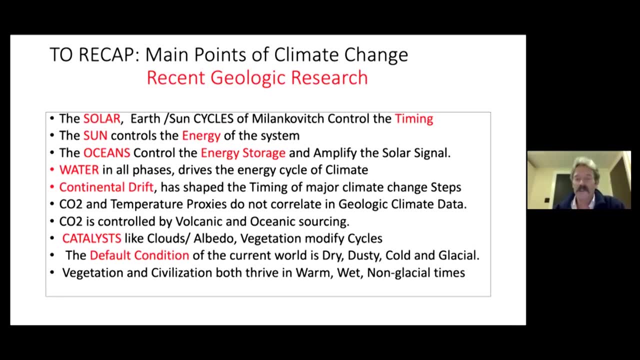 the depths of a solar minimum. So that's pretty well the end of this talk for the first round, but there's a second round coming and hopefully you can come to that as well. So, to recap, the important points that are really important from the talk are all based on recent geologic research. 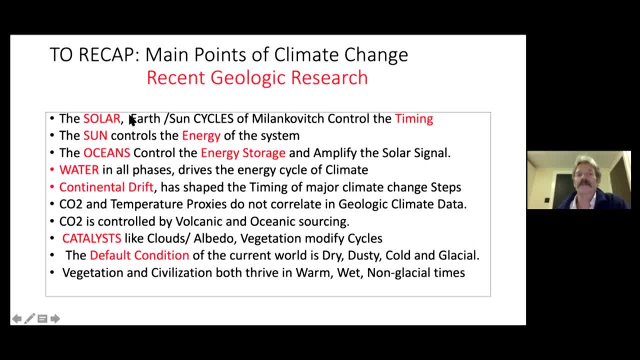 They relate to climate change. First of all, the solar component. the cycles, the Milankovitch cycles, govern the timing of everything. So we saw that and that is very obvious to almost everybody at this particular time. I don't think that there are many other differing views. 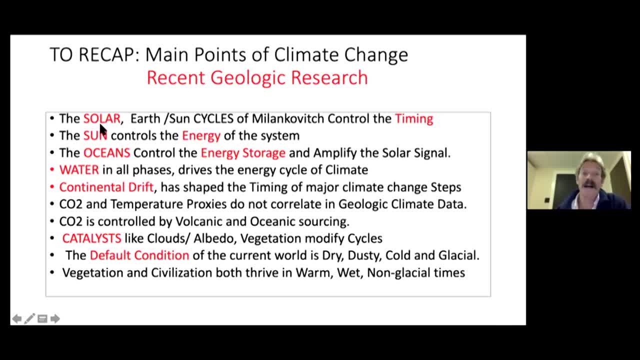 of exactly what controls the overall timing of Earth changing its climate and warming or warming. There are other controls which can be short term, such as volcanic eruptions, et cetera, but those aren't necessarily what we're referring to and they are short lived. 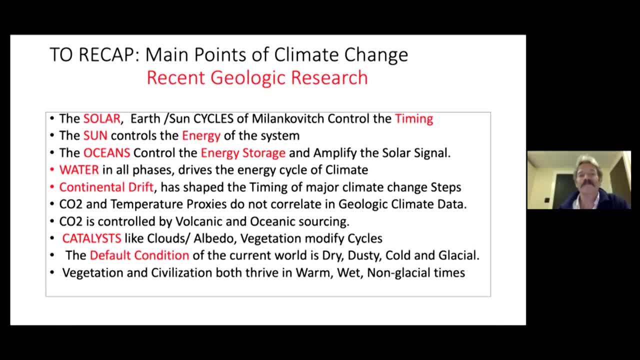 We're talking about longer term change. The sun: The sun controls the energy of the system. The oceans: The oceans have to be put into this in a much more meaningful way, because they have an energy storage component that can amplify any solar signal. 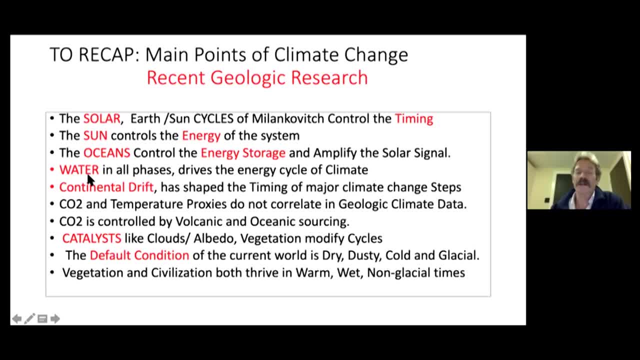 It can save it and keep it going through time effectively. It has a memory. So there's a solar memory in the ocean. The water in all of its phases drives the energy cycles of climate. Continental drift has to be implemented and understood in the stories that are being told. 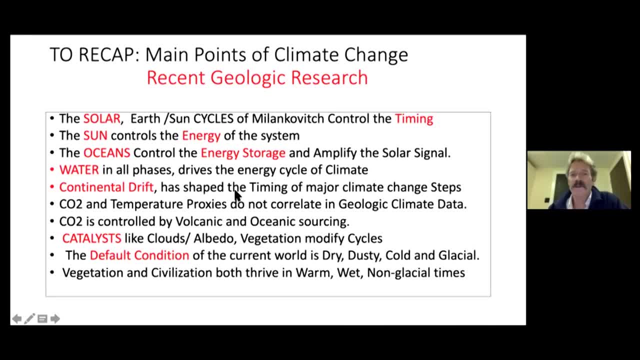 We are not looking at two end members of time properly. We're trying to say that the continents were the same at those different times. They were not. They were radically different and they radically changed the climate. We saw the steps. Do you remember the steps? 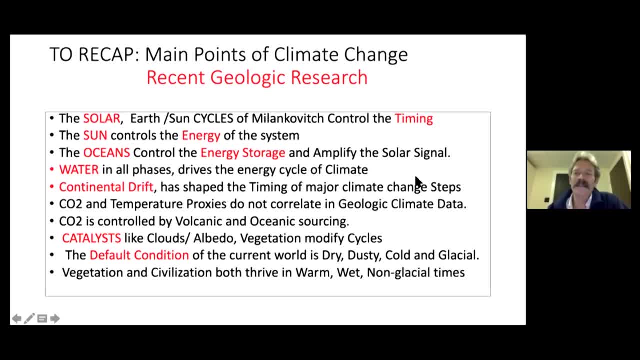 I should probably have made this red because that was a big deal. The movement of CO2 back and forth and back and forth without changing the temperature of the world. CO2 and temperature proxies do not correlate in geologic climate data of an advanced nature. 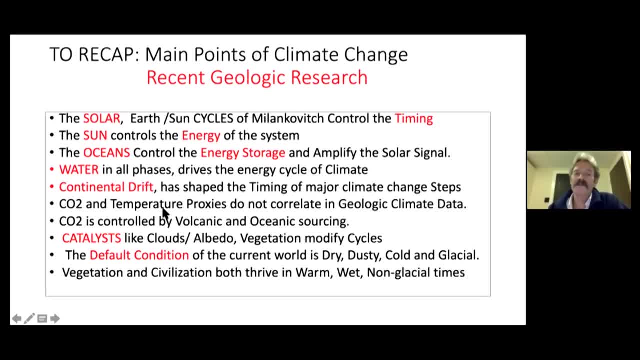 CO2 is controlled by volcanism and the ocean. Ocean sourcing of CO2 is what was driving CO2. in some of that early time The Eocene did have a high CO2 level. sometimes It did have a heating cycle which was really based on the ability. 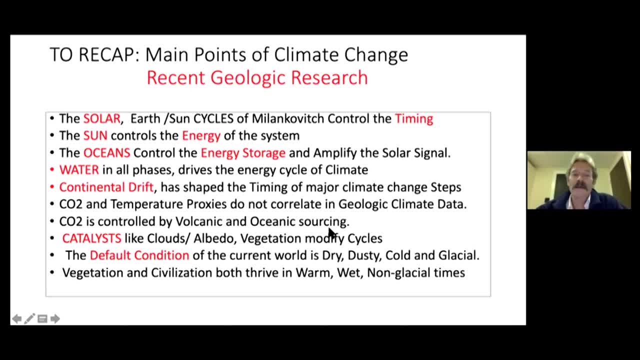 of the ocean to store energy. So there is a conflation of facts which needs to be broken down on a very precise and exacting basis. We have catalysts, the clouds, albedo, vegetation, that all can modify the cycles slightly. These are slight variations, of course, in what we see. 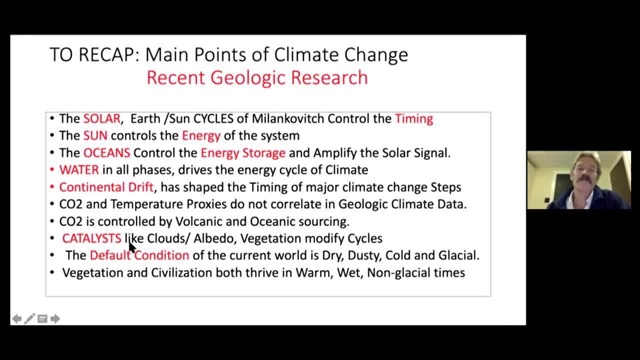 as the Holocene period as well. But many of these are ephemeral, as you'd expect. They aren't necessarily something except in their basics that are something to build into everything, but to understand in the short term It's a little bit like the difference between weather forecasting.